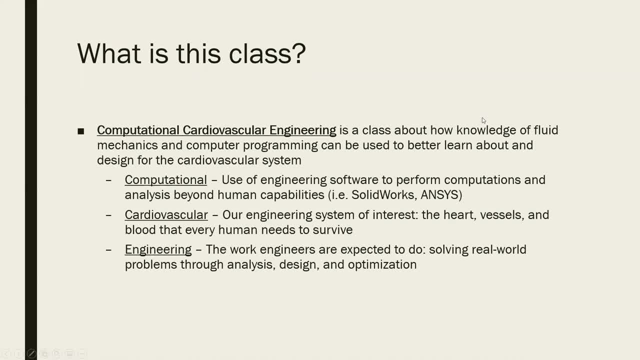 Engineering right, And so kind of. in a nutshell, what I like to describe this class is: it's a class about how we can use our knowledge of fluid mechanics and computer programming to better learn about and design for the cardiovascular system. okay, And so let's break down each word in the 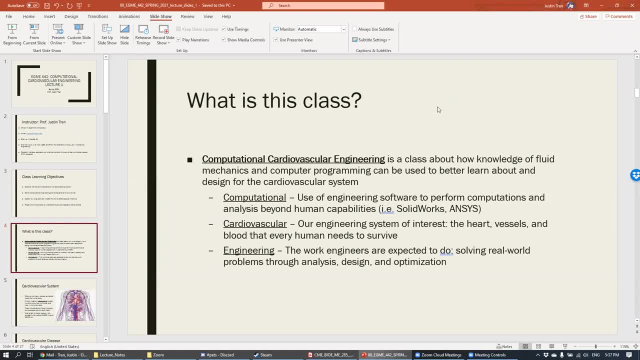 title. okay, And so first let's do computational, And so when I say computational, what I mean by that is we're going to use engineering software to perform calculations and analysis that are beyond human capabilities. okay, And so some softwares that you might be familiar with are: 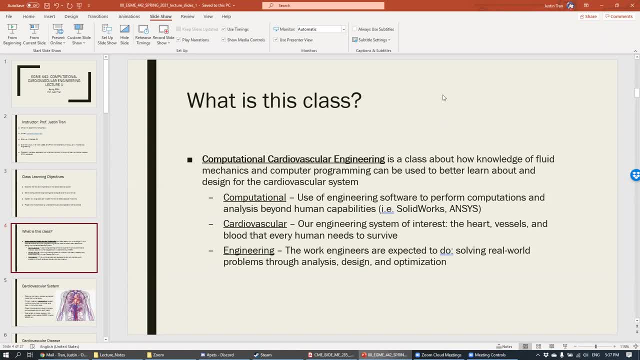 things like SOLIDWORKS and ANSYS, right, And so the things that you do in SOLIDWORKS and ANSYS, you know you wouldn't be able to do it by hand, because it's you know a computer is going to do. 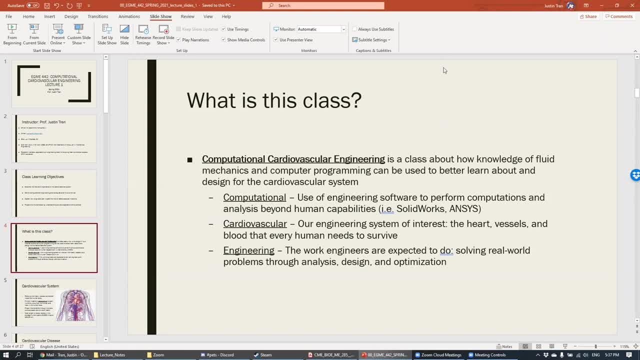 it. We're not going to use those softwares in this class. we're going to use a different software, But that's you know. I mentioned those there just because I know a lot of people are going to have experience with those and that's kind of you know what you can think about, okay. 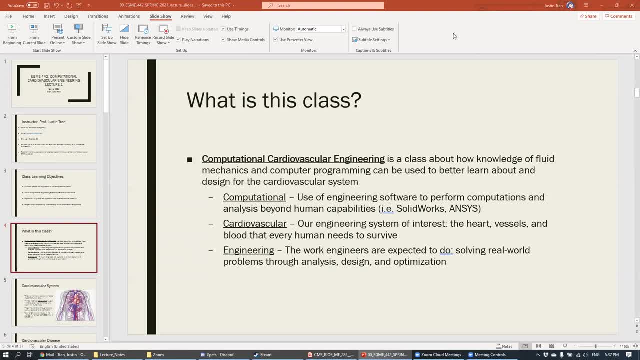 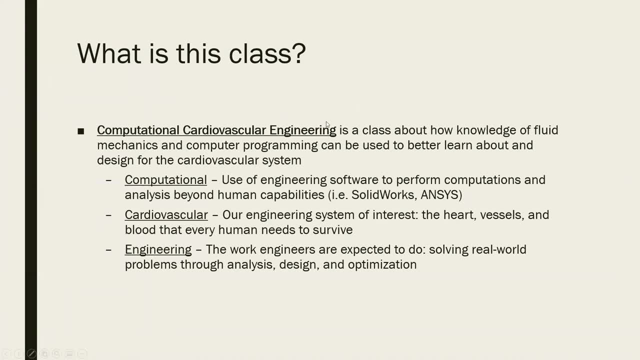 I see some questions in the chat. right, Okay, Okay, so let's do cardiovascular, right. And so when I say cardiovascular, that's basically our engineering system of interest, right? So whenever you know you're talking about engineering, you need to work on a certain kind of system. 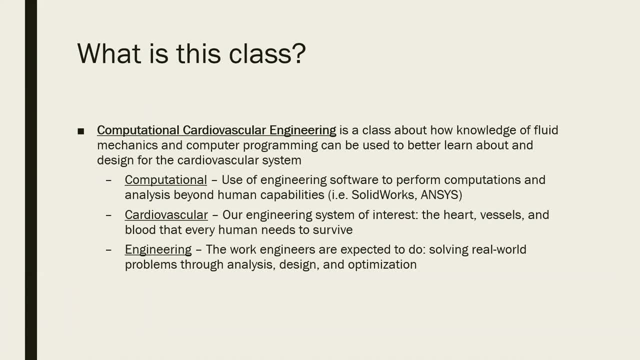 And so for this class, that's going to be our. you know the human cardiovascular system, So that includes your heart, your blood vessels and the blood you know that every human needs to survive in this world. okay, And so we're going to be studying those things pretty closely. 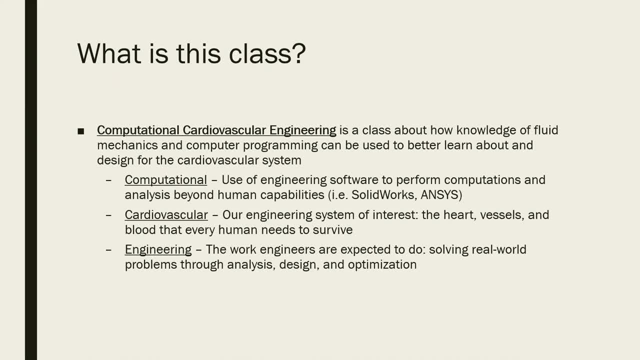 which is different, because usually we don't work in engineering curricula. you know we don't work on organic things like this and especially living things, And so hopefully you know that part is going to be interesting for you guys. So we're going to learn a lot of biology in this class. 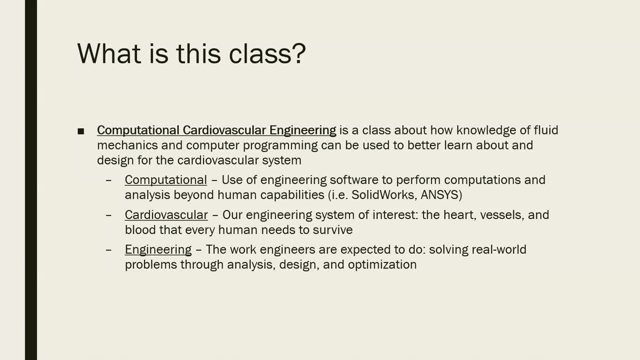 I know, when I started this work, I hadn't taken a biology class for like five years, ever since, like high school biology. So you know, I know for a lot of you guys it's going to be. you know we're basically going to be learning these things, but we're going to be learning these things and 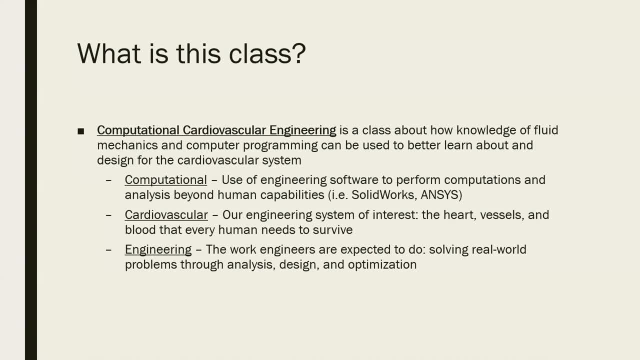 we're going to be learning these things from scratch. But don't worry, you know we're going to do basically reteach you guys all the anatomy stuff from scratch. But even better, you know we're going to be viewing these things from kind of an engineering mindset or an engineering lens. 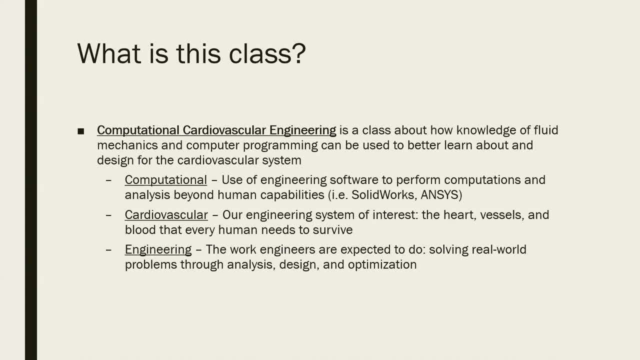 So you know, you might be thinking about, you might not think of your heart and your blood vessels, kind of the same way as you did before this class. okay, And then the last word in here is engineering. right, And so engineering, this just basically means just the work that engineers. 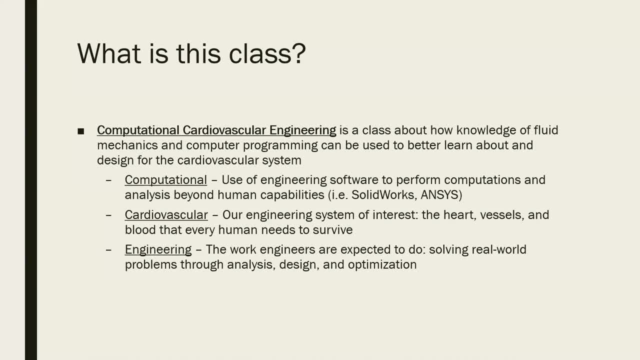 are expected to do right, And so a lot of times you know you're going to be thinking about engineering differently, but the way I like to think of it is: you know we solve problems right. We solve real world problems through analysis, design and optimization. okay, And so? 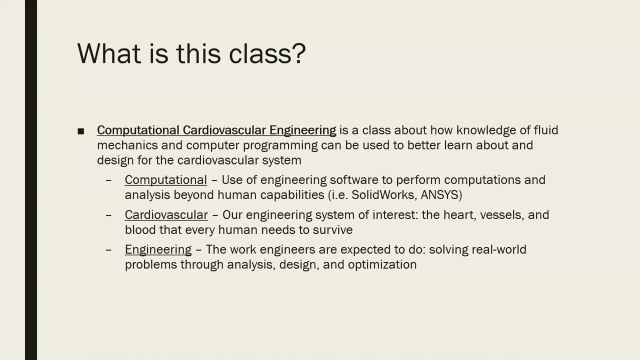 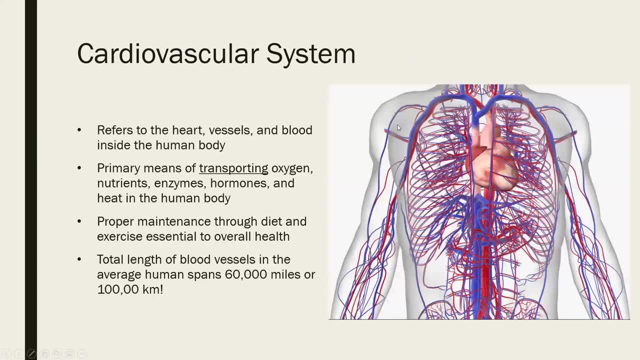 when we put these all together, we can say that you know this class is. you know we're going to use computer software, we're going to work on the cardiovascular system and we're going to do that to solve problems. okay, Okay, and so let's start talking a bit more. So you know, I promised you. 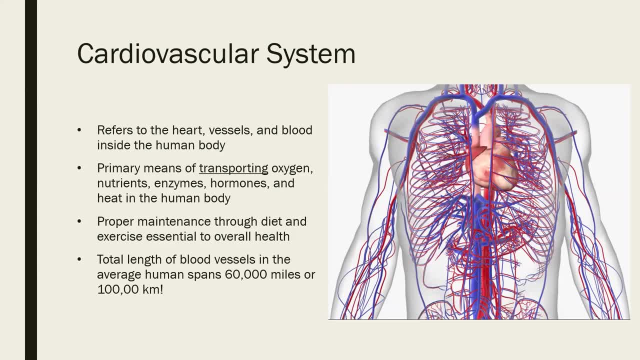 guys, some biology, and here's kind of the first kind of appetizer for it. okay, And so you know what is your cardiovascular system. And so the cardiovascular system refers to your heart, your blood vessels and all the blood that's in your human body, right? And so what I have on the 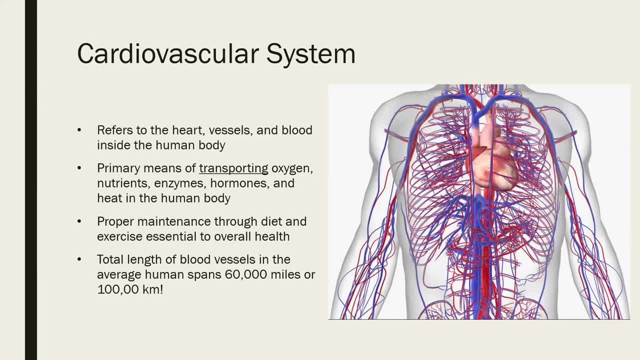 right here. this is just a graphic. you know, this is not an x-ray or something like that, but you know, as you can see, there's a ton of blood vessels that go through your body. okay, And so what is the purpose of the cardiovascular system, Which you know, ironically, which you know. 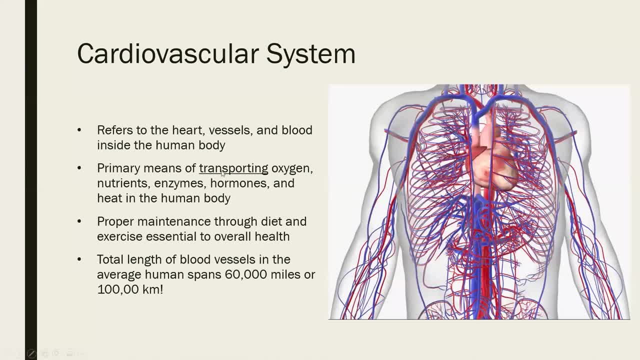 funnily enough, you know, when I first started this work, I didn't really think about you. know what's the point of the cardiovascular system? My thought is to bleed and make people squeamish, But you know the main function of the cardiovascular system. 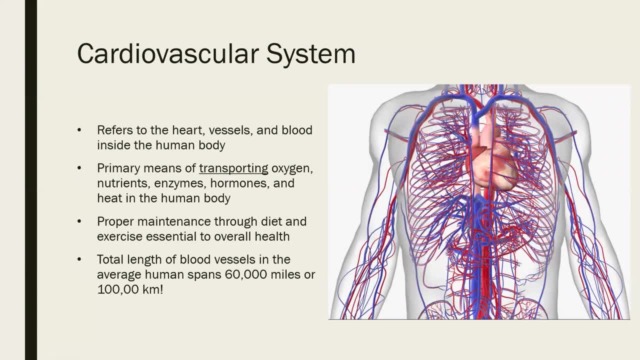 is actually. it's a transport mechanism, right? And so you know, all of the cells and all the muscles in your body: they need oxygen, they need nutrients, they need hormones, they need enzymes in order to perform their daily duties. But you know, if you think about it, the only place where 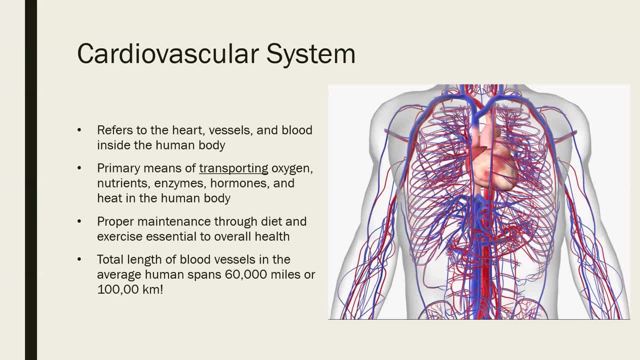 you absorb oxygen into your body is into your lungs, right, And so there needs to be a system that basically takes the oxygen from your lungs and then it takes the oxygen from your lungs and transports them to, like all your muscles, all your fingertips, you know, all your, you know. 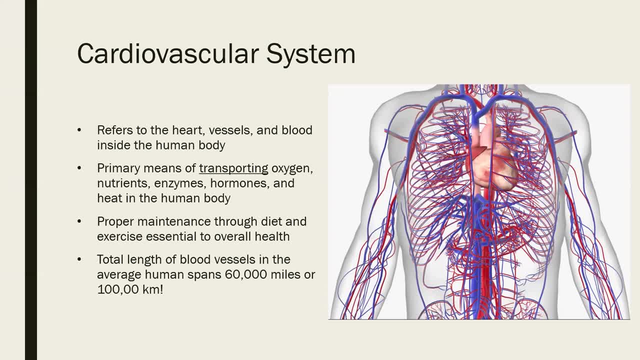 to your leg, to your brain and things like that, right? Not only that, you know, whenever you eat food and you absorb, like the nutrients and things like that, all that gets processed into your intestines, right, And so all of the you know- the protein, all the carbohydrates that you 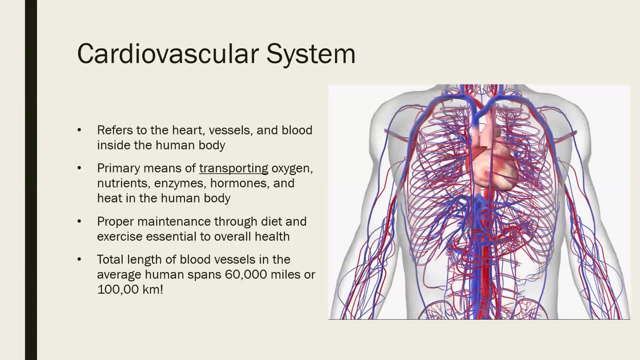 eat in your intestine. they need to get, they need. there needs to be some way for that to be transported to the different parts of your body, And the way that happens is the cardiovascular system, right, And so you can almost think of the cardiovascular system as a system, that's. 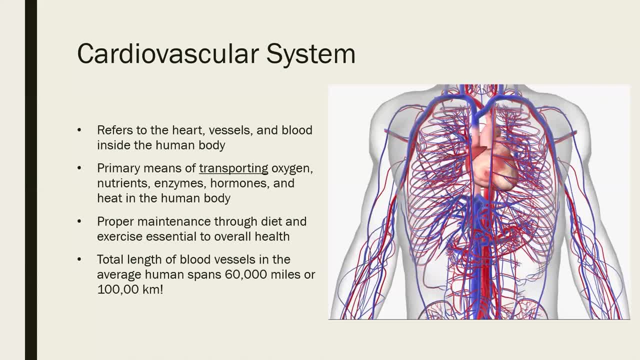 like the freeways and the trucks. you know that transport things throughout your body, So you know it's, it's. you see how important transportation is today. right, Uber is making you know tons of money, And so the cardiovascular system is kind of like the Uber of your, of your. 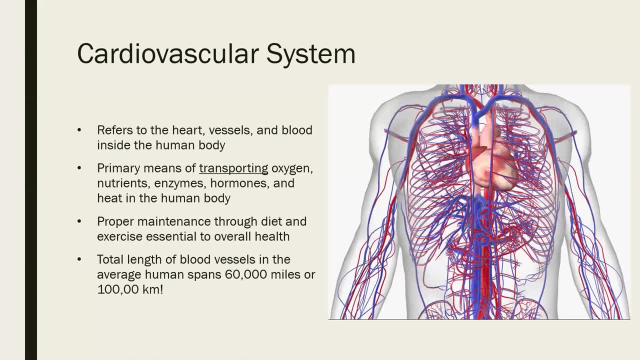 body right. And I think this next part, kind of everyone knows, is that you know, in order to be healthy, you know you need to maintain your cardiovascular system. So you know you eat a good diet, you need to exercise. well, you know, because if your cardiovascular system goes down, 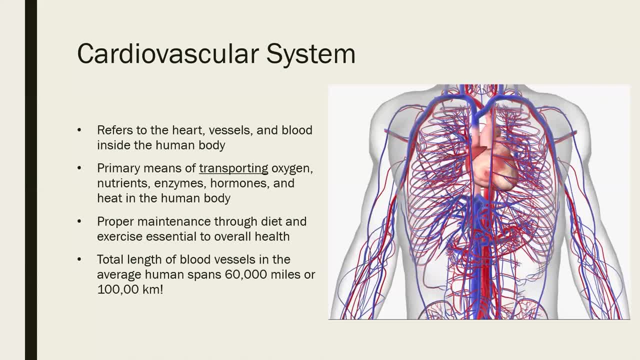 then there's- you know there's- it's really, it's a really vital part of your body, So you're not going to last very long, So you really need to get take good care of it. And an interesting fact: you have so many blood vessels in your body and it's so tightly packed that you take every. 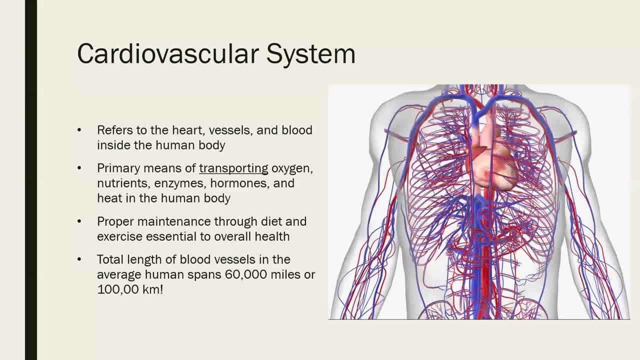 single blood vessel in your body and kind of laid it out kind of end to end. For the average human that would be 60,000 miles of blood vessels, or a hundred thousand kilometers. There should be another zero at the end there, And so there's a ton of blood vessels in your body, which is hard. 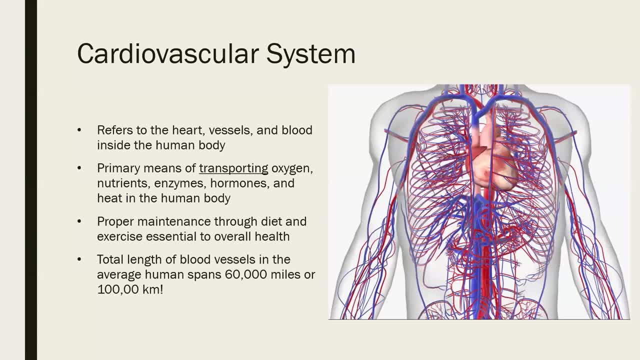 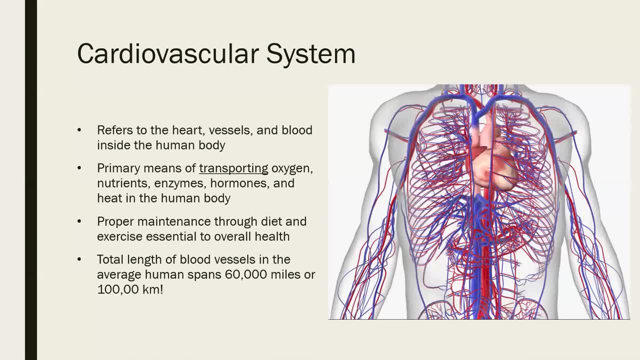 Right. So to know that there's 60,000 miles of blood vessels inside me, that's, that's kind of mind-blowing, Right. So it's, it's, it's fascinating And it feels like you know. 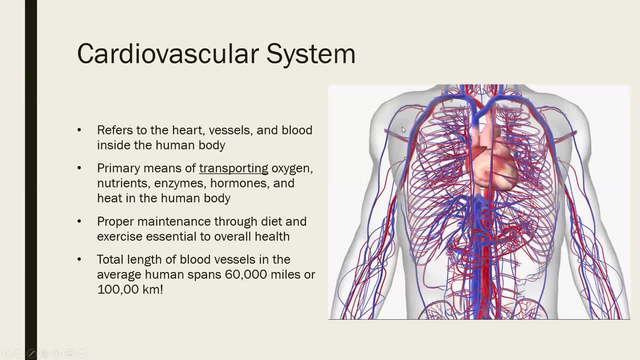 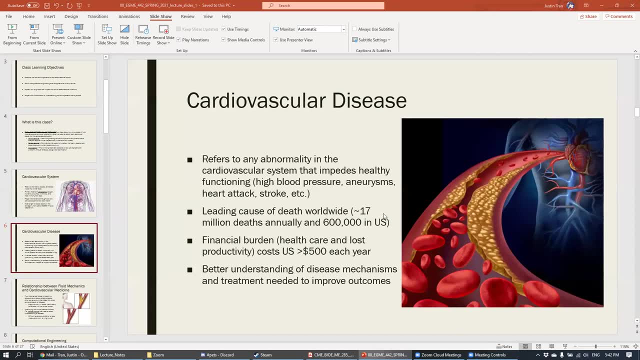 we've come a long way in understanding the cardiovascular system, but there's still so much that we don't know. still, All right, Question in the chat. Let me see. Yeah, I had the same response too. Okay, And so the next thing I want to talk about is: 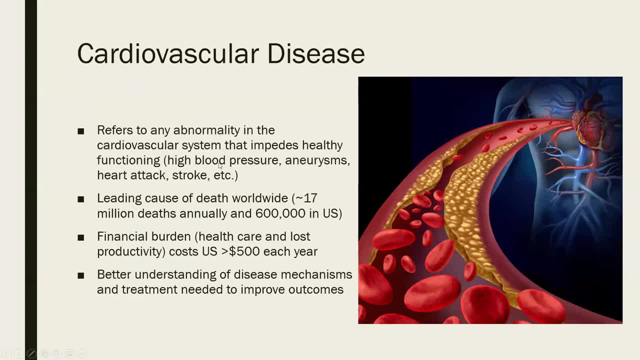 cardiovascular disease, And I'm going to talk about cardiovascular disease And I'm going to. So this is kind of a really big thing too, especially especially in America, So we struggle with this a lot, Right? And so when I talk about cardiovascular disease, what I basically 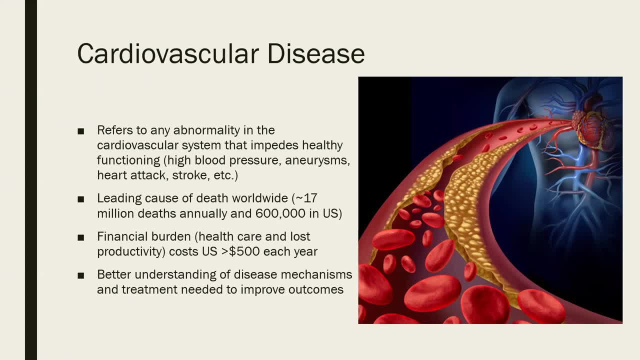 refer to as any abnormality in your blood vessels or your heart or anything that can impede healthy function. Right And so so some common diseases that you might've heard about is high blood pressure, aneurysm, heart attack, stroke. You know, what I have in the picture here is like: 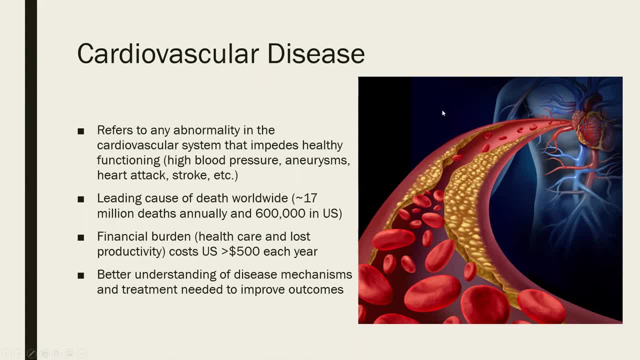 plaque buildup from, like fatty foods and things like that, Right? So anything that any kind of you know, anything that's going to impede healthy functioning of your cardiovascular system, that's going to be your. that's going to be considered disease. Okay. 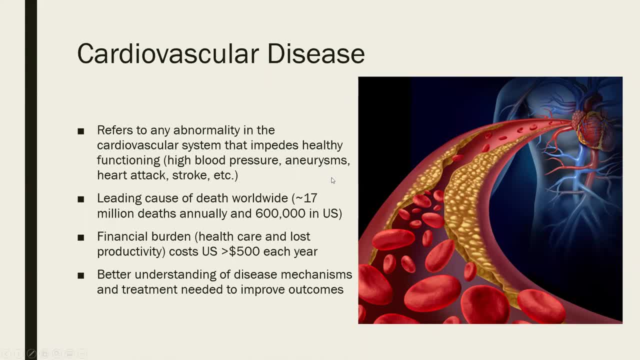 And, as I just mentioned, you know we have, you know we struggle with this, not only here in the U? S but throughout the world. Right. So you know, even even during COVID times, cardiovascular disease is still the leading cause of death worldwide. Right, And so about 17 million. 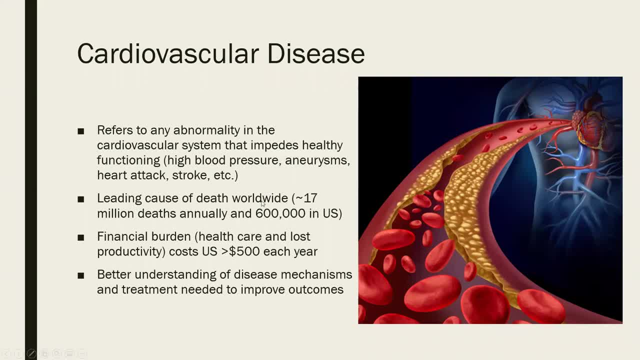 people in the world died from from cardiovascular disease each year, And about 600,000 of those are in the U S. okay, Not only is it the cost of life, but it's a huge financial burden too, Right? Um, oh, I forgot a number here. So, um, and so this is. this is an old number, So this was back. 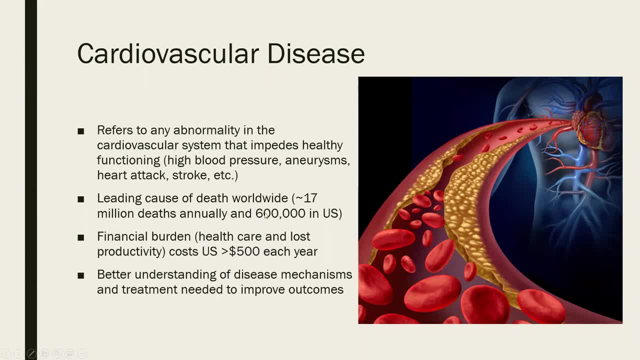 in 2010,. but in 2010, what they estimated was it costs the U S about 500, um billion dollars each year, uh, in terms of taking care of cardiovascular disease. So you know, that's that's money, that. 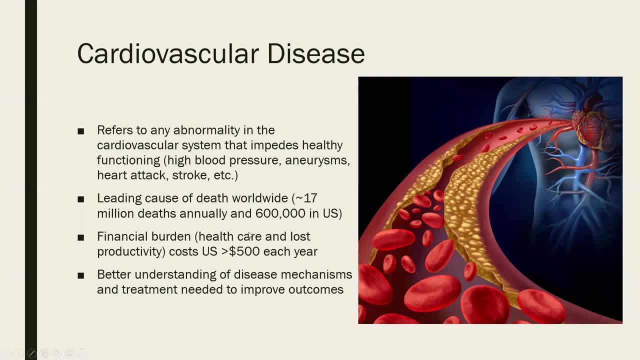 goes into hospital treatments, but it's also money in lost productivity too, Cause a lot of times you know: if you have a heart attack, you know you're going to be out from work from two weeks, Right, And so the financial burden that cardiovascular disease puts on our economy is 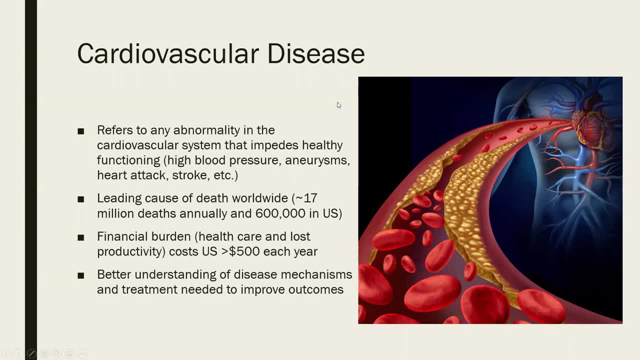 is really really huge as well. Okay, Um, and even though we've come a long way in terms of treating cardiovascular disease and understanding it, there's still so much work, there's still so much improvements that that can, that can be done Right. In order to do that, we we need to better understand. 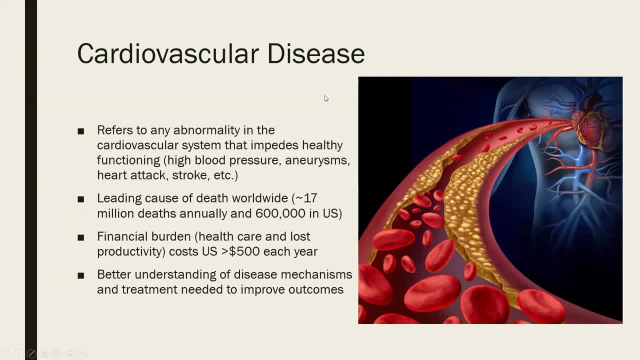 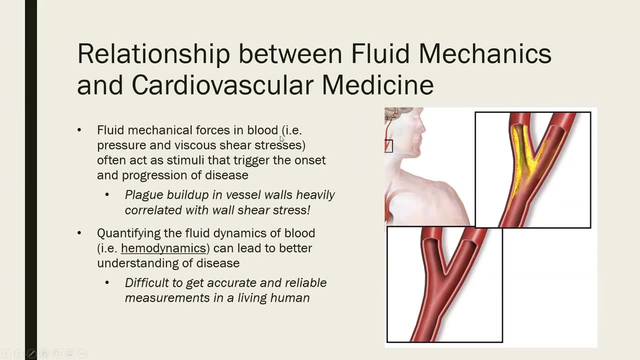 you know, how does disease, how does disease happen and how does it progress in the human body. Okay, Okay, And so what can what, uh, what can we do about that? Right, And so you know one. 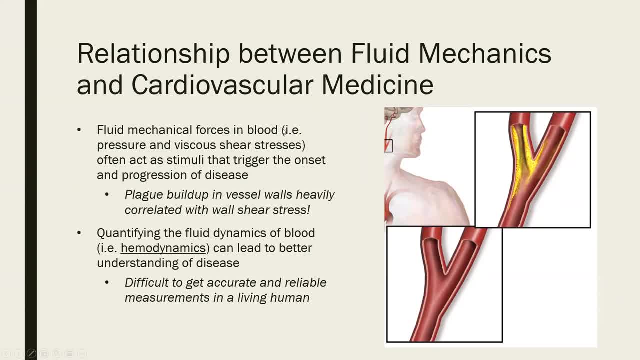 one way that we can better understand disease is to understand fluid mechanics, right, Um? because, like we just talked about, you know, your, your, your cardiovascular system is basically, you know, the transport system and it's basically, you know, a bunch of tubes in your body filled with blood. 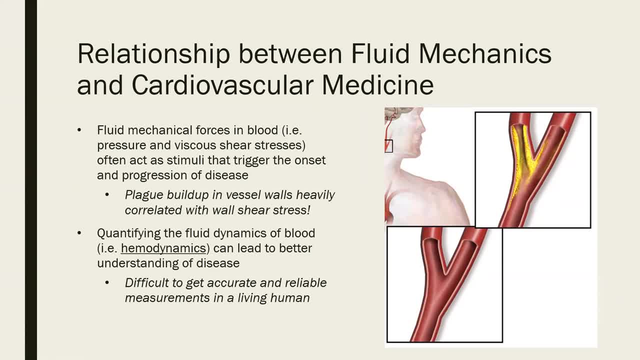 which is a fluid right. And so, just like the water in your faucet, you know blood is going to obey the same laws of fluid mechanics, right. And so if we can understand the fluid mechanics of your cardiovascular system, then maybe that's a that's, that's a step towards understanding. 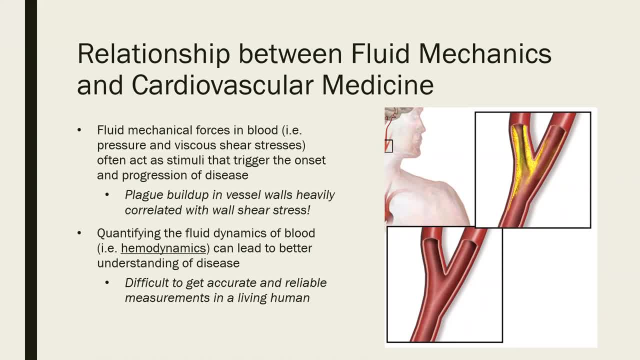 you know how can we better treat people with cardiovascular disease? Right, And in fact you know there's there's a ton of interest in this because there's a lot of studies out there that have shown that there's a lot of connections between fluid mechanics and disease, right And so. 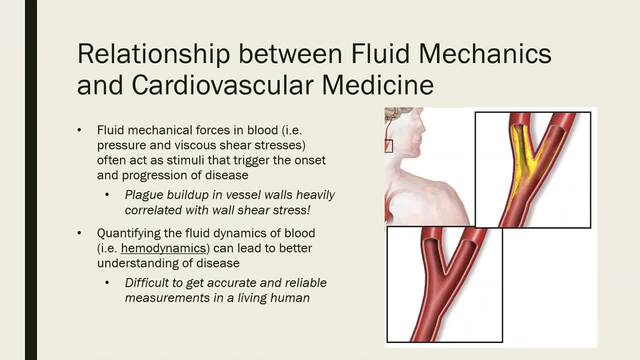 one, one famous example is that you know, uh, in terms of plaque buildup, right, Um, this is really heavily correlated with um, with the viscous, shear stress that you experience in the fluid. Okay, And so you know, if you remember from your fluids class, you know every fluid. 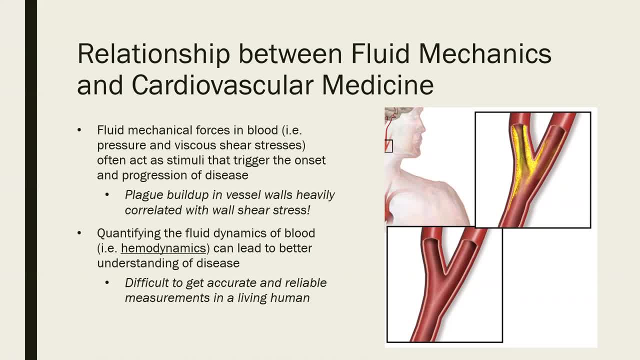 has some kind of viscosity And so the the shearing force or the shearing stress that occurs within the blood vessels, that's been heavily correlated with with disease, right, And so if we can better understand this, this, uh, you know this mechanism- this can help us maybe to 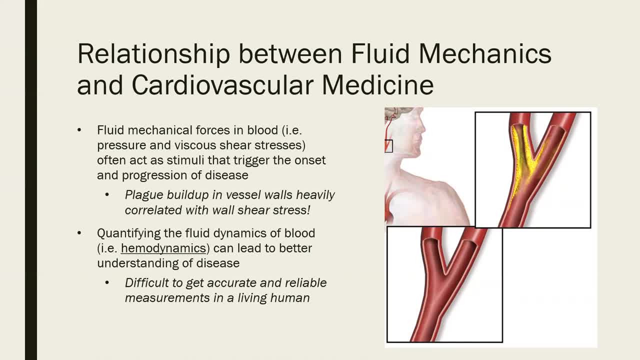 better design um treatment and devices to help with cardiovascular disease. Okay, Um, but the difficult thing about this is that, you know, most blood flow? um happens inside living people, Um, and it's really hard to get measurements inside a living person Um, because you know. 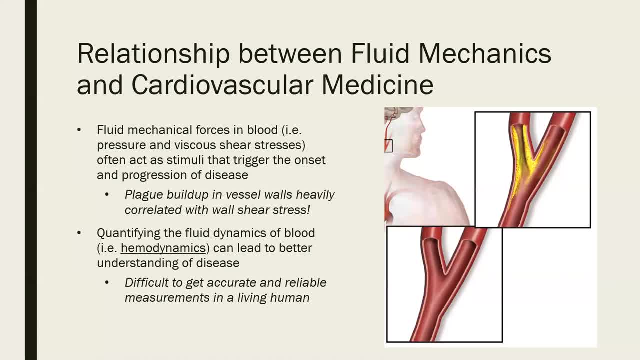 in order to get, like, basically, accurate measurements, you have to stick a probe inside someone. Um and no, uh, so and so that's that's. that's a. that's a really important process. So, if we can better understand this, this- uh, you know this mechanism- this can help us. 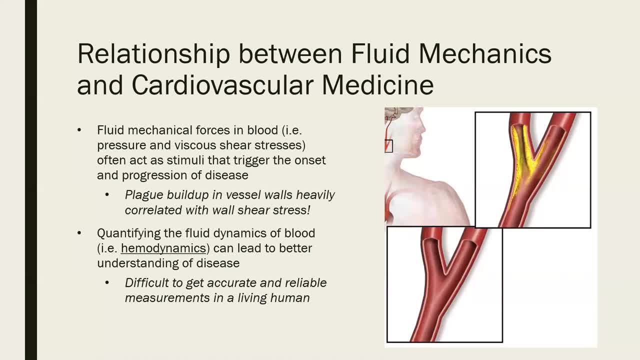 likes to do that, even if you pay them. you know you can't uh, do that for for too long, uh, and so we're really limited in how much data that we actually have on living. you know blood flow, just because you know we just we just can't measure it. just because you know all the blood. 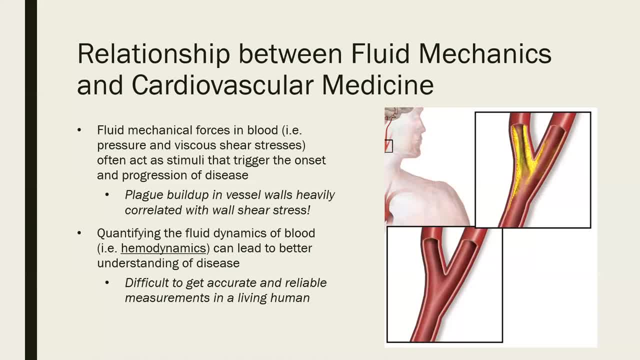 flow happens inside a person and actually, you know, as soon as you cut someone up to measure, you know you're kind of altering the blood flow in a certain way. so it's really difficult to actually get accurate and reliable measurements. um, in order to to form these, these correlations, 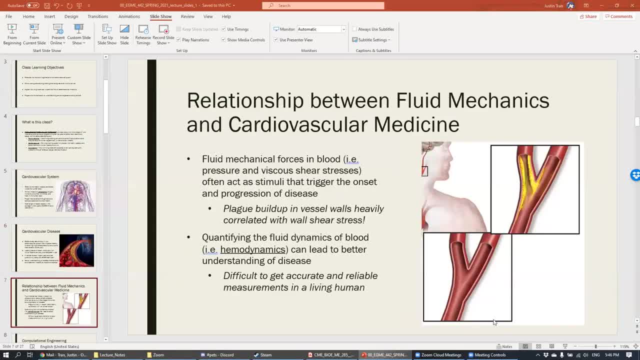 yeah, all right, question in the chat, let me see. oh so, question in the chat is: do we, are you supposed to take notes or just watch and listen? um, yeah, so the the lectures are recorded so you can definitely view them again um later. but i can definitely slow down a bit if you guys are are taking notes. yeah, 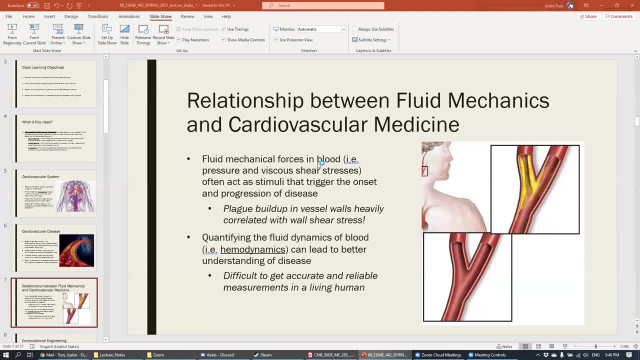 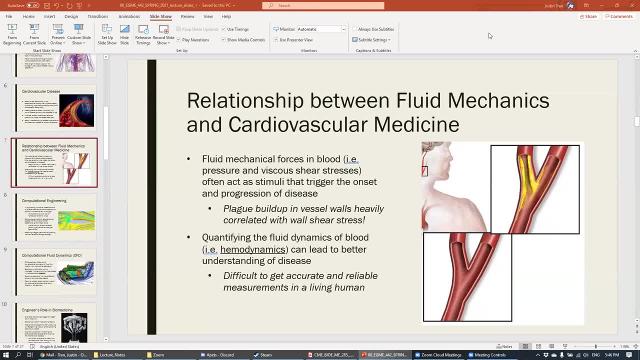 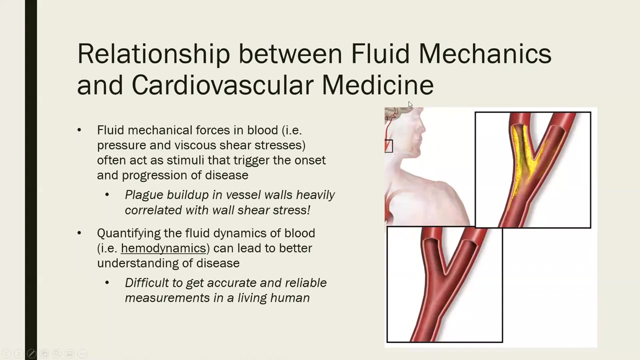 okay, um, so actually this is a good time to to stop. so, uh, are there any questions on on this? so far? okay, oh, question, okay, okay, um, and so we kind of have this issue right now where you know it's it's really hard to measure and quantify the, the fluid mechanics, even though even though we know that there's a correlation. 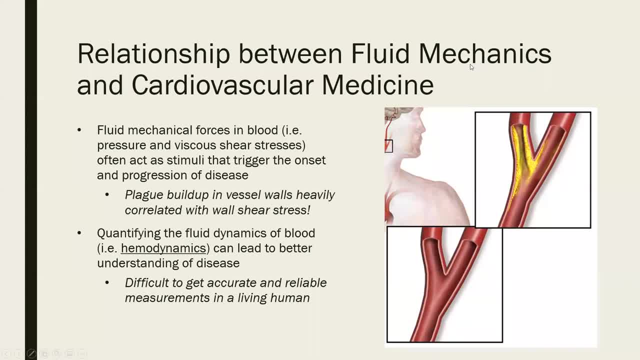 okay. and so in these situations- you know this is not um an uncommon occurrence in engineering, because in engineering we have a lot of similar things, uh, where you know it's really hard to get measurements, like you know it's really hard to get measurements on like a rocket. 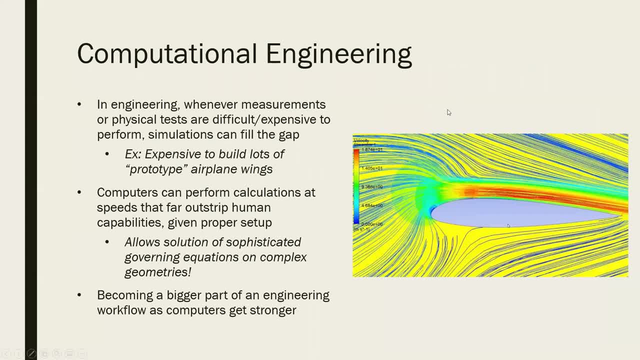 chip, that's, that's leaving the atmosphere right, and those situations you know, in engineering, what we've done is we've relied on simulations, okay, and this is where the computations come into play, okay, and so whenever, you know, whenever we have, we were forced- we're faced with a situation where 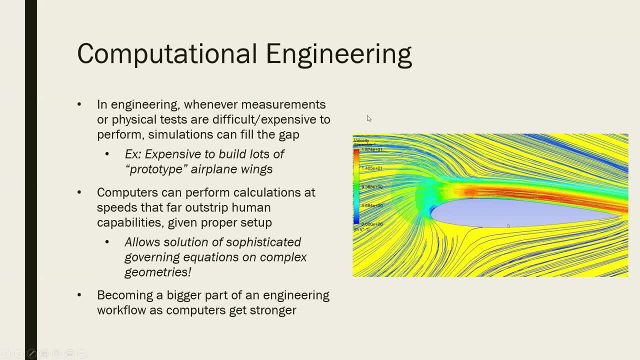 physical test, um, or a physical experiment is really difficult to perform. uh, we can, we can do a simulation to basically, you know, predict what's going to happen, okay, um, and one example of this, which happens a lot in aerospace, is that you know it's really expensive to to, you know, build prototypes and to run experiments on things like an airplane wing. 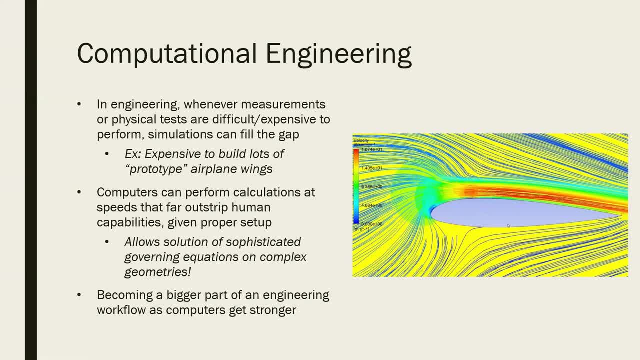 right, and so you know, uh, boeing is not going to build an airplane wing just for the sake of testing, right, it might build one or two, but they're not going to build like 20 of them. just so you know, just so that we can test them, and so a lot of the engineering work, that's that's done at these. 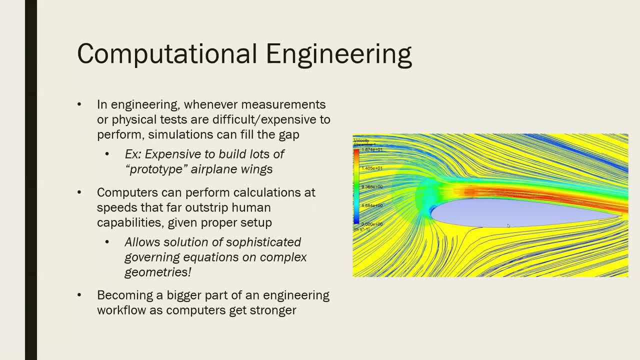 companies is actually done on the computers. okay, because they're not going to build like 20 of them. because on the computers what we can do is we can set up simulations, um, that mimic these, um, these conditions, um, so that we can, you know, find out what's happening without having to perform a. 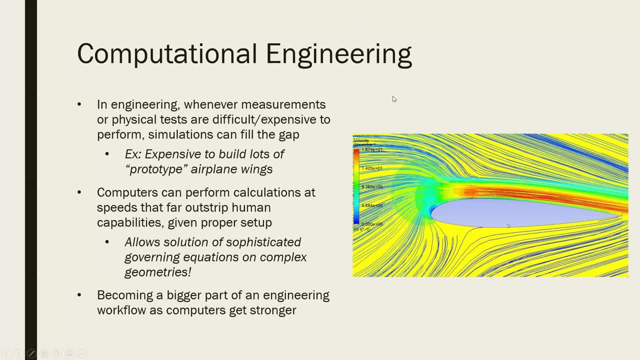 you know, physical test, okay, um, and the, and the cool thing is, as computers get stronger and stronger, you know this- this branch of engineering, computational, is becoming, you know, a bigger and bigger part of the workflow where, you know, as we, as, as you know, we can perform more calculations. 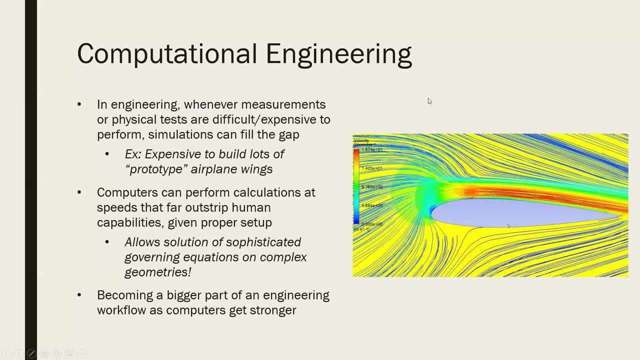 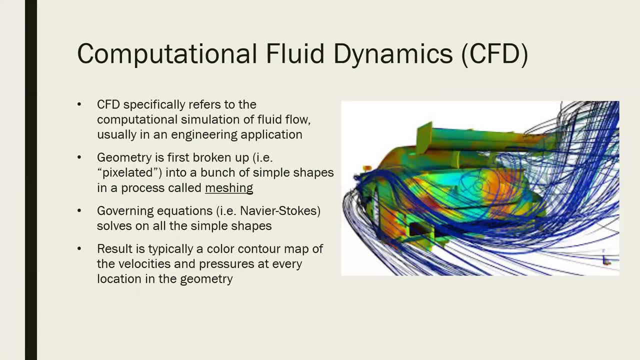 and the more that we can trust them. you know this is, this is becoming a much more viable option, okay. okay, and so let's talk about in specifically computational fluid dynamics, or cfd. okay, and so you might have heard the acronym cfd before, but cfd um is a special kind of simulation that that. 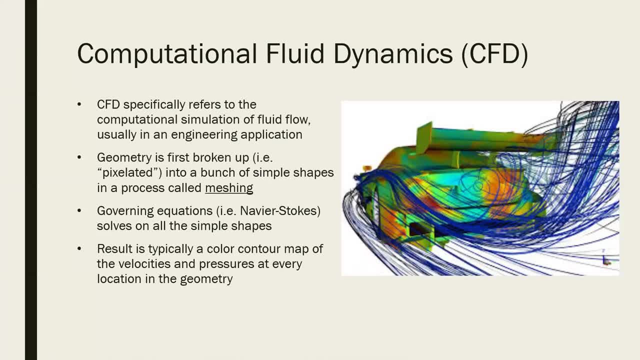 refers to just fluid flow. okay, and so you can run a simulation on lots of different things, so i think the the most common one is for structural simulations. um, that's typically done in elements, but any simulation that involves fluids is known as cfd. okay, and so that's what. that's what. 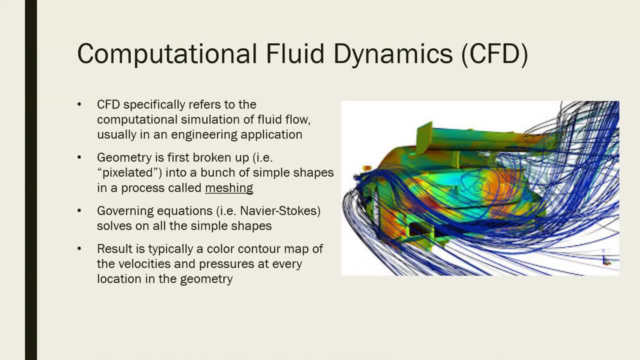 we're going to be using in this class too, actually. so, um, for your final project, which you know we'll talk about later, um, you're going to be running a cfd simulation on blood flow inside a on a certain part of the body. so you know that part. hopefully, you guys, uh, hopefully that part will be really 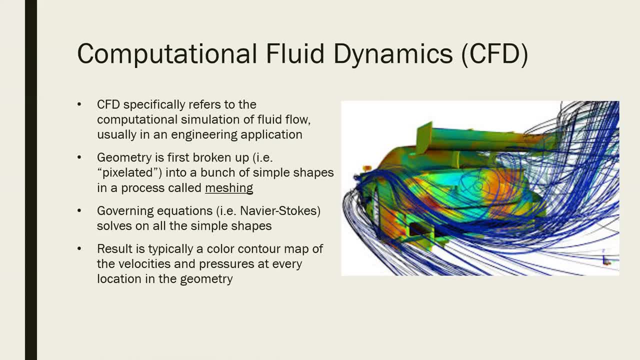 cool for you guys, okay, um, and so just very quickly, just the the process of running a cfd simulation is that the first thing that we have to do is we have to take our geometry and then break it up into, uh, simple shapes, okay, and so this is a process called meshing, right, uh? and then, once we've meshed our geometry, we can then 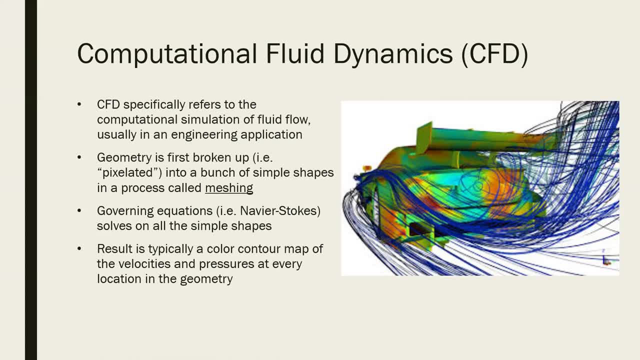 take our governing equations, which is, nab your stokes and then solve that equation on all of our simple shapes, okay, and then, once we run that simulation, we can then present the results as kind of a color contour map, and so that's basically what you're seeing on the right right. 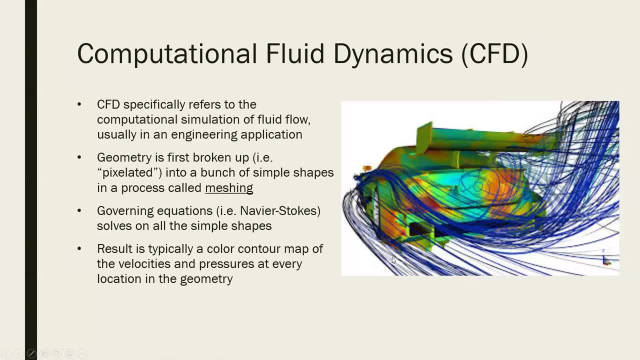 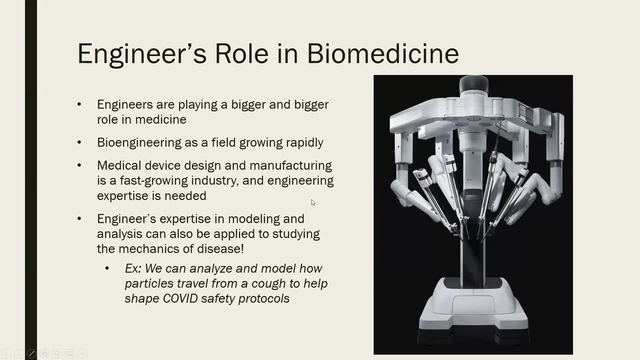 here. so, on the right, uh, what you're seeing is a cfd simulation of a sports car that's basically driving down the freeway, okay, so you're seeing kind of the wind patterns that are flowing past the, uh, the car. okay, okay, um, and we can use tools like this and other- you know other- of our engineering analysis to 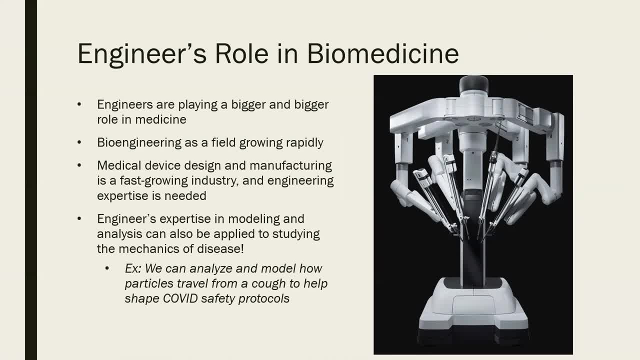 impact biomedicine? okay, and in fact it's, it's, it's a field that's growing more and more and more, okay, and so you know, not only in analysis, but also in manufacturing, um, and also in device design, engineers are playing a bigger, bigger role in medicine. okay, um. so, yeah, we've talked about 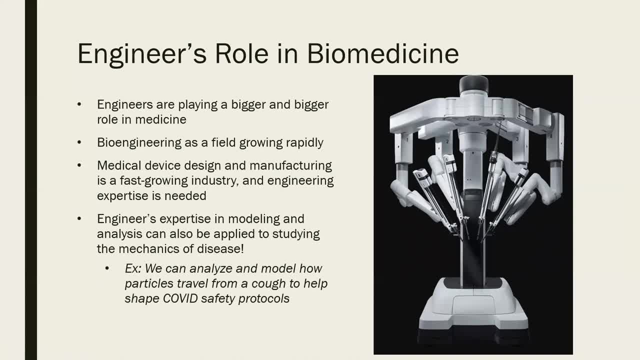 you know medical device design and manufacturing. you know engineering expertise is is needed for that, and also you know for modeling and analysis. you know we're starting to see that. you know, like see it, things like cfd can be used to- uh, to analyze things as well. okay, and so one example: 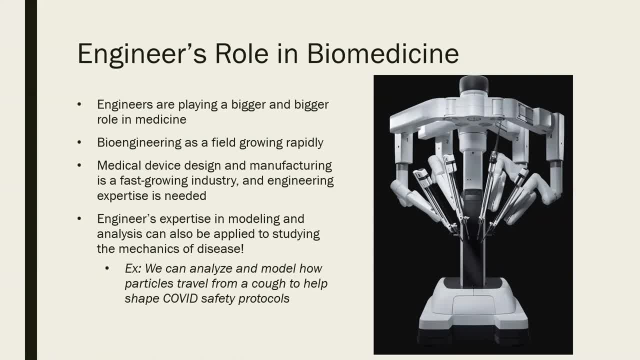 you know i've seen some work that people have done is they've run cfd simulations to see that they can, you know, see how far covid particles travel in the air, and so information from simulation like these can be used to, you know, to better shape covid safety protocols okay. 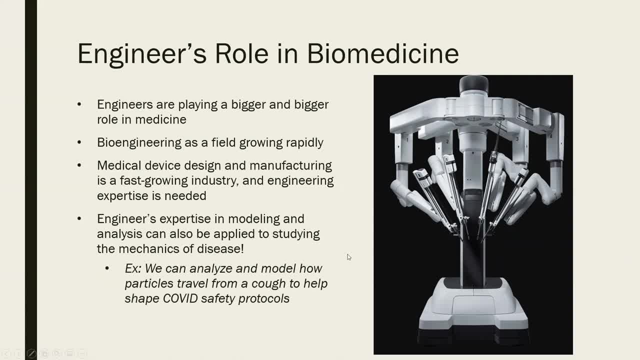 um, and so this kind of scary device that i have on the right right here, this is actually a surgical robot, and so this is another really interesting field. um, that i, you know, admittedly don't know that much about, but i think is really cool, is that you know a lot of. 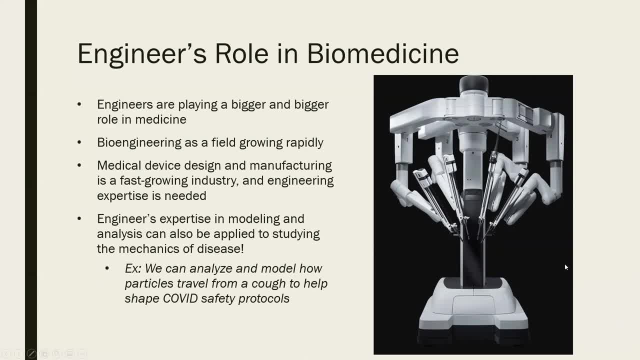 surgeries, or a lot of hospitals nowadays are invested in the medical field and they're investing in machines like this to kind of help assist someone with with assist the surgeon with surgery, okay, and so what you can imagine is that down here, you know, we have a patient that's laying. 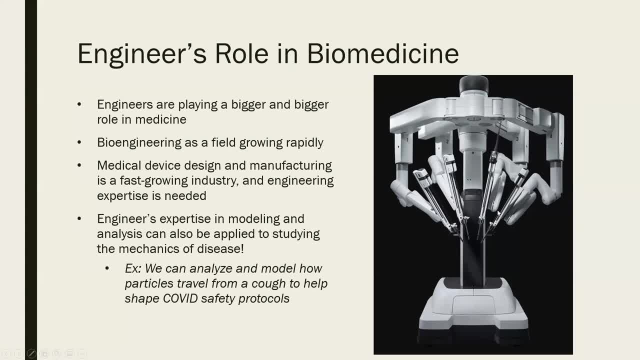 down and then you know these, all these arms right here contain all the different tools and with a device like this, the surgeon's actually not even looking on top of the patient. the surgeon's on the other side of the room on his computer. you know, basically operating these? 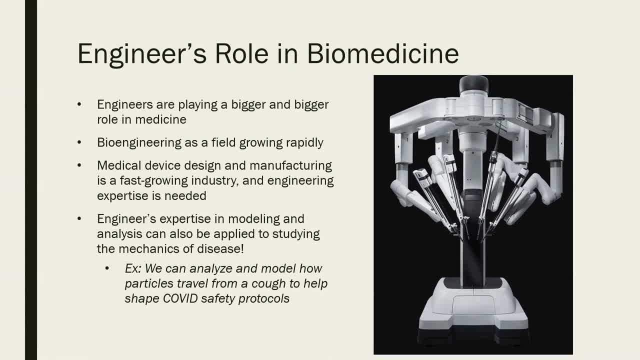 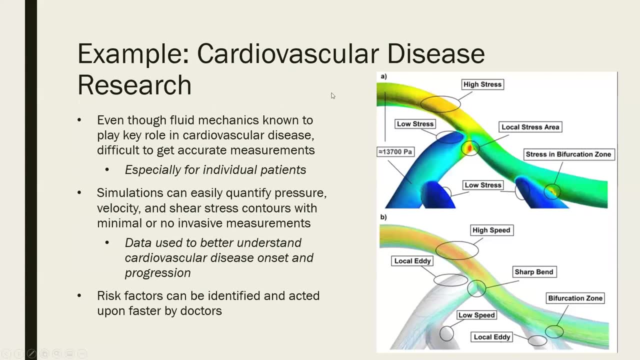 these four arms kind of like a wizard of oz type of thing. so it looks kind of scary. so it looks kind of like something you might fight in, like final fantasy 7 or something like that. but you know, this is, this is a, an emerging field that uh, you know that's becoming bigger and bigger. yeah, okay, um, and so are there any questions on? 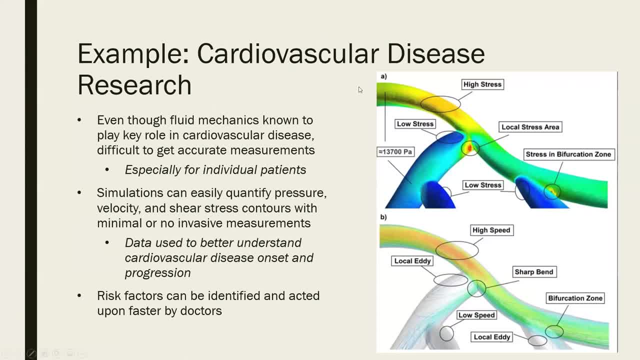 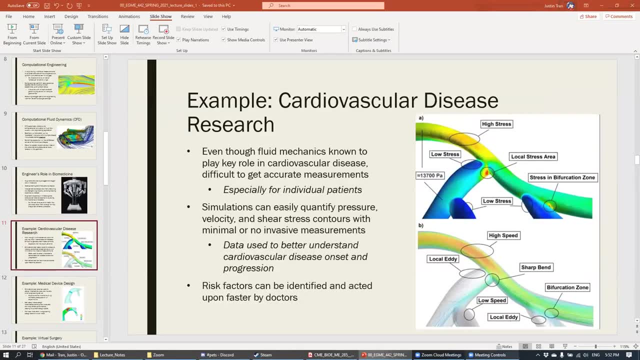 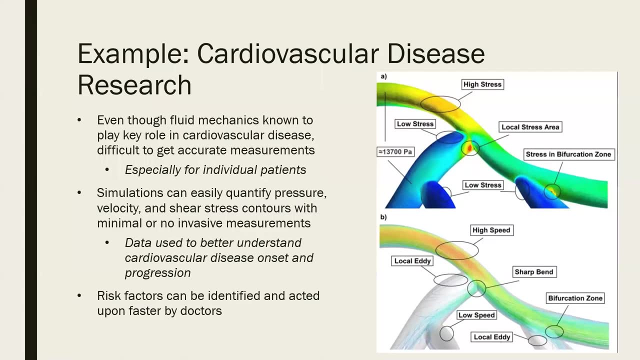 any of this at at this point? sorry question, cool, yeah, okay, okay. so what are some examples on on which we can use? um, you know cfd, right, and so one example this is: this is kind of the area that i worked on a lot- is to study cardiovascular disease. okay, 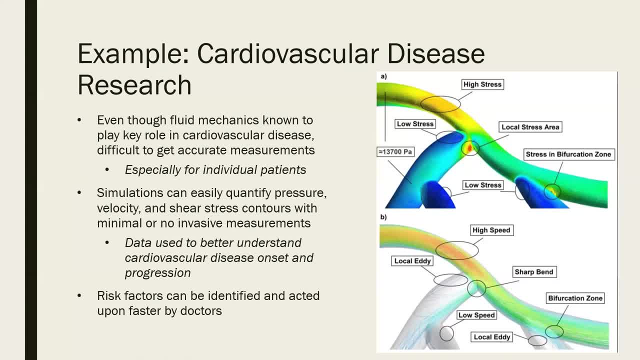 uh, and so just like we talked about you know, we know as as kind of as a field, that fluid mechanics plays a really big role in cardiovascular disease. um, you know there's been a lot of experiments that that have shown this and just naturally you just kind of it's just kind of obvious, just because 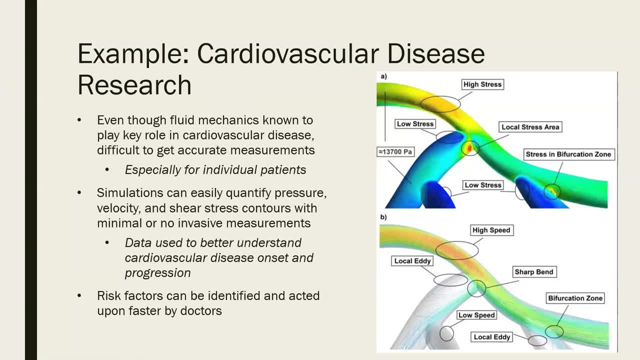 you know you have, you have a, a fluid that's flowing in a pipe. you know the physics of that flow are gonna are gonna affect, you know, things like disease and things like that. okay, um, and so what we can do in simulations is we can use them to quantify things like the pressure, things like the velocity, things like the shear. 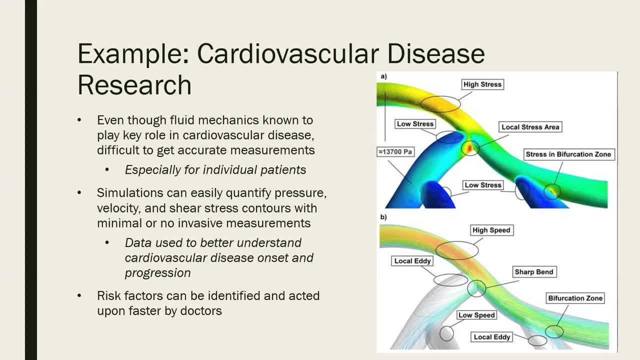 stress, um, which you know, normally would be basically impossible to measure in a person without sticking a probe inside them, right, um? but with simulations you can do this, you can basically simulate it without having to, you know, stick something inside someone, and in the field we usually call that invasive measurements because, you know, we call 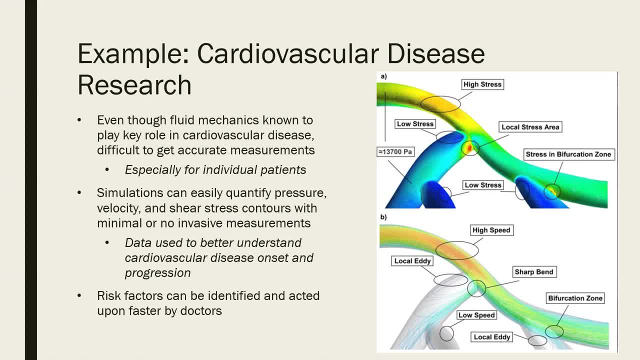 invasive because it's you have a probe that's invading your, your body. okay, and so we can basically use this data to better understand. you know, how does cardiovascular disease start and how does it progress in a person? okay, because even in situations where you do stick can stick a. 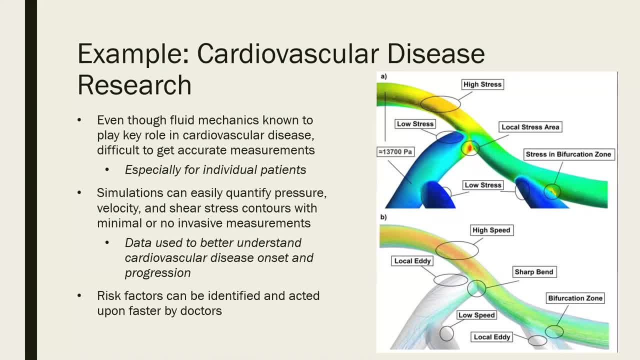 probe in someone. you know they're not going to walk around with that probe with them all day, okay, and the unfortunate thing is, you know a lot of diseases, they take a while. they take a while to develop. so they take, you know, uh, months, sometimes years, to develop, and so someone's not going to walk. 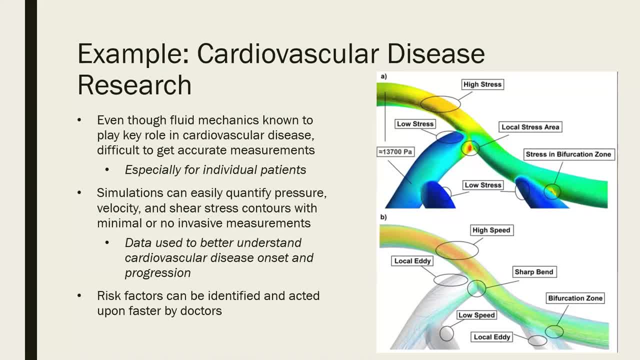 around with the probe inside their body, you know, even for research purposes, for you know, months and for years, and and so what we can do is we can use simulations to decide this. okay, and if we can better understand these disease um mechanics, then what we can do is we can assign better risk. 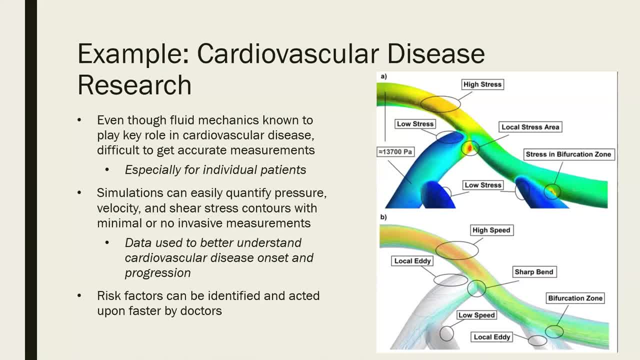 factors to people um, as well. so we can say: you know, based on you know, a simulation, or this is kind of the. the goal is that, based on a simulation of someone's you know of their heart or something, we can say that you're at a big risk of. you know, maybe heart. 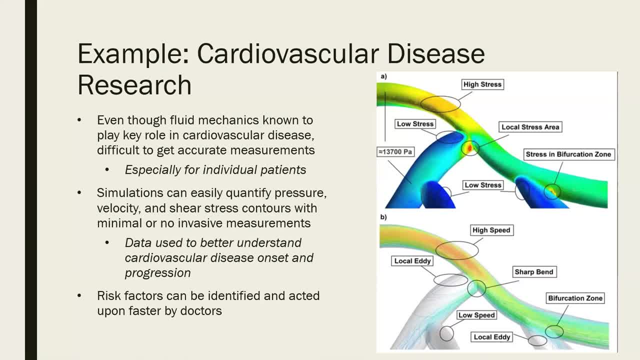 failure in 10 years. so you know, maybe we can do this. you know um preemptive surgery, to kind of help you with that right um, because i don't know if you've heard this term in medicine before- that said, an ounce of prevention is worth a pound of cure, right, and so if you can stop something bad, 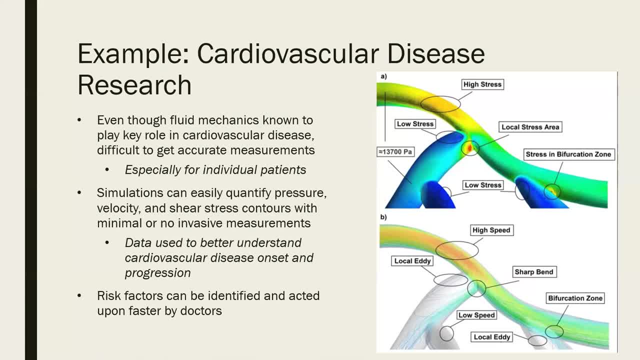 from happening. that's way easier and way better than if something bad happened, than if you tried to fix it right. and so if you can stop people from having a heart attack, that's way better than trying to treat people with a heart attack right. and so if you can stop people from having a heart attack, 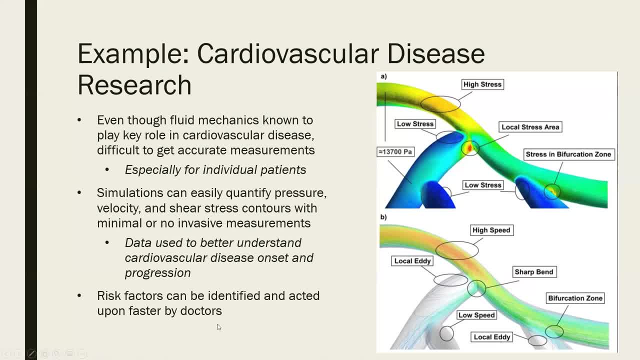 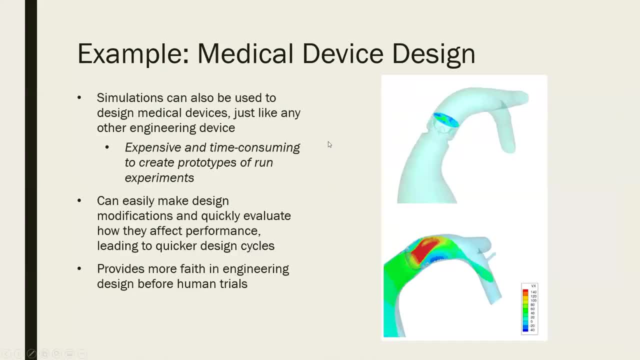 and trying to, you know, manage that right, and so if we can use simulations to try to determine this ahead of time, that would be a huge um, a huge bonus, okay, okay. and so another field that's really interesting is we can use simulations to better design medical devices, right, and so you know the 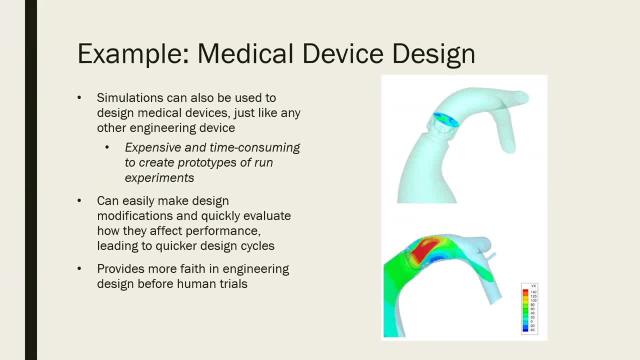 the field of medical devices keeps growing and growing. so, you know, people are coming up with all kinds of crazy devices that they can stick inside your body, right? um, and you know, just like any other kind of engineering device, we can use simulations to better design them, right? uh, and so, just like we talked about in the beginning, 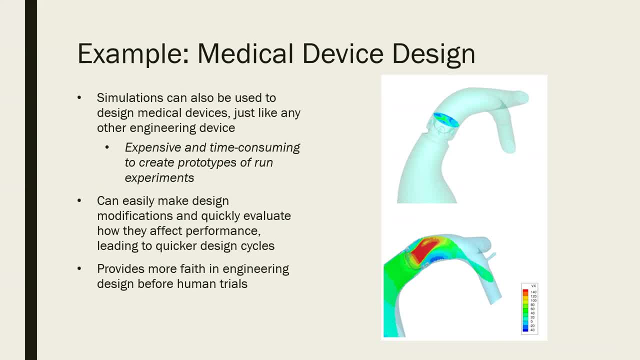 with the airplane wing right, and so you know how boeing uses simulations to design their airplane wings. we can also use simulations to design better medical devices too, because, you know, in order to run experiments, it's just really expensive and time consuming. okay, and the nice thing about a 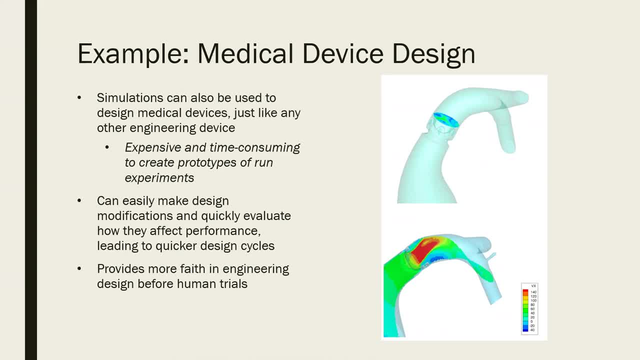 virtual platform with simulations is that you can make design modifications and just very quickly you can evaluate how they actually perform, and so this leads to quicker design cycle and you know better products overall. okay, um, and what this helps with is that you know before you actually start testing things on humans- you can actually simulate them first. uh, you know, just to. 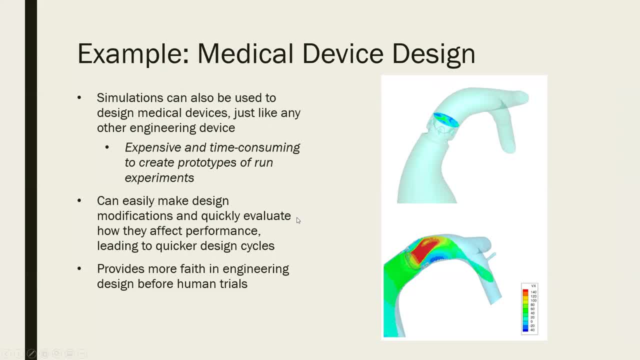 kind of provide some more faith. so you know you're not sticking a valve into someone and say: you know this is kind of the first time that we're trying this. so, um, you know, with simulations it's a little better than that. okay, all right, and so the a third area, and so this is not the the last one, but 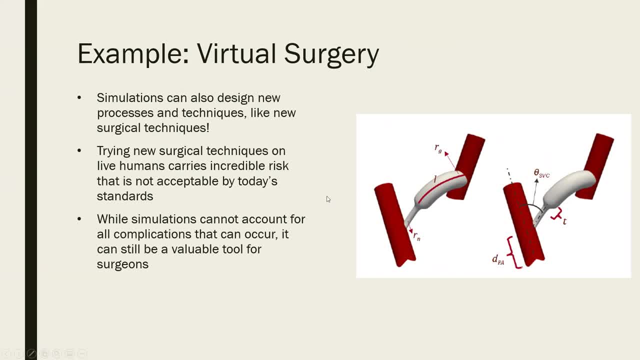 certainly a very exciting one, and i'm going to go ahead and show you a little bit more of the exciting one is that you can perform virtual surgeries right, and so you can actually use surgery. you can use simulations, say you know, you know. a surgeon can come to you and say you know. 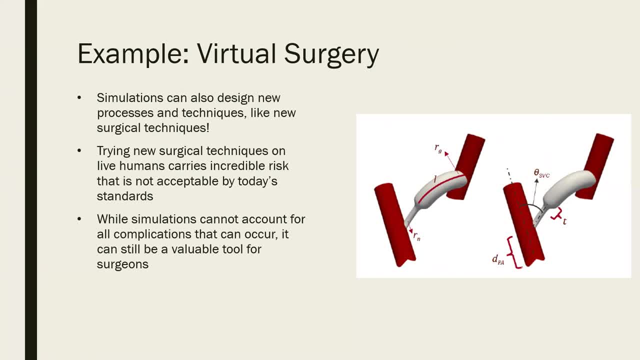 i'm thinking about trying this new surgery on someone, but i don't want to try it out on a new person, right, um? and so you can use simulations to basically simulate how that's going to be, you know, before they actually try it, right? because you know, we live in kind of a world today where 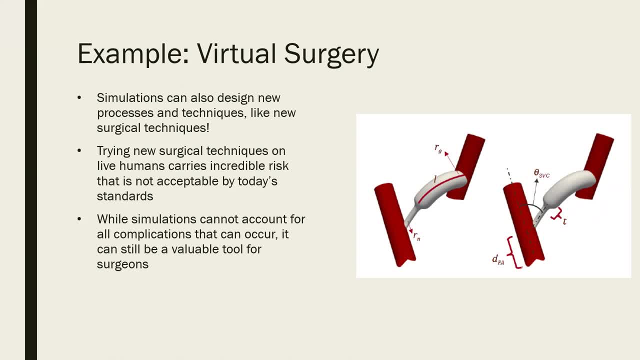 like you know, when you try trying any kind of new surgical techniques on humans, it carries an amount of risk, um, and so actually back in the day, you know, when medicine hasn't advanced too far, you know, this was actually pretty easy to to do, to just try something new on someone right. um, i remember a 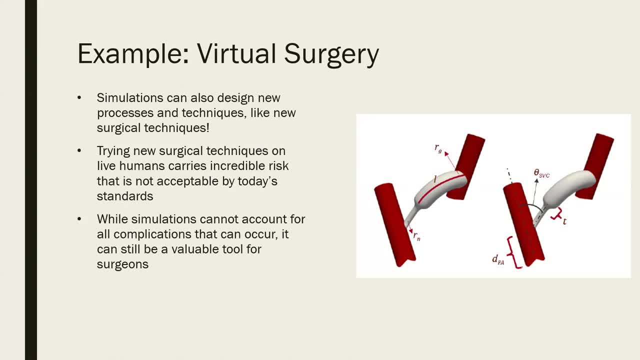 conversation i had with the surgeon, uh, and you know he was kind of famous for kind of discovering a certain kind of surgery- and i said i asked him: you know, so i like how did you come up with this? like this is kind of a really brilliant design. and he said you know, honestly, you know he's kind 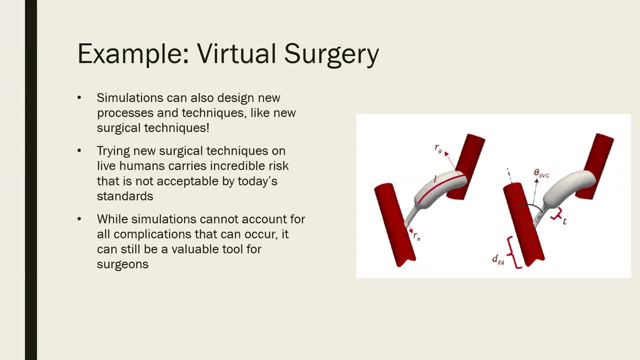 of an older guy, so you know he's kind of in his late 50s. he said: you know, back when i was first, the standards were a lot lower back then. so basically what happened was that a patient with this condition came in and nobody knew what to do. he said: so i just tried something and it. 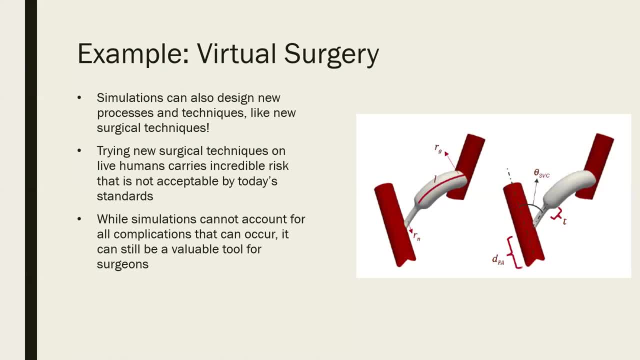 worked and now i'm famous for it and, like i was, i was kind of dumbfounded that like that was kind of the the process that he went through, because back then, you know, he basically said that if he tried something, you know, and the patient passed away, then you know, then that's just that's kind of 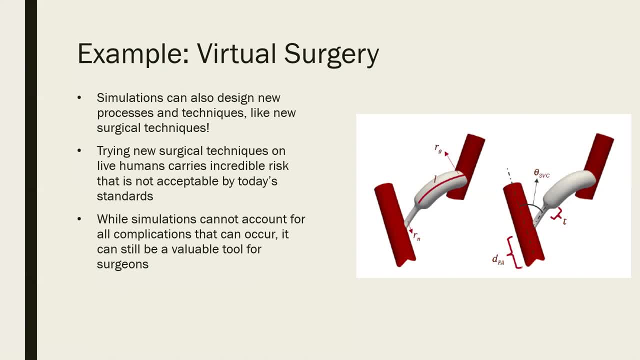 the expected outcome, and so he had kind of the freedom to kind of try something new. but in in the end, you know, it didn't come a long way, so you can't really do that anymore. so you know, and if you want to try a new surgical procedure, you have to kind of try it in simulations first and you 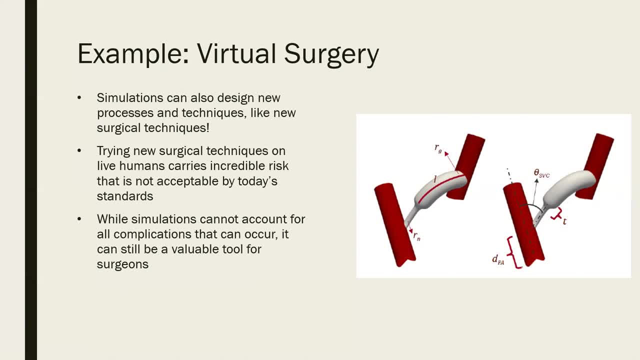 have to go through a really long process before you actually try it in a human right. um, and i will say that you know, surgery is a very complicated, you know thing. so a simulation can account for all the complications that occur, but it can still be a valuable tool because it can. it can you know. 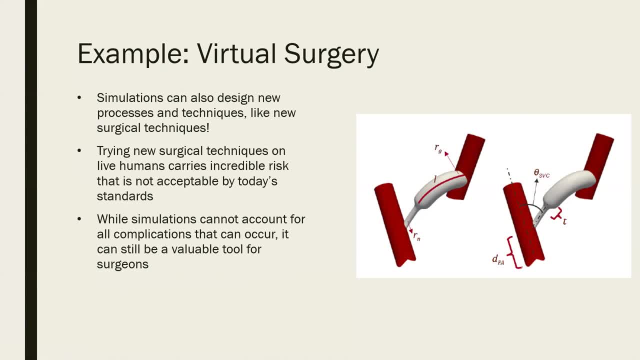 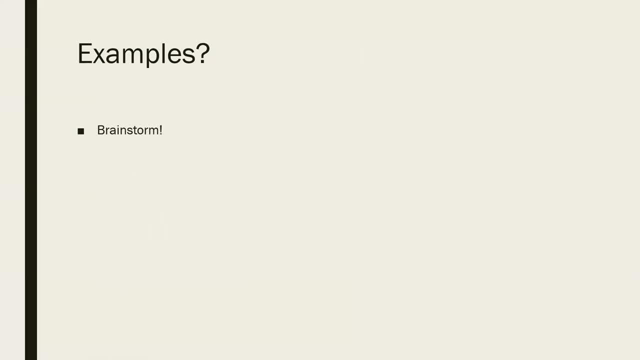 it can give you an idea of how things are going to perform before you actually do it in practice. okay, uh, and so at this point, you know, i want to turn it to you guys because it's you know, um, i know there's a lot of you guys have a lot of interest in the biomedical field. 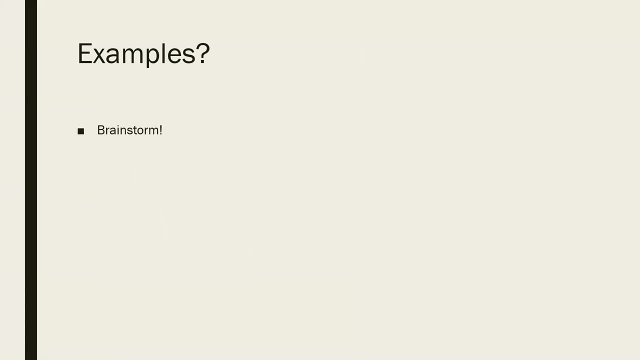 and so are there any kind of you know things in the cardiovascular system or anything biomedical in general. you know that you want to um, that you want to learn about, because i think you know this is probably one of the only offerings that we have at cal state fortum that have to do with 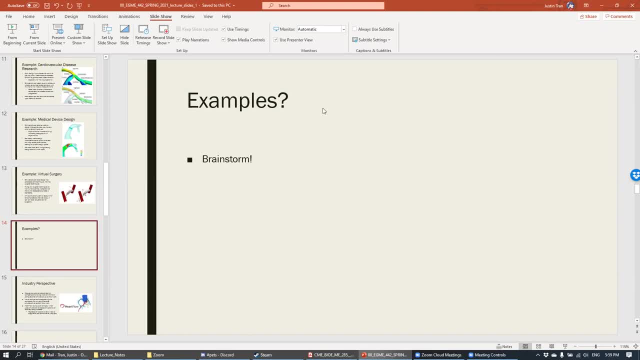 bioengineering, so anything bioengineering related or biomedical. just go ahead and shout them out. you know, and this is this is the time to share- uh, heart transplants, heart transplants, yeah, that's a, that's, that's a very, very interesting um field, because it's, uh, it's, it's one of the most complicated surgeries out there. 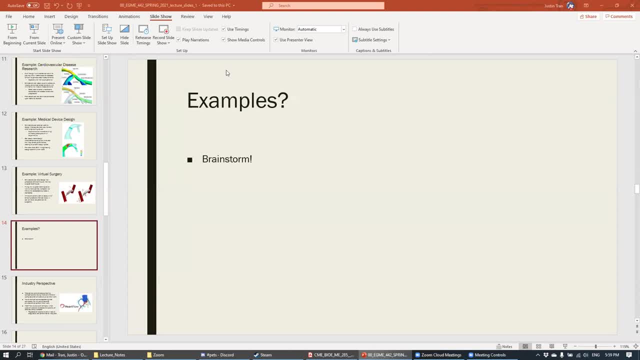 and so, um, i know that there, in terms of simulations, there hasn't been um, a lot of uh of um attempts on that yet, but you know it's, it's definitely something that's out there and definitely something that we want to improve as well. okay, okay. 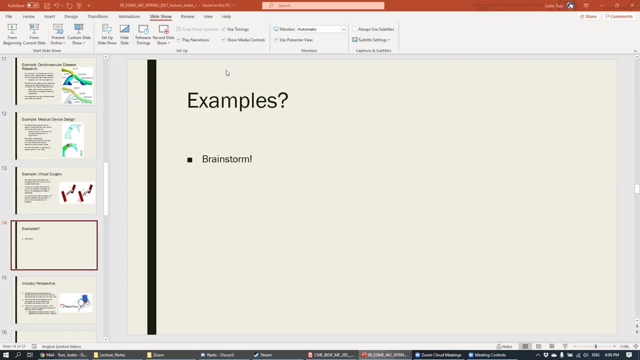 I see some questions in the chat. will i be able to perform heart surgery? no, so, uh, we might be able to simulate heart surgery. no so, uh, we might be able to simulate heart surgery. no so, uh, we might be able to simulate it, but you won't be able to conduct it because that takes many years of training. yeah, 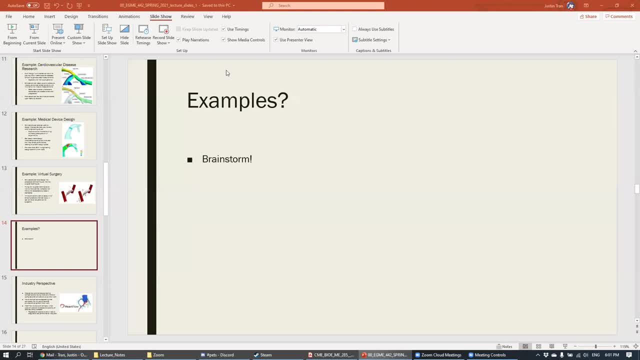 pacemakers. yeah, pacemakers a great device, so that that actually has to do more with kind of the electro, um, the electromechanical things that happens in your heart, and so we're going to be- we're going to be focusing a lot more on the fluid mechanics, but pacemakers are definitely, you know. 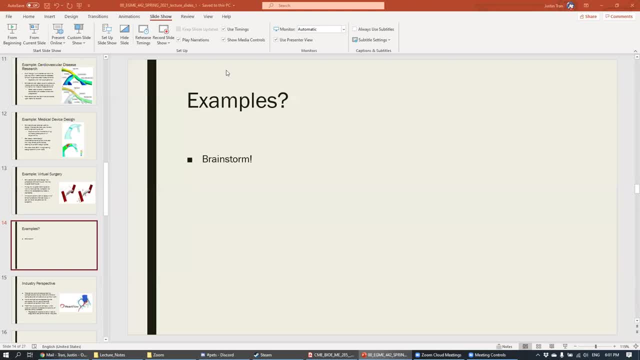 um a very common device. that's um that has to do with, kind of the electrical signals in your, in your heart, right erectile dysfunction. no, we're not, we're not going to be able to do that, but not going to go over that. catheters- yes, catheters is is a is another, um really common device too. 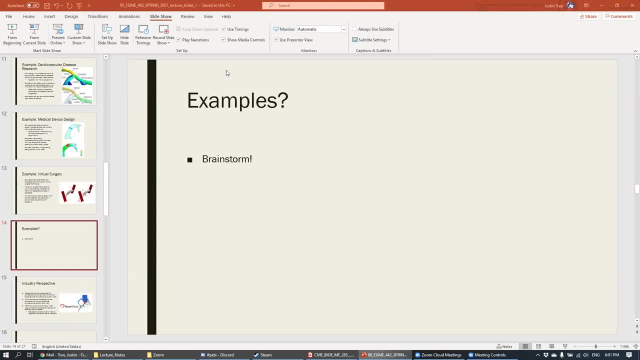 and so when i was talking about before, you know, when you insert probes into people to measure their, um, their vitals, you know a lot of times they use a catheter to do that. so, um, catheters are really interesting and i i wouldn't want to have a catheter inserted in me anytime soon. um, 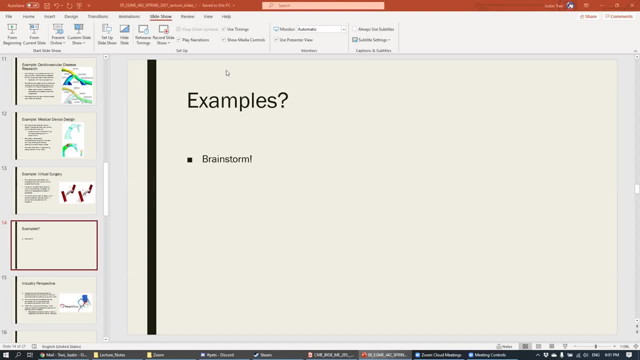 because usually, because there's only so many places in your body where you know you can insert a giant freaking wire and then have you be, um, be okay with it. so actually i've been doing a lot of very common place where catheters are inserted or is actually in your groin, and so if they, if they. 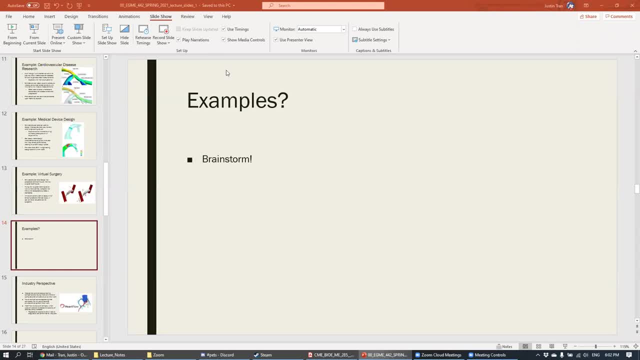 if, like, a surgeon, needs to go and measure something in your heart, they're going to stick a wire in through your groin and they're going to snake it up to your heart, and so i've seen it happen to people and like i don't feel comfortable even just watching it. so i hope that you know i've. 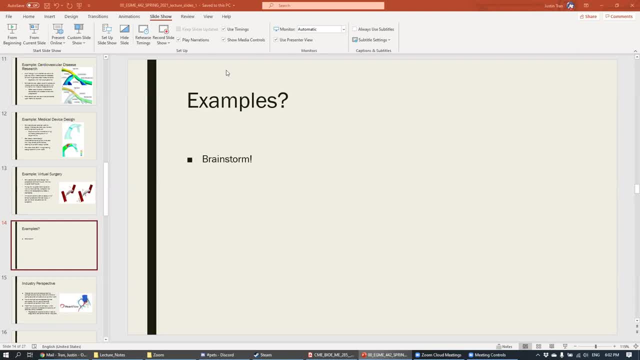 definitely been taking better care of my body ever since i've seen that happen, because i don't want that to happen to me. yeah, mitral valve prolapse: yeah, very, very big field for for cardiovascular and so valves. you know we'll talk about that more when. 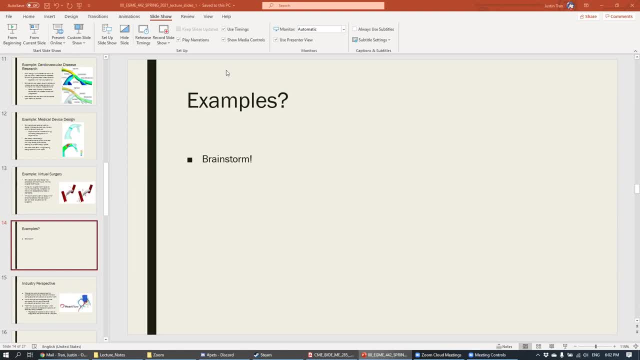 we do our anatomy. but valves are basically structures inside your heart that can basically regulate, you know, the, the direction of flow, and so people's valves get faulty all the time. so prolapse is one of those diseases where you know the valve kind of fails on itself. so 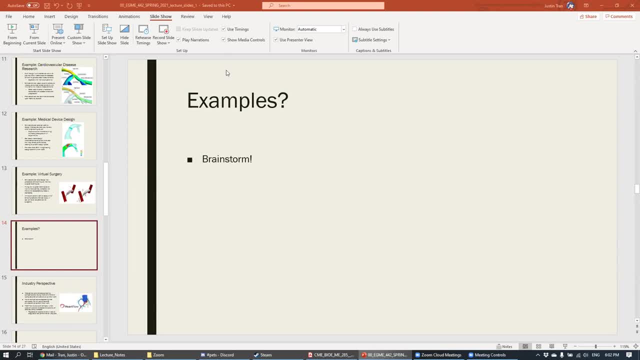 um, there's a lot of- you know- research and a lot of money into artificial valves for people. so definitely a great, a great feel right. 3d printed tissue, cardiovascular tissue- yeah, it's a really, really interesting field out there. um, i i have to say that i'm i'm not the person to 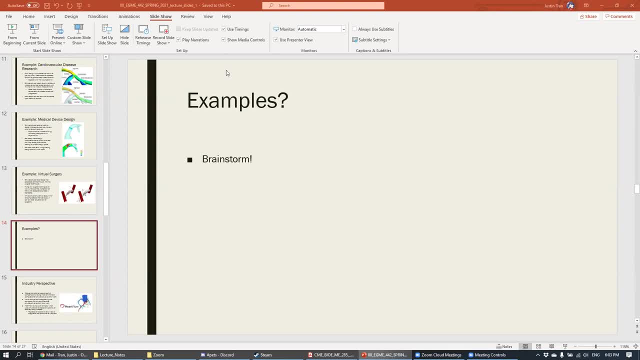 talk to for that. so actually, um, dr sue is actually an expert on on biomaterials, so i think she's teaching a class this semester on biomaterials and so she would definitely know a lot more about 3d printed tissues. but i know it's, it's a very exciting field and you know if it, if it, you know. 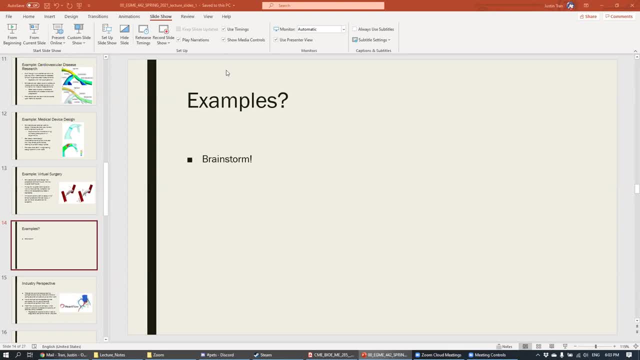 once they improve it, it's going to make a big impact on the field as well. yeah, angioplasty- yep, that's another, uh, really important um, you know, um procedure out there, typically done with catheters too. actually, yeah, balloon pumps, yeah, wow, you guys, you guys know a lot, man. i did not know nearly as much. 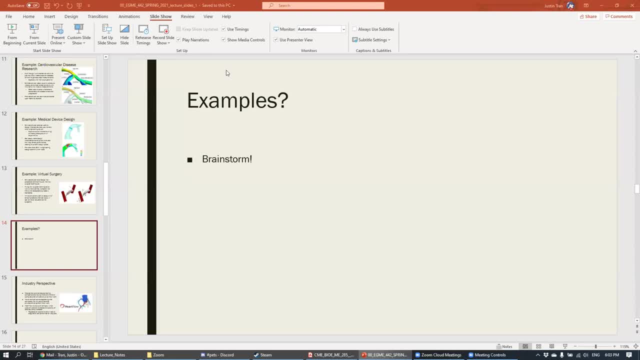 about cardiovascular stuff, as you guys, when i first started this. uh, this stuff, right, yeah. yeah, i've heard. i've heard a lot of good things about dr sue's biomaterials class. when performing a heart transplant, do you technically die for a second um for the new one to be successfully transplanted? yeah, 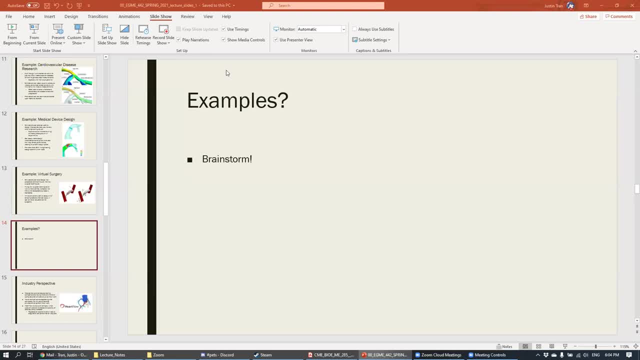 so it's. it's a complicated procedure. so actually they use a machine called a heart and lung bypass, and so they basically hook you up to a machine that's going to perform the pumping for you, you know, while they kind of swap out your heart, yeah, and so you don't, you don't die, i guess. but 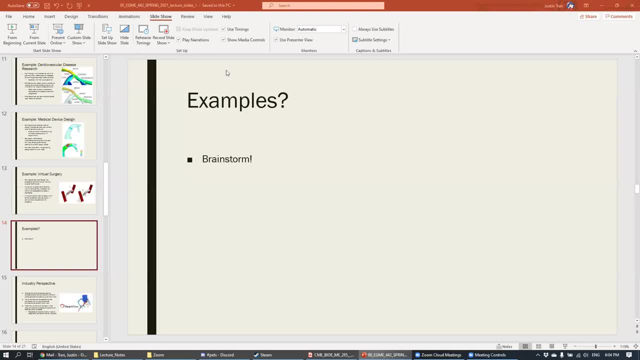 you have another machine that's going to perform the pumping for you. yeah, oh, you're kinesiology major. oh, that's awesome. yeah, got a youtube degree. yeah, let's see how will we relate, uh, computational fluid dynamics to subjects like stents and catheters. to improve, to improve designs of these medical devices? yeah, yeah, so the uh. so basically, 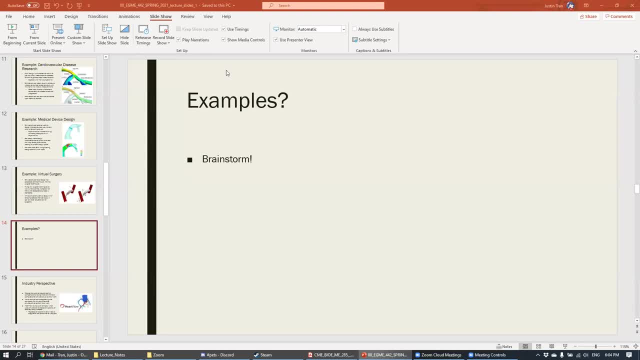 we can use simulations to simulate. you know what are like, what are the stresses and what are. you know the um, uh, what are the big impacts on these devices that the blood is going to impart. because what happens a lot with these stents is that you insert them into a person and then over time, they 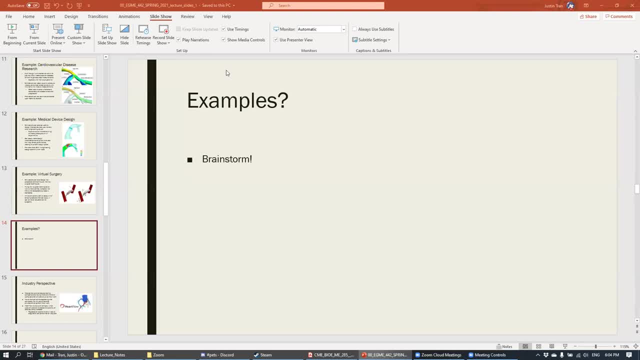 start to degrade because kind of the blood vest, the blood kind of acts on them. so i know that there's a lot of things that you can do with these stents that you insert them into a person. there's been a lot of research into, you know, simulating um the blood flowing over these stents. 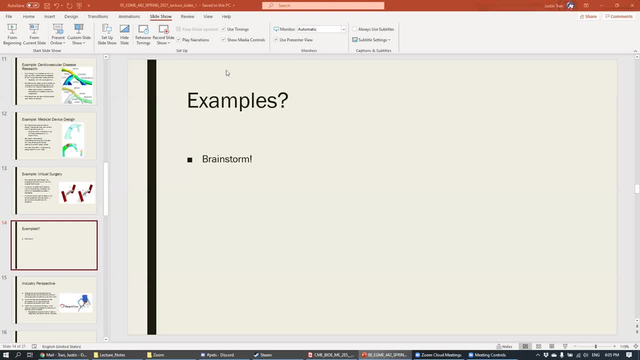 you know, to to improve their uh, to improve their efficacy. yeah, yeah, great examples, guys. i, i, i knew literally like 10 of what you guys just put in when i uh, when i first started this field. so that's, that's great. so i'm, i'm really happy to see that this field is growing. you know, not only um in the 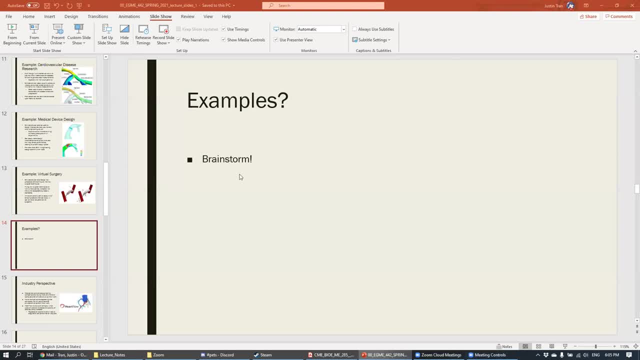 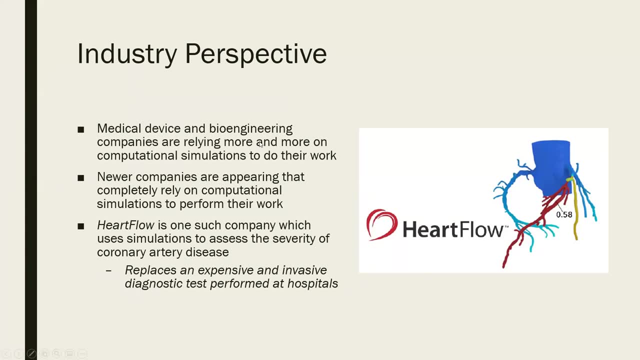 you know in the industry, but also you know from from students as well. yeah, okay. so let's go ahead and continue on, okay? so, speaking of industry, you know um. i think a fair question to ask is: you know how much is this being used um simulations in the industry? so i know before the class. you know i said a lot of the 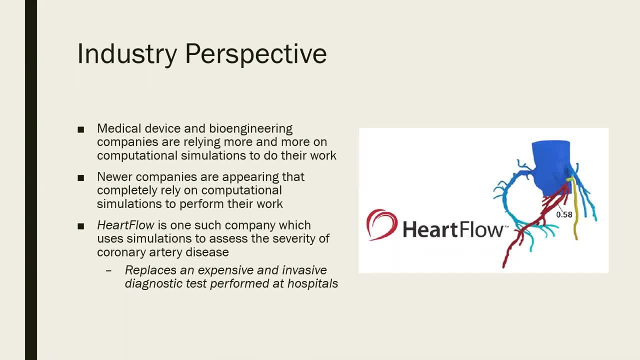 big companies out there are still kind of adopting it, but there's a lot of startups that are that are occurring, that are, you know, popping up, that are starting to use just solely simulation technology, right, and so one example that i'd like to talk about is a company called heartflow, and so, actually, 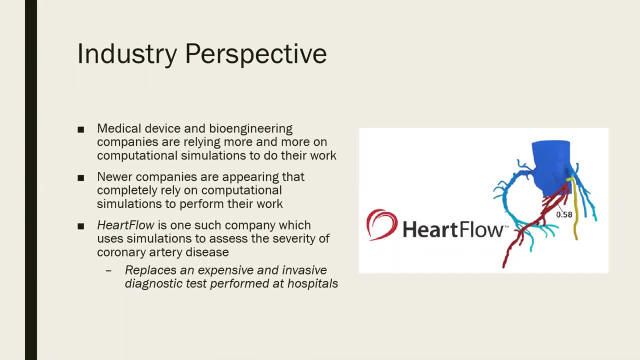 this is. this is a company that i. i know a lot of people that work there, and actually, you know, one of my good friends, one of my good buddies, is a company called heartflow, and so actually this is works there and i'm trying to get him to give a talk sometime this semester too. so 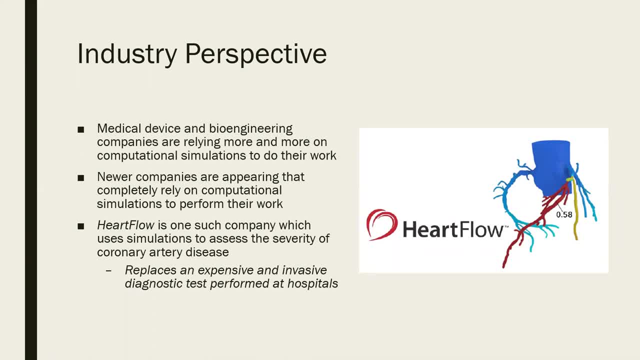 hopefully, hopefully, he's free, right. um, but what heartflow basically does is that they use simulations to basically assess. you know heart disease right, because normally you know to assess heart disease a lot of times you have to stick a catheter into someone and measure it. but heartflow- 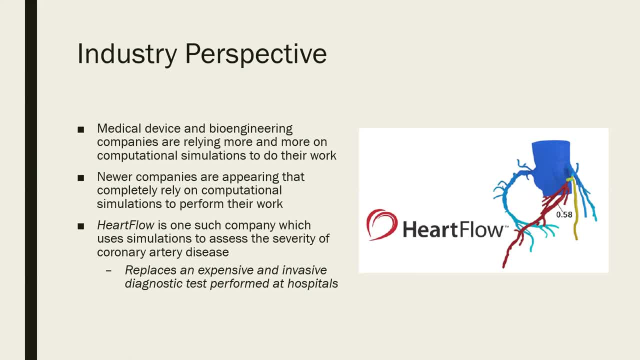 says: you know, we can do this with simulations and they've. they've been pretty successful. so they've actually seen, they've actually received fda approval for their methods and so it's really great that they're kind of the first ones to to do that. yeah, um, because what it does is it for. 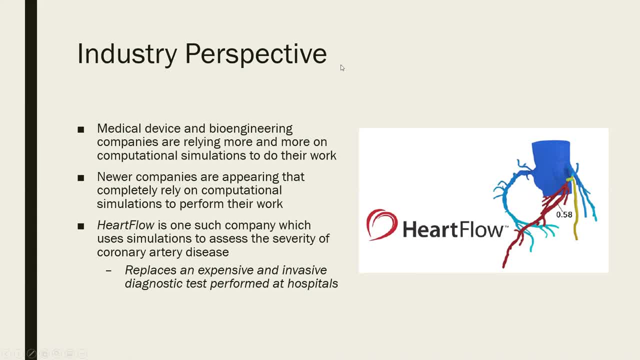 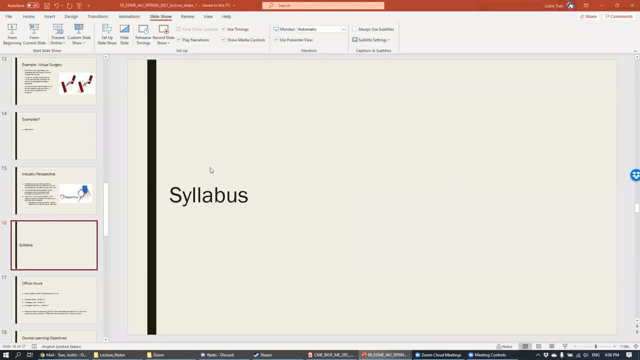 patients. it helps kind of avoid a really expensive and invasive test, um, and it kind of saves them a lot of money too. yeah, okay, uh, so any any other? any final questions on the kind of the course introduction, and so from here i was going to kind of give a tour of the of the course website. 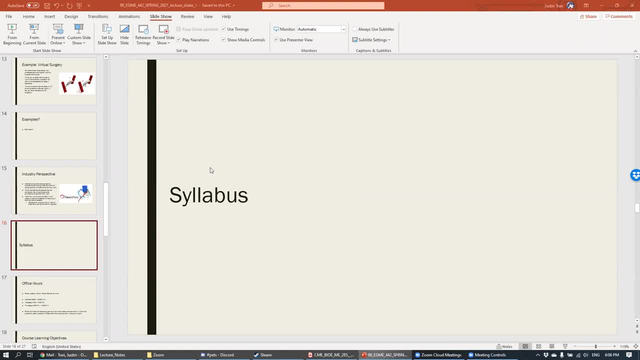 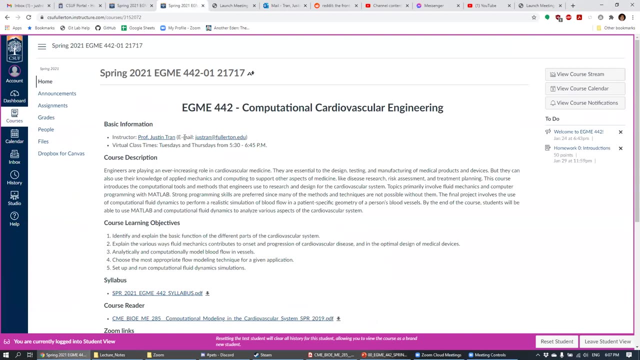 and also just talk about the syllabus. but are there just any questions about the course in in general? okay, so let's go ahead and tour the course website, not my email. okay, and so we're using canvas for our course website. so, um, you know, when you, when you first log onto canvas, this is the 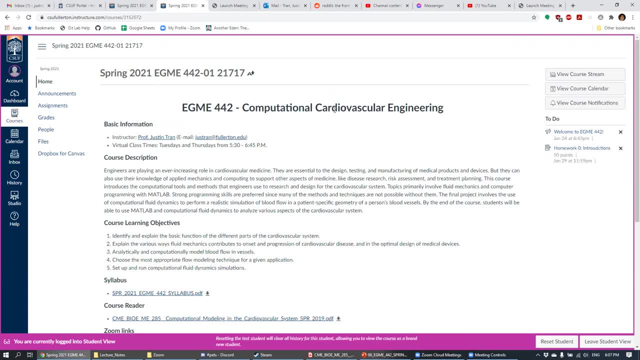 page that you'll see, okay, and so the first thing you'll see is the name of the course. so the name of the course is egme 442- computational cardiovascular engineering. okay, and then first we start with the basic information. so here's my name, right here, and, if you want to, 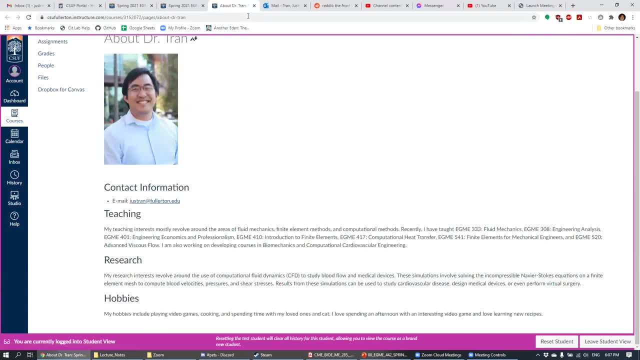 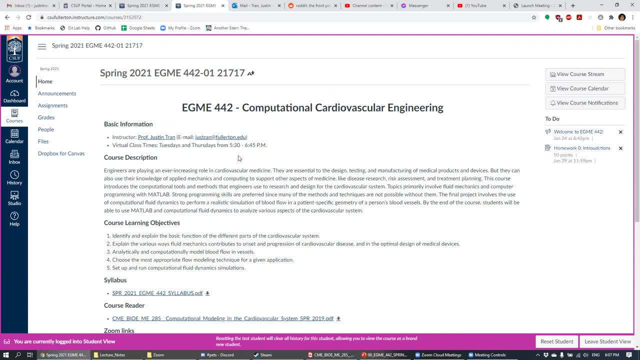 if you click this link you can come up and uh see like my tinder profile for teaching, if you really want, right, uh? and also here's my email address. so if you uh forget my email, you know it's right here on the on the front page of the uh um of the course site. okay, and next we have the. 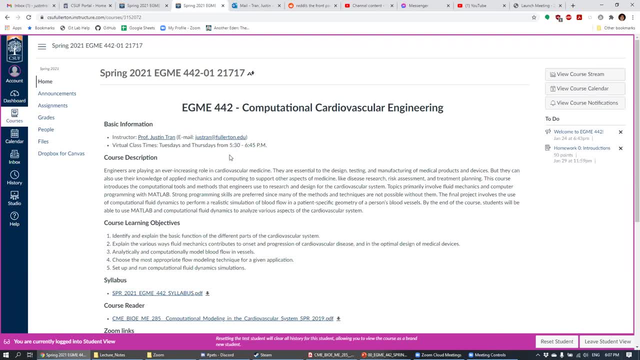 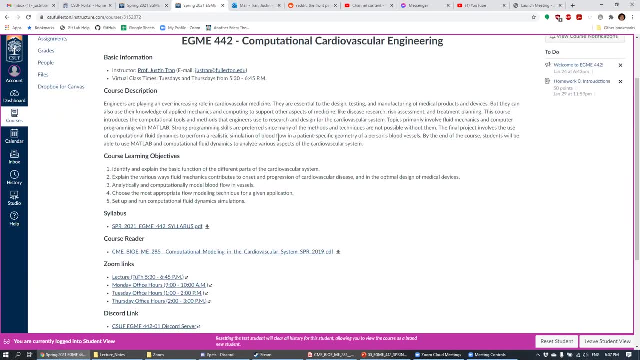 the times for the course. so you know, we're living this right now, and so this class takes place from 5: 30 to 6: 45 on tuesdays and thursdays. okay, okay, and so from here we have a description of the course. so this is kind of what i wrote to, kind of. 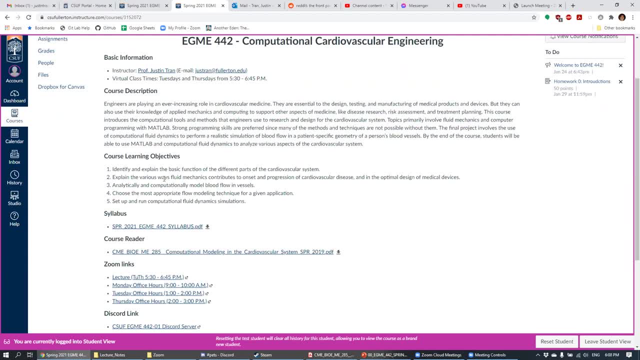 describe just the course in general, and then we have our course level learning objectives, okay, and so you know, these are the learning objectives. that are that i'm going to use to basically guide the course. so what i'm hoping for is, by the end of the course, you should be able to do everything. 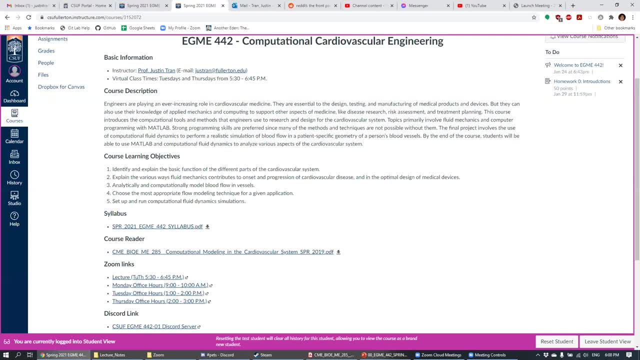 on this list right here, okay, so that's, these learning objectives are basically going to guide everything that we, that we cover. okay, tinder, it's more of a. if you read it, it's more of a tinder than a linkedin. yeah, um, but i'll leave you guys to read that. okay, uh, okay. 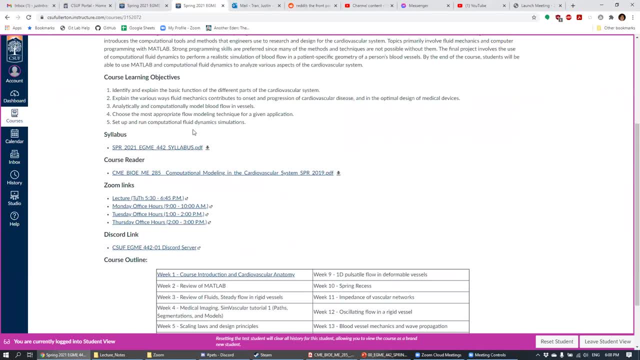 then we have the syllabus, and so if you want to download the syllabus, we're going to talk about that in a, you know, maybe in about 10 minutes, so you can go ahead and get a head start on that, okay, and so the next thing is the course reader. uh, and so you know you'll see in the syllabus that there's 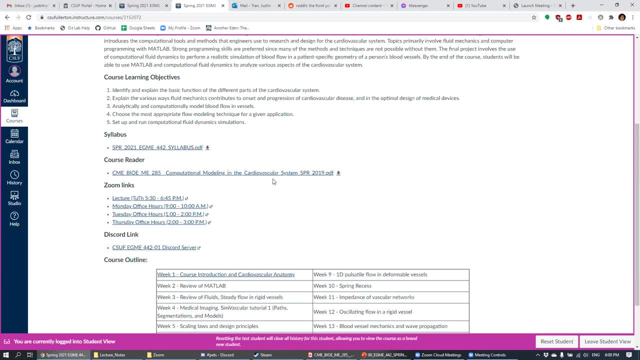 um, i'm using two references here, and so one of those is a course reader. so you can go ahead and download this, you know, and you can use that as a reference. okay, um, and so this will be like one of the, basically one of the textbooks that we're going to use for for the course. okay, um, and so. 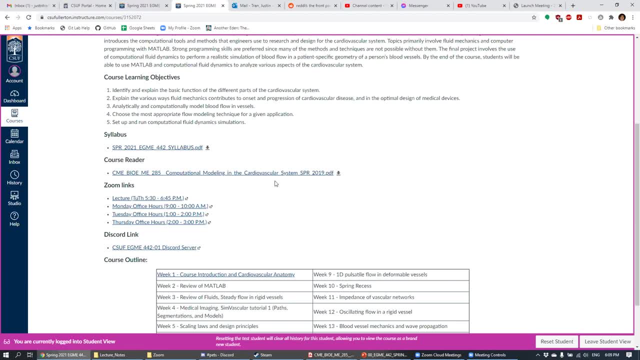 this was graciously provided to me by my old advisor, so this is basically something that she's written. um, i will say that, you know, as i'm going through it, i've been noticing a few typos in there, so i'm i've tried to correct them where. where i've seen them, you know, in my own personal lecture. 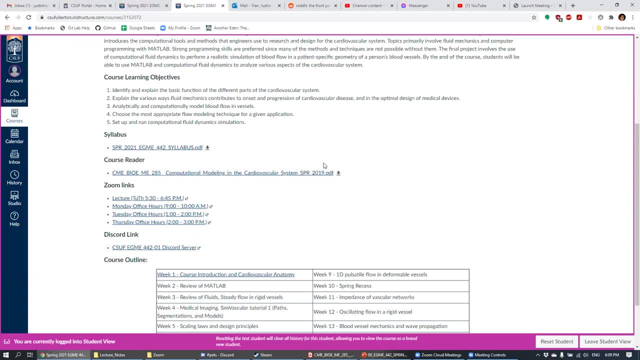 notes. but you know this is this is a really nice um reference because it's uh, you know there's not a lot of books out there that just strictly do cardiovascular computation, so this is a good resource, and then the other textbook that we have is also a good resource as well. okay, okay, then we 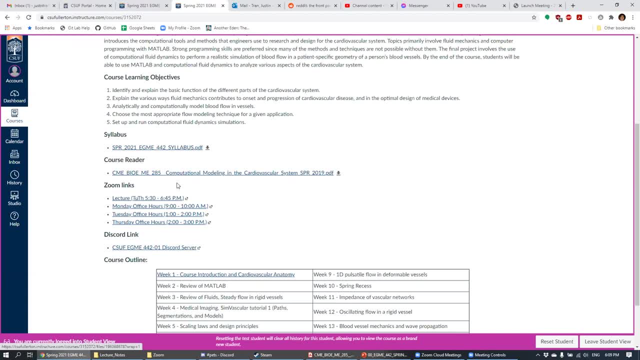 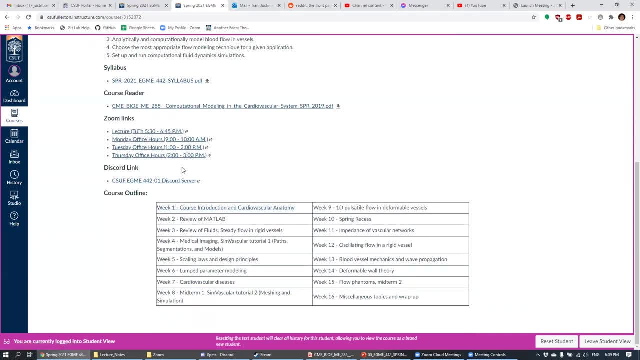 have the zoom links, and so the first is we have the zoom link for the lecture, uh, and so that's you know what we're all viewing right now, so that's, that's great, okay. then we have the zoom links for all the office hours, okay, and so i have office hours on three different days of the week, and 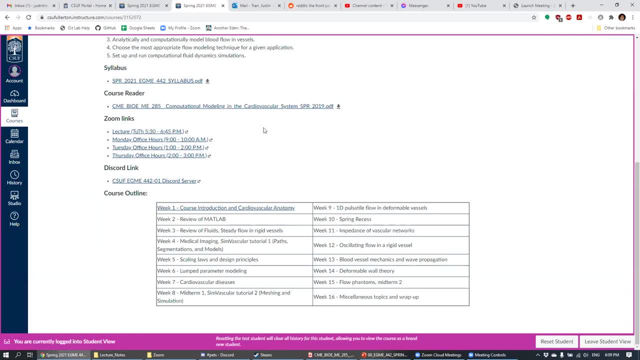 so each of them have a separate zoom link so you can go ahead and click them right here. okay, and so i, i, i try to make my office hours such that you know, i try to you know, vary their times and days so that you know, hopefully everyone has a chance to to get um, to um, get a chance to come to office. 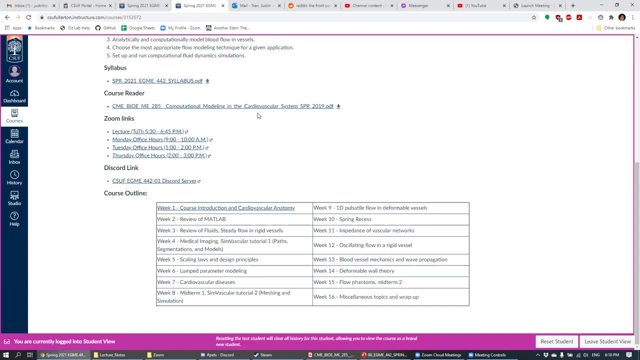 hours because i know that you guys are really busy with with other classes and with work and things like that, so i try to vary them to try to make sure that you know everyone has a chance to to come to office hours. but, with that said, i know that these aren't perfect and i know that there's 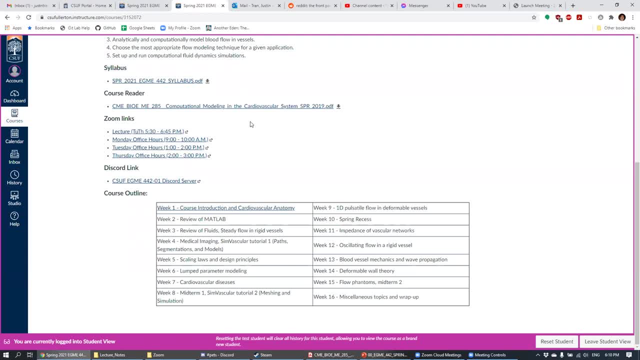 people out there who wouldn't be able, won't be able to make these at all, and so if you uh, you know, if you can't make any of these office hours, you know, please, you know, if you wanted to uh and you want to talk to me about something, just let me know, just send me an email or shoot me a message. 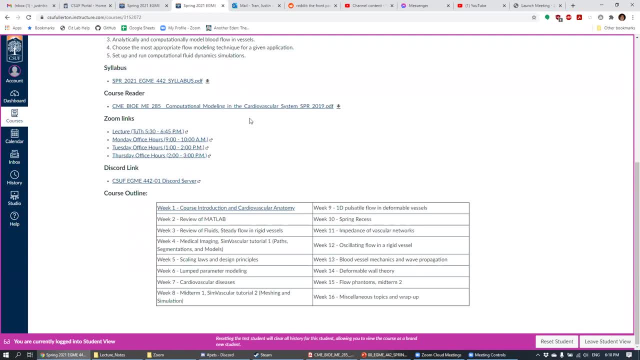 on discord and i'm always happy to kind of make you know a private appointment or, you know, uh open up a zoom room for you to uh to discuss, uh, discuss things. but but these are the, these are the hours that i'll be available. um, you know, for for, um, just for office hours, um, but again, you know if, if you, 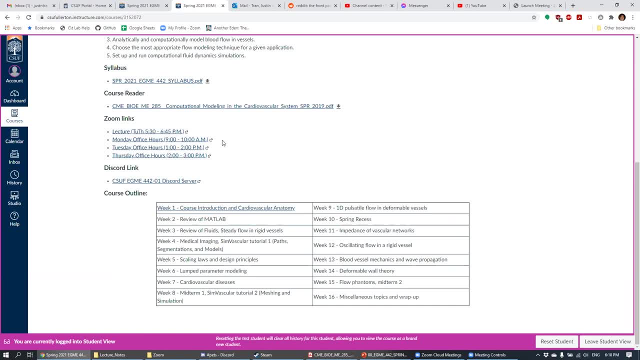 can't make these times or what, what tends to happen most often. if it's the day before the homework's due, then, and you want to, you want to get some help, just just shoot me an email, just send me discord um message and i'm happy to arrange something for you. okay, uh, okay, and so. 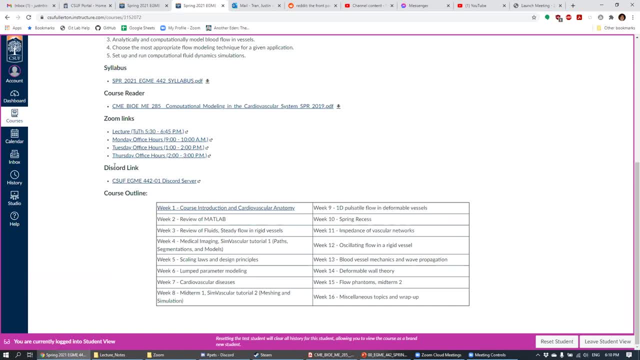 the next thing i want to talk about is the discord server, and so we have a discord server for our class, and so, because this class is taking place, uh, virtually, you know there's no way for us to kind of meet physically, because, you know, one thing that's nice about having the, the physical classroom, is that you know you can meet people. 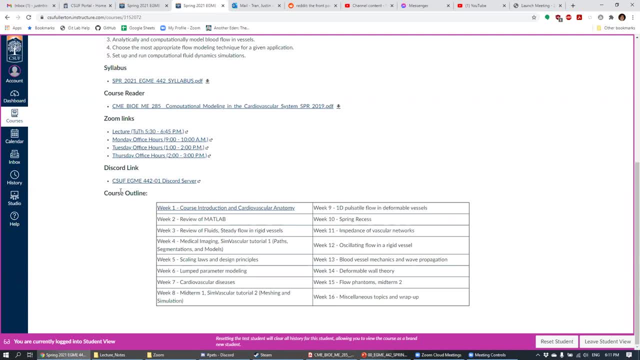 there you can kind of discuss things. you know, we can talk, you know, amongst ourselves, but you know, obviously we can't have that. and so to kind of recreate that, um, that same feeling or the same, the same interactions, i've created this discord server for us, okay. so if you go and click this, 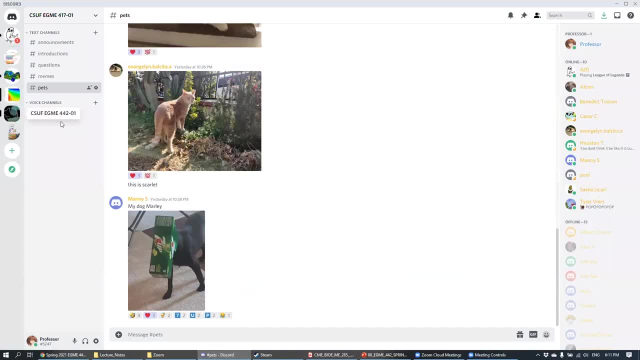 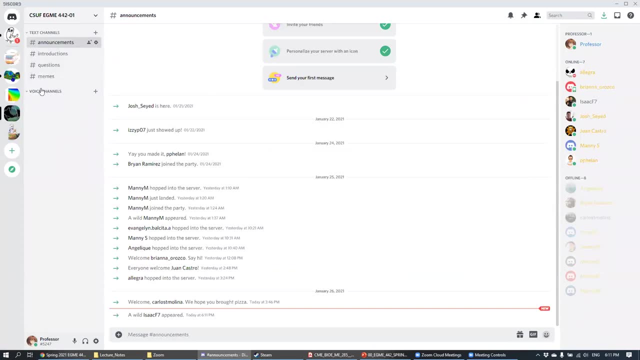 link. if you have a discord account, it'll take you to, um, you know this, um, this page right here, uh, and this is our discord server. okay, and so i have four different channels here, and so the first channel here is for announcements, and so anything you know that i want to announce to the class, i'll you know, i'll put it here. 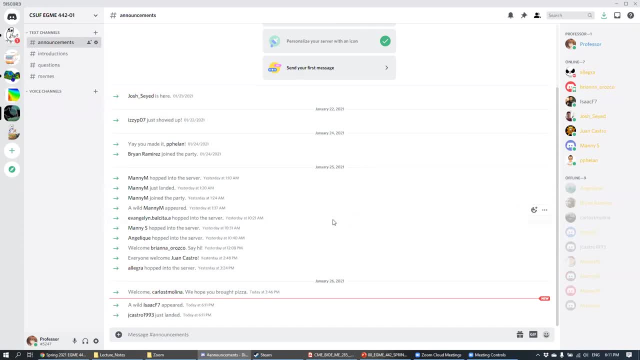 um, but you don't have to come here for announcements. so any announcement i'm going to, you know, send through um canvas so it'll email you. but you know, if there's something quick, you know that i want to uh mention to you guys. i can, um, i can use this for that, okay. 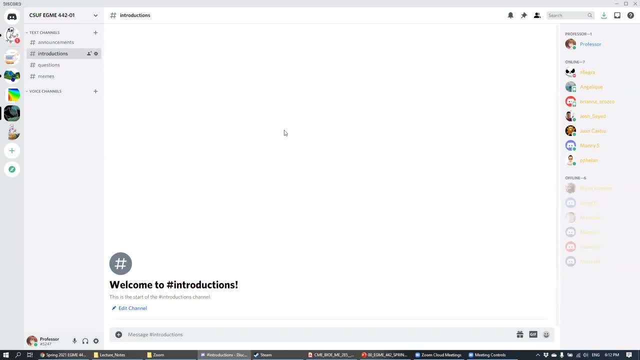 uh, the next channel is introductions. so you know, uh, this is for you guys to kind of introduce um yourselves to each other, right and so if you want to, you know, meet other people in the class. you can just leave a quick message. so just say: you know um your name and you know just something. 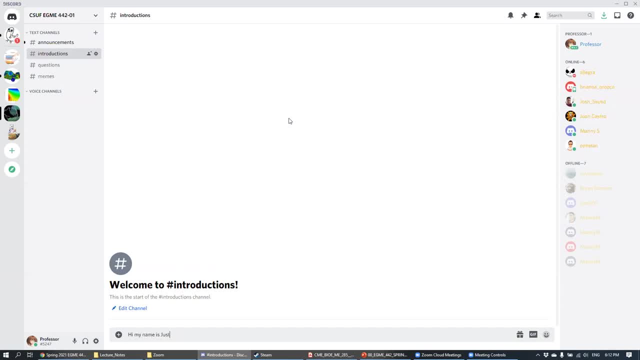 interesting about you. so say: hi, my name is justin and i love my cat. okay, um, so just maybe your name and something interesting like that, just so, just so other people in the class can kind of get to know you. okay, okay, and so, uh. next is the questions um channel, so i imagine this one's going to be the most active. 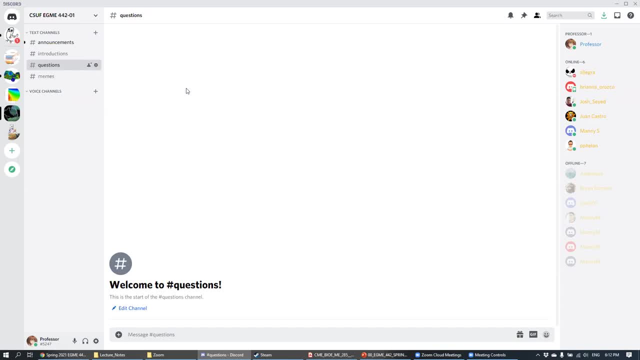 throughout the semester, and so this is where you can ask questions about you know, maybe something you're stuck on a homework assignment, um problem, or you know you're having trouble debugging something in your in your software. right, this is where you can go and ask questions, okay, and then? 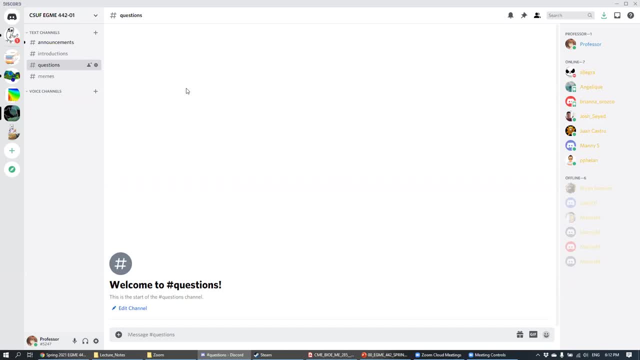 when questions are posted here, you know, definitely feel free to answer each other's questions, because it's, you know, that's that's kind of what the- uh, the discord server is for. it's for you guys to help each other, okay, uh, so i will say that, um, you know, because i have four different classes. you can see, dickbutt's not one of the. 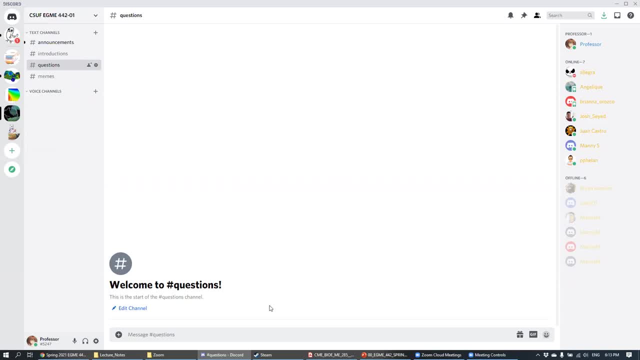 classes. i think that's one of someone messaged me um, you know it can be a lot sometimes to uh, um, they're constantly getting notifications, so i've turned off notifications on this channel. but if you would like to summon me um and ask me a question, all you have to do is just tag me. so 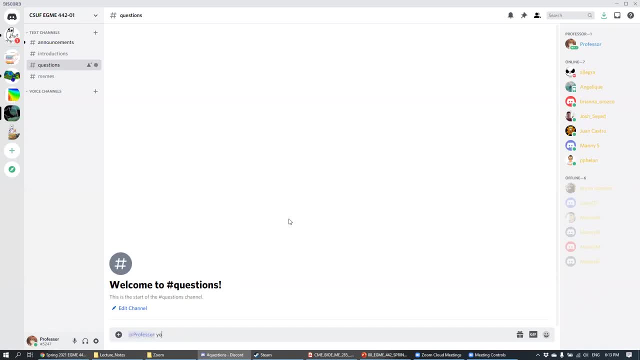 just do at professor and just say: yo need help here, please, okay. and then, once you do that, it'll send me a notification and i'll be able to answer your question, and i'll be able to answer your question and then i will appear in the discord server. i will answer your question and then i will. 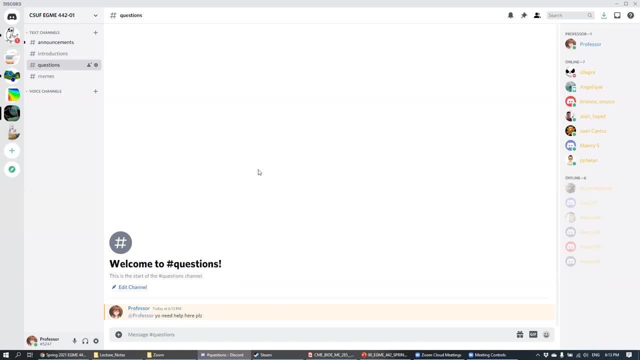 leave after that. okay, um, but mostly, you know, i want this, this discord server, to be for you guys, so that you can kind of interact with each other and help each other out, because that's you know, that's, that's, you know, a big part of the uh educational process. okay, okay, and then finally, 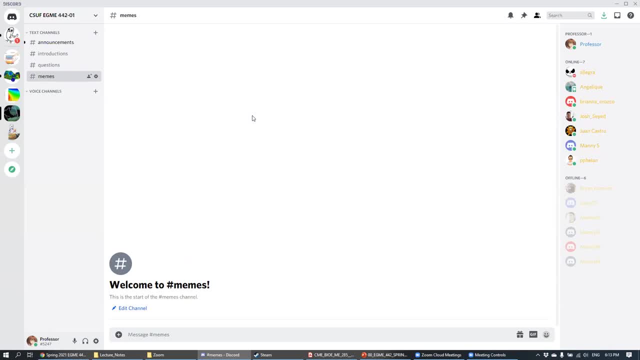 i have just- i just have a channel for memes. so you know any kind of you know memes that you want to share, um, you want to make fun of of me or things like that, or you know um, share some jokes. this is kind of the place for that. so this is the discord server and i'll be able to answer your questions. 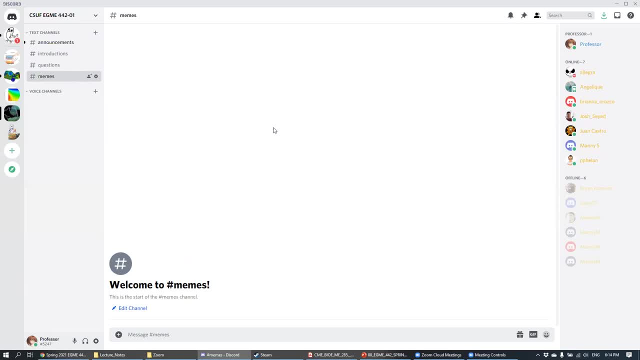 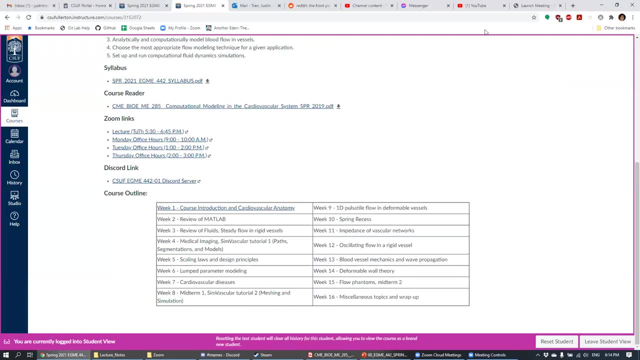 this is kind of just for: you know fun things, so i call it memes. but you know anything, anything fun you want to share, um, you can put here too, okay, uh, so are there any questions so far on the course website or uh, um, or the, or the discord server? 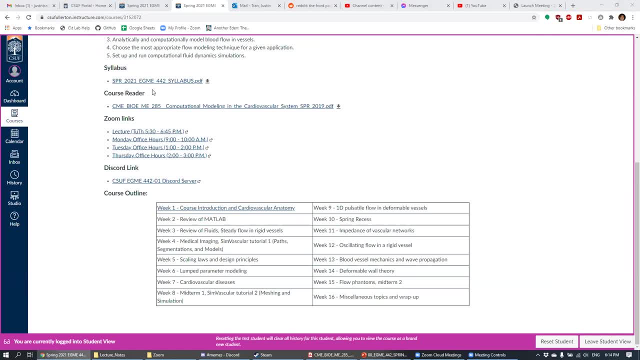 okay, okay, and so let's let's come back to the course website, and then let's come to the bottom of the home page and let's go to the course website, and let's go to the course website and right here, and then here we have our course outline, okay, and so you can see, here i've broken. 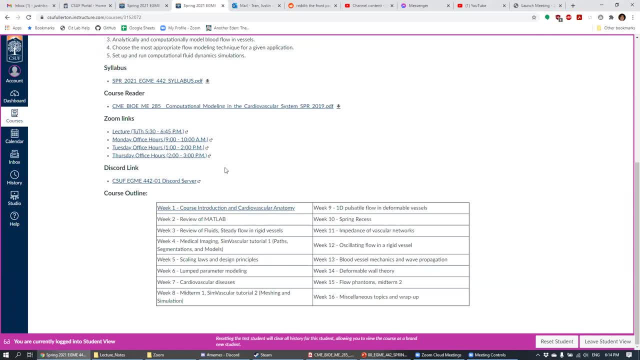 down our semester here into all 16 weeks, okay, um, and then what's going to happen here is that as we progress through the semester, these links will become active and you can click them. okay, and so we're in week one, so we go ahead and click week one right here, okay? 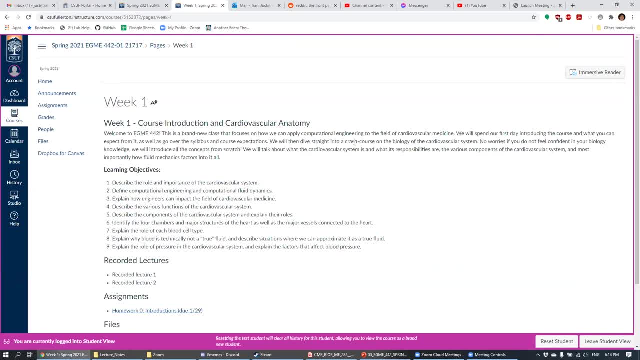 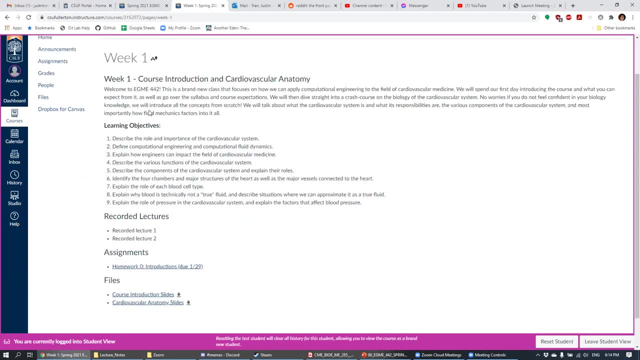 and then, once you come to this page, you know, um, you know, it'll tell you some information, all the information you need to know for that week. okay, and so, since this is the first week, um, this is all that i have. but every every week is, uh, going to have basically the same format, okay, and so every 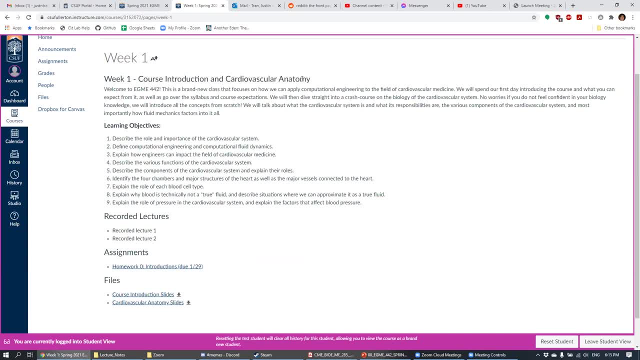 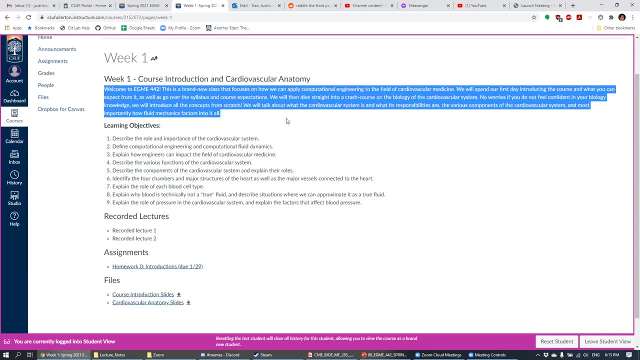 week is going to start with its title, okay, and so this week is going to be course introduction and cardiovascular anatomy, which is what we're going to do on thursday, and then from there i've written kind of a short blurb, um, or a short paragraph about you know, describing what we're. 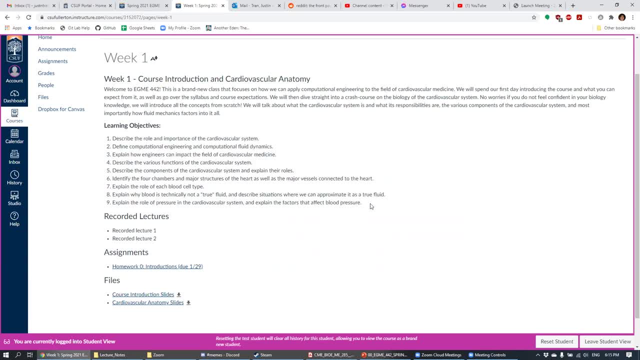 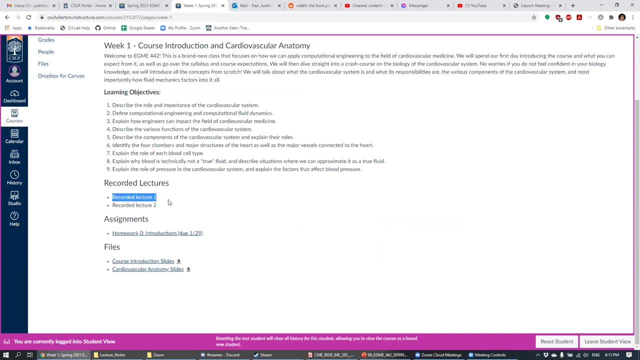 going to learn this week and i've also listed all the learning objectives for this week as well. okay, um, and then also on these pages, i'm going to um put the youtube links for the recorded lectures. um, because, you know, after every lecture, basically i take the video file and i upload it to youtube. 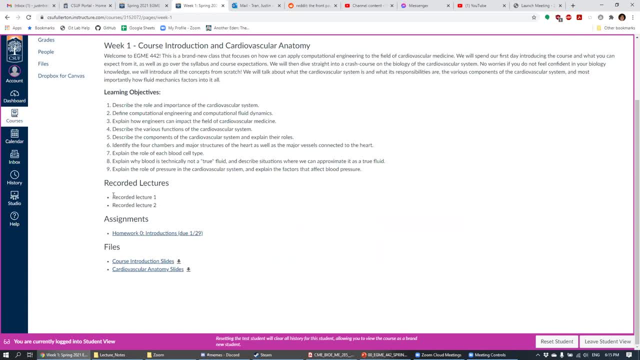 and then once that, once youtube is done processing that, then i put the links for it right here so you can- basically this is easy access for you to um- view all the lecture videos. okay, and so i have a slot for lecture one and lecture two. okay, um, any homework assignments that i've assigned that week. 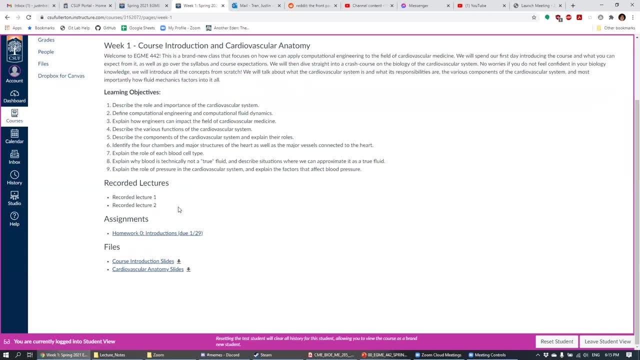 will be put here as well, okay, and so right now, there's only one homework assignment, um, and that's for the introductions, okay, and so we'll talk about this later today, um, and then any files that i want to share with you guys will be here as well, okay, and so any. 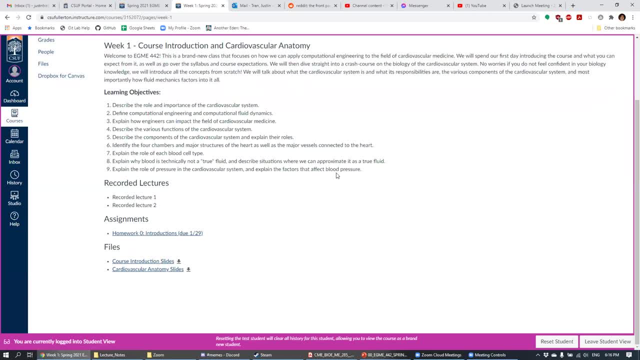 lecture slides, any lecture notes, um any homework assignments, um any homework solutions, um study guides, extra material, basically any, any material that i produce for this class. you know i'm going to upload onto the onto the course website and you can find them, you know, within the files for for. 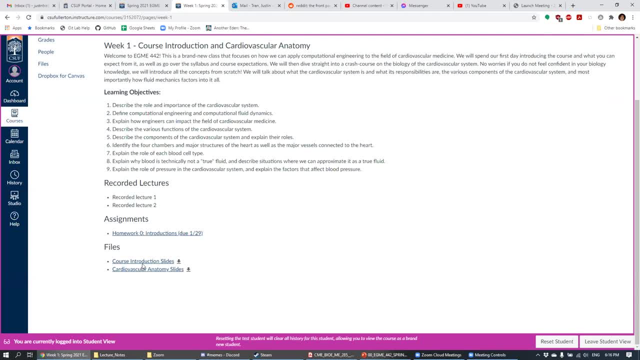 that week, okay, and so at the very least you know each week you can expect the lecture slides or lecture notes for that week to be posted. um, at least you know the friday before the the week, okay, and then just any other files that you can you can find here as well, okay, 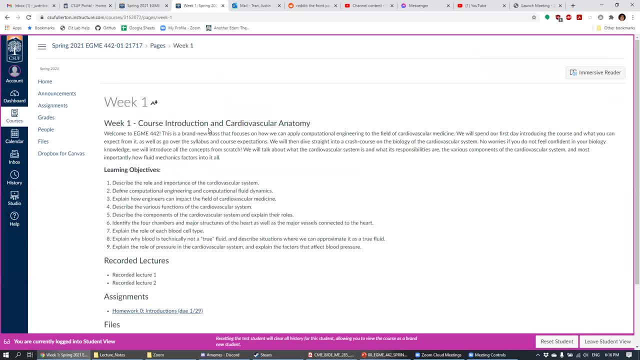 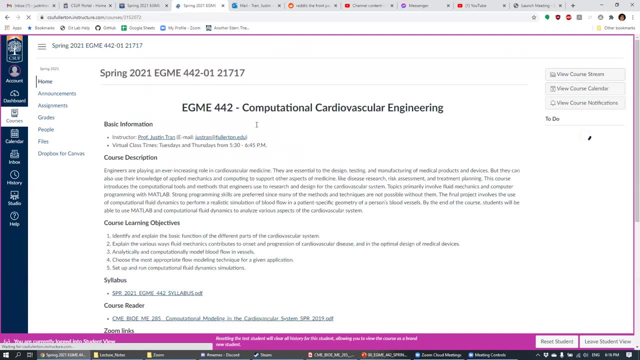 and so you should, you should definitely be visiting these weekly. you know these um weekly um pages a lot, because this is where i post. you know a lot of the information, okay, okay, and so that's the weekly viewer. okay, and so that's everything you need to know on the home page. 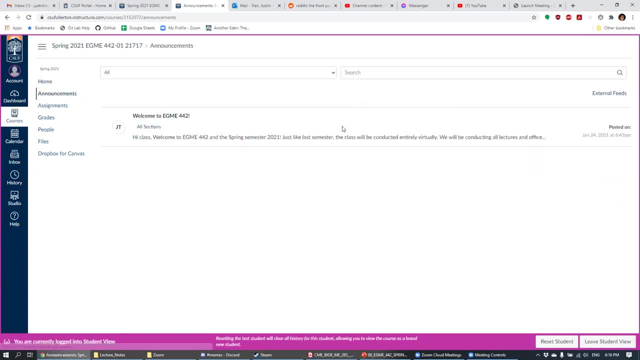 so let's go through all the different tabs now, and so the first tab is the announcements tab. so, um, probably you'll never have to come here, because this just lists all the announcements that i sent throughout the the semester, because whenever i make a post here on the announcements, it sends you an email. 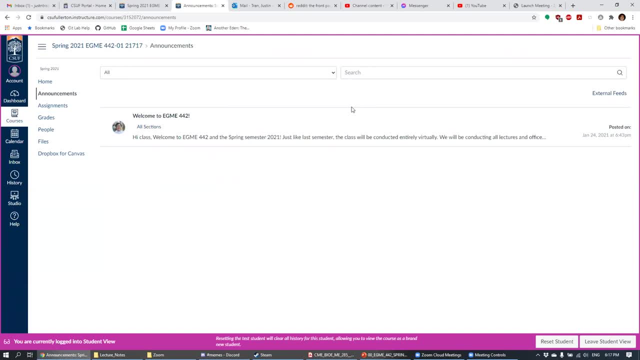 automatically, but for some reason, if you want to view kind of a list of the announcements, you can come here and do that. okay, uh, next we have the assignments tab, and so anytime i assign an assignment- um, you know, i create a homework or create, you know exam, you know it'll- it'll show up here. so this: 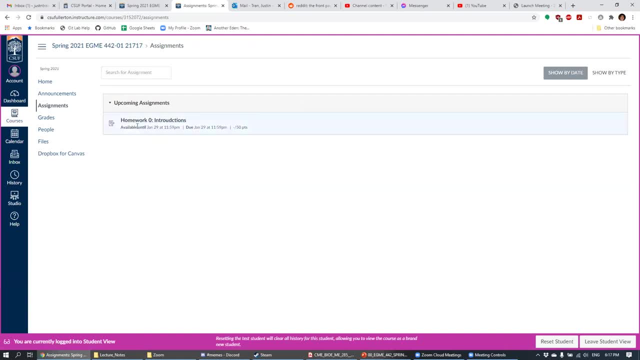 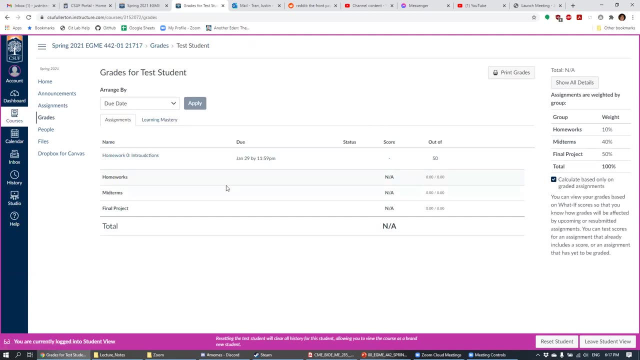 is just a simple list for you and you can see here you know, when it's when the assignment is due, how many years of absentia or if we're not doing a whole semester of intercourse or an extra year of points is worth, and when it's available from Okay. Next we have the grades tab, And so when 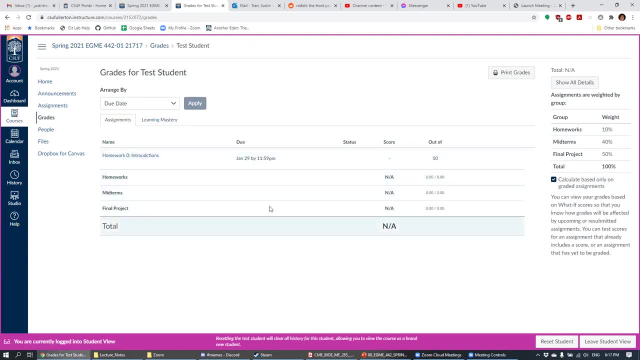 you come here, you can view, you know, basically, your grades for every assignment, Okay, And then once you, once I've entered some grades, it'll, you know, have a total for you here, And then what it's showing you here is also how the grades break down. So you know for this class. 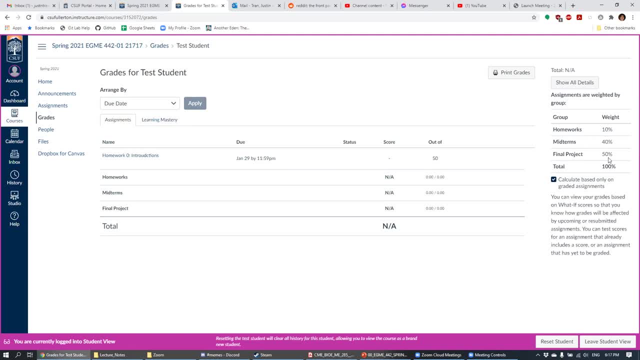 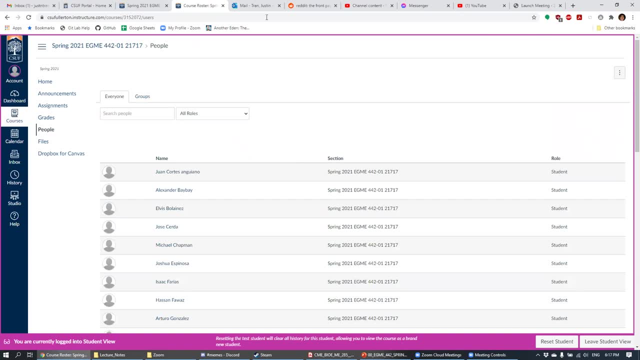 homework should be worth 10%, Midterms are going to be 40% and final project will be 50%, Okay, Okay. Next, we have the people's tab, And so if you want to see a list of everyone in the class, 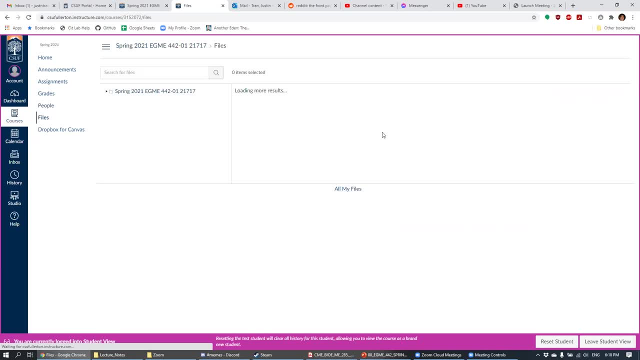 you can do that here. Okay, All right. And then the last tab that I'm going to show is the files tab. So this is kind of kind of the raw, kind of file folder, that where I'm going to upload everything. So, and so you know, every everything that I upload here I'll put a link toward to. 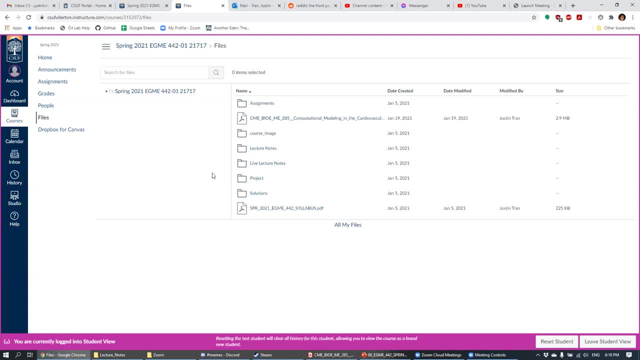 you know somewhere else in the course, usually in the weekly viewer. But you know, if you want to come here and say you know what, what tends to happen often is that you know I sign a homework assignment and I make, I make a mistake in the solutions And so sometimes I'll update. 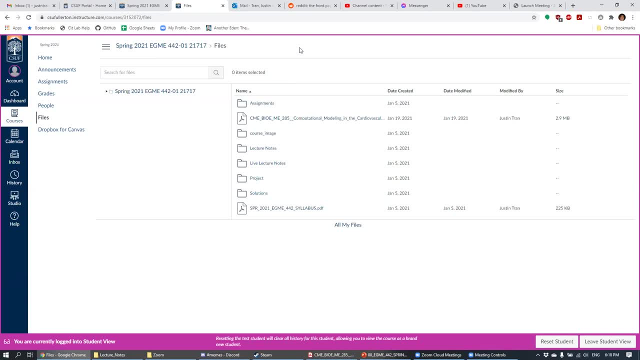 those, And so if you want to come here and just download the updated, you know, homework assignment, you can just come here and do that, Okay, And so I have a folder here for assignments And so basically all the homework assignments will be here. So it's empty right now. Okay, This lecture. 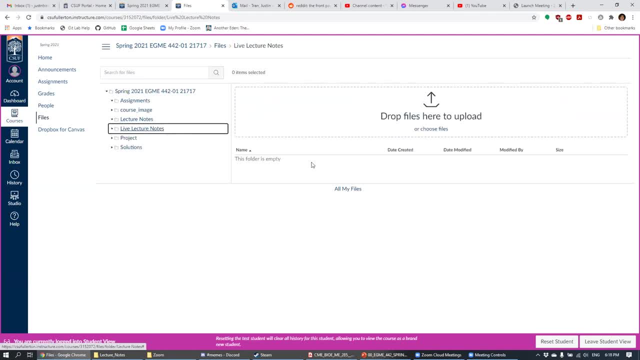 notes folder will contain all of the lecture notes. Then I have the live lecture notes, And so, basically, what this folder will do is it's going to show you all the assignments that you have, And usually when I, when I lecture, I like to write notes on my iPad, And so you know I turn those. 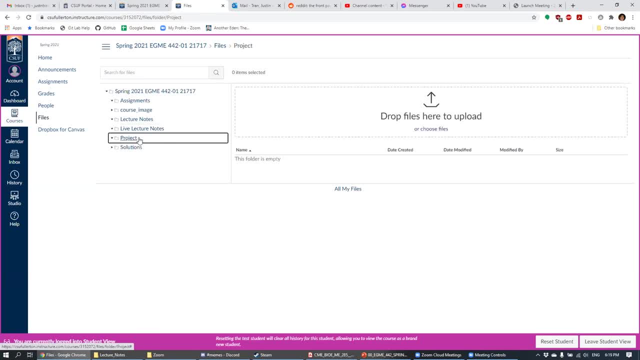 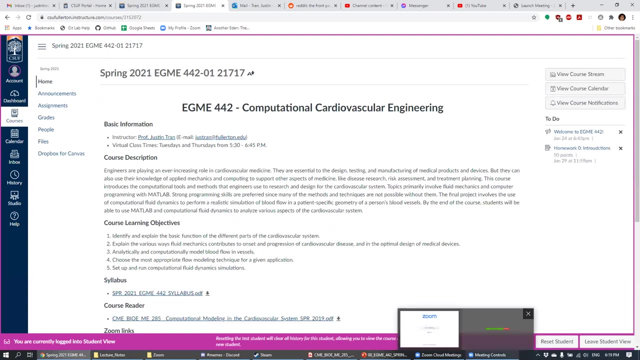 notes into a PDF and I upload that here. Okay, I have another folder for projects, So any, everything that has to do with the project will be here, Okay, And then any solutions, I'll put it in this folder right here too. Okay, Okay, And so that's everything in the course website. So are there? 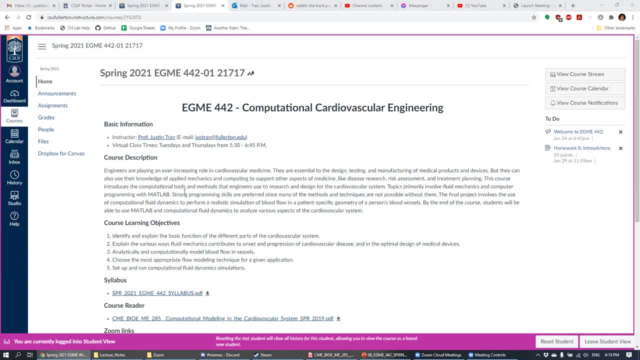 any questions before we we start talking about the syllabus. Question: Is this a tech elective course? Yes, this is a tech elective And so, since it's a new course, I think it's it's. I think Dr Weiss told me it's. it's not like officially approved yet. 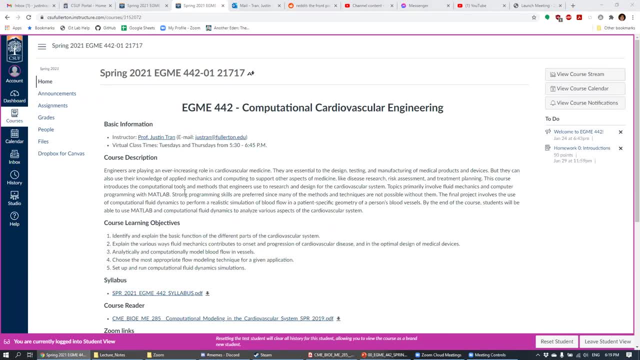 but it's, it's, it's going to be approved for a tech elective. So yeah, So you don't have to worry about that. Yeah, It's not approved yet, but it's, it's. it's basically in the pipeline, It's just. 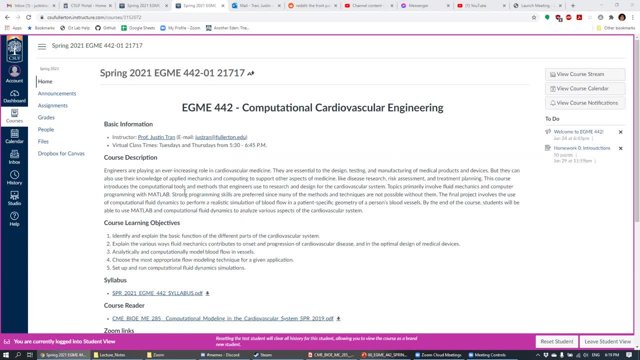 waiting for some signatures. basically, Yeah, Yes, You will get credit for it. Yeah, We'll it will. it will count towards your degree Question. So how much would I be referencing the textbook that is on file separate from the file? 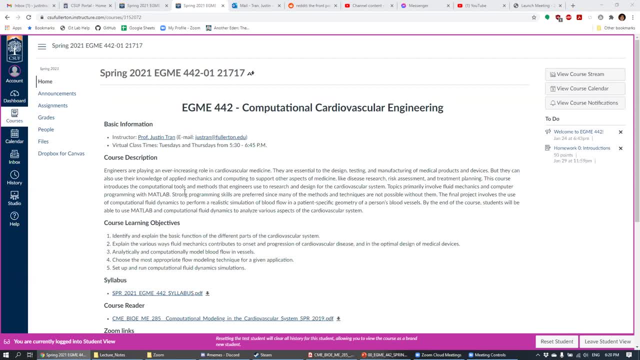 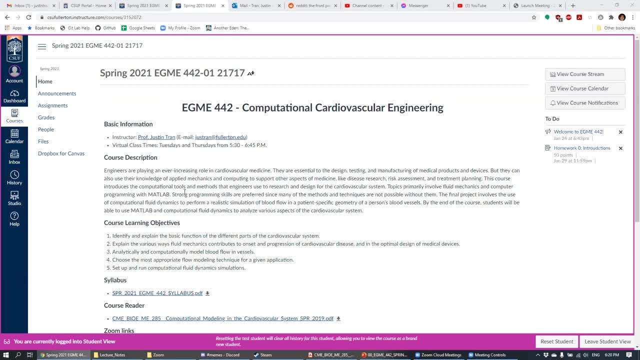 bottom of the syllabus. you know I have both textbooks that are covered there. So for each week, basically I've listed basically the, the chapters in each textbook that I'm going to. that that people cover Yeah, And so you can kind of refer to that, that file or that table there, Yeah, 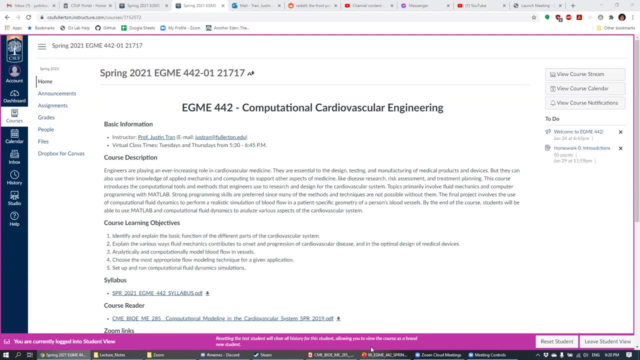 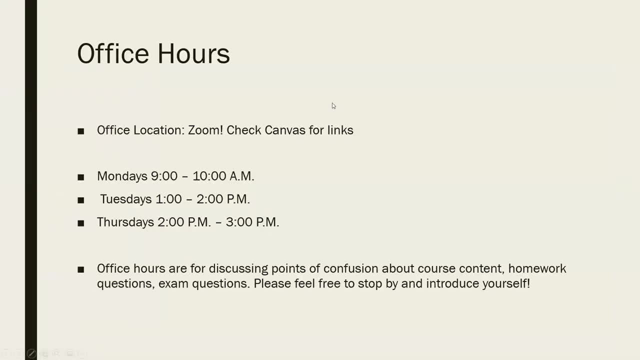 Okay, So there's no more questions. Let's go ahead and start talking about the syllabus. Okay, All right, So the syllabus. so office hours. So we, we already talked about this, And so the office hours will take place on Zoom. And here's all the times for the office hours. Okay, And so office hours. typically, what they're used for is, you know, discussing any points of confusion. So, if you know, if you were confused about anything we went over in the lecture, or if you have questions on the homework assignment or the, or you know we want some clarification on the exam grading, then you can come and talk about that here. That's typically what they're used for, Okay. 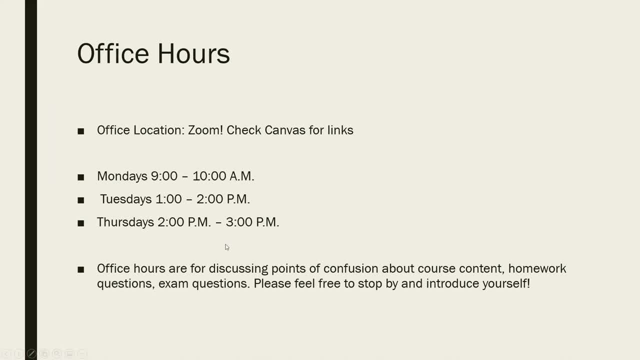 But you know, if you just want to stop by and just say hi, you know, that's, that's, that's great too. Sometimes office hours can be kind of lonely if no one shows up. So you know, that's, I'm always, always makes me happy for when people show up, Okay. 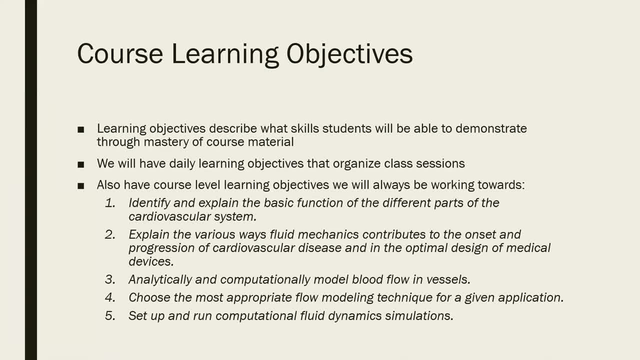 Okay, And so here we have our course level learning objectives again. So again, you know, we've, we've seen, we saw this in on the course website. But you know, I basically use these learning objectives here to design, you know, the entire course. Okay, 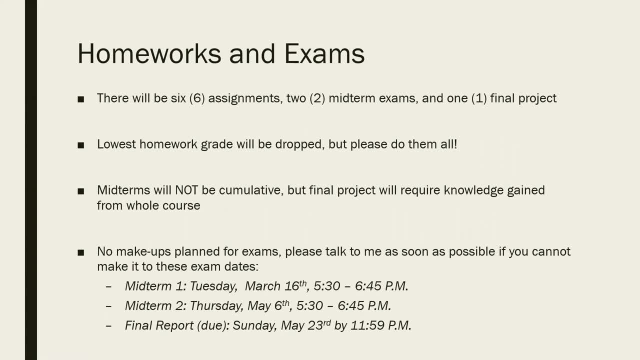 Okay, So let's talk homeworks and exams. So right now, I have six homework assignments that are planned, two midterm exams and one final project. Okay, And so, out of those six homework assignments, whatever your lowest grade is, I'm going to drop it. 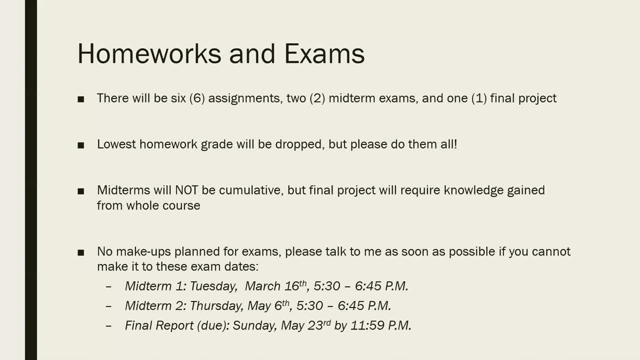 Just because I know it's, you know it's. it's always a busy semester, So you know, I want to give you guys the flexibility so you don't have to be, you know, absolutely perfect on the homework assignments. 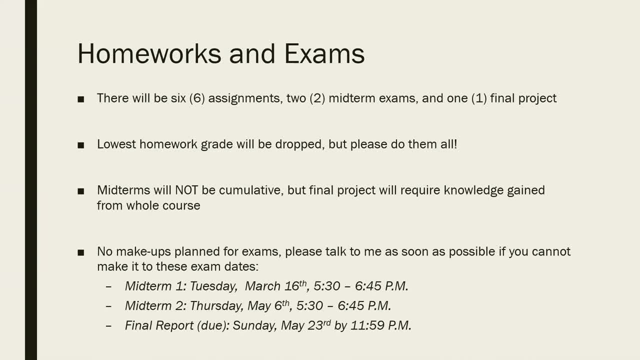 And so one other thing that I forgot to mention here is that, because this is a tech elective and you know, generally for tech electives, you guys are here kind of because you want to be. it's not because we're forcing you, And so I'm only going to grade the homeworks for completion, Okay. 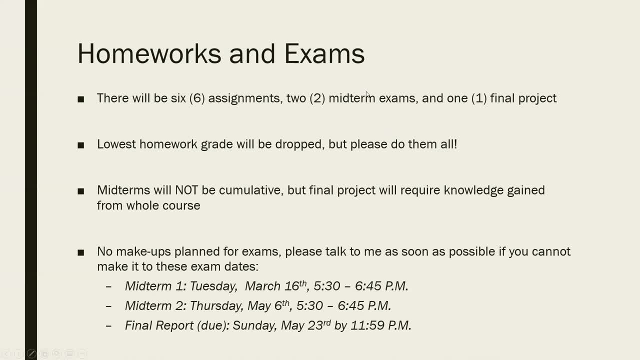 And so I'm not going to be giving you that much feedback on your homework assignments, So and so, when I finished grading the homeworks, you know, and I posted solutions, you know it's going to be up to you guys to to look at the solutions to you know, to find out. you know what you did, you know if you did anything wrong and you know how to learn from that. Okay, 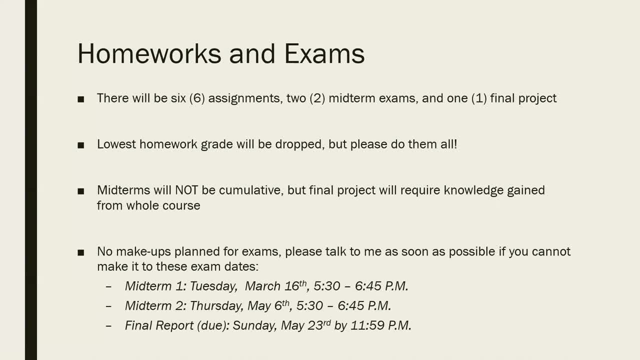 And so you know that's going to be on you guys to do, to do that, Okay, Okay. So the midterms they're not going to be cumulative, So the midterms are just going to be just for kind of one chunk of the class for about like about six, seven weeks worth of content each for the midterms. 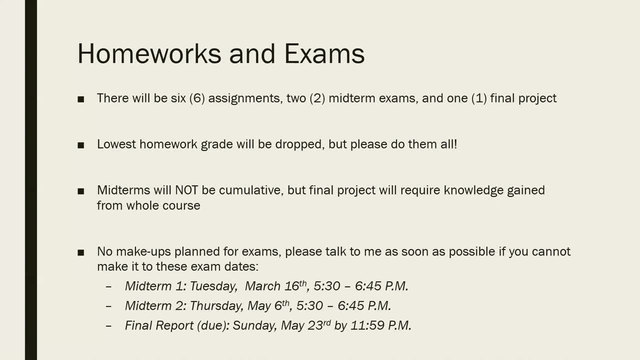 But the final project. it will require you to have knowledge throughout the entire semester. So you know, don't forget anything. you know you're going to use everything throughout the whole semester, So make sure you keep it all all there, Okay. 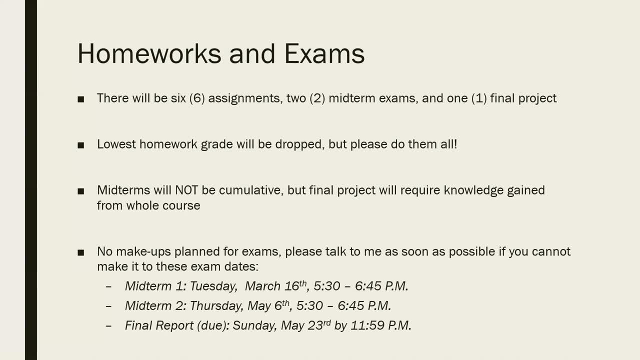 And so here are the dates that we have planned for the exams, And so the first exam will be in March. The second exam will be pretty close to the end of the class, Just because, just because that's just how kind of the content kind of rolls out, And so that'll be in May. 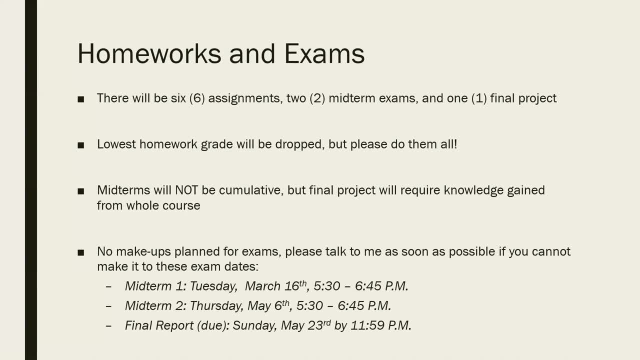 And then the final project. And so, since we're not going to have a final exam, you know we have the final project that's going to be due on Sunday, May 23.. Okay, And so I want- and I want to address this too, because you know, last semester what I did for the exams was I did 24 hour exams, which I really liked, but I also had a lot of instances of academic dishonesty. So in order to kind of curb back on that, you know, I've 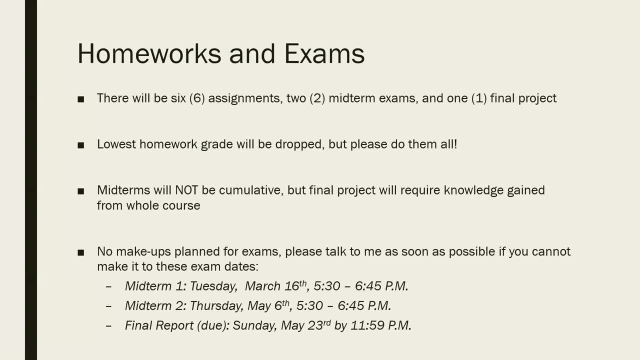 I've decided to make my exams timed and in class Okay, And so what I'm going to do is I'm going to make the exams shorter than I usually make them, Because I know some people last semester told me they spent like eight hours on the exam. So you know they're they're going to be a lot shorter, just so that you can finish them within the time period and also scan and upload them. 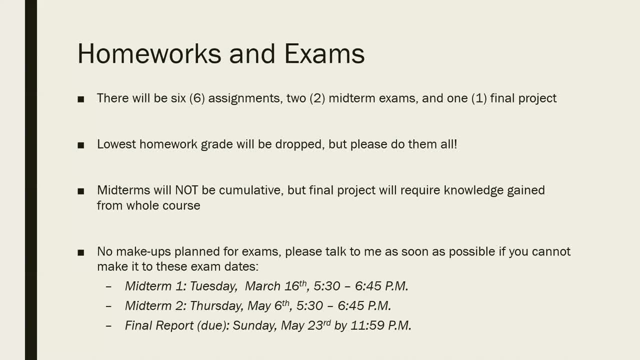 But they will take place during just the lecture period. So make sure, make sure you're available on on those days. Okay, And then the due date for the final project, that's going to be the- that's going to be the Sunday after the exam. 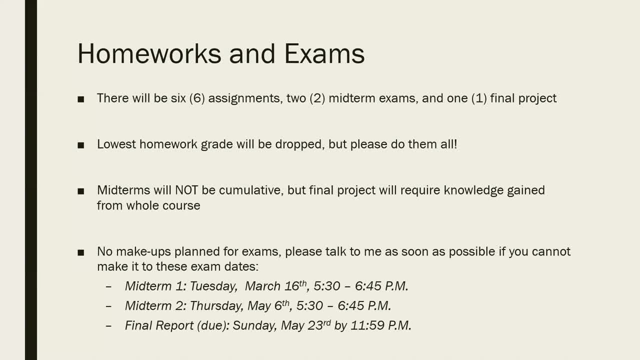 Okay, Okay. And then the due date for the fall semester finals week, because I know spring semester finals week is always really busy for for you guys, especially for the seniors. I know you guys have seniors, a lot of senior design stuff, you have graduation stuff, So you know I want to give you guys some extra flexibility for that so that you can turn it in. you know, hopefully after all those things are done, but soon enough so that I can actually grade them and not get in trouble by by the department. Okay, 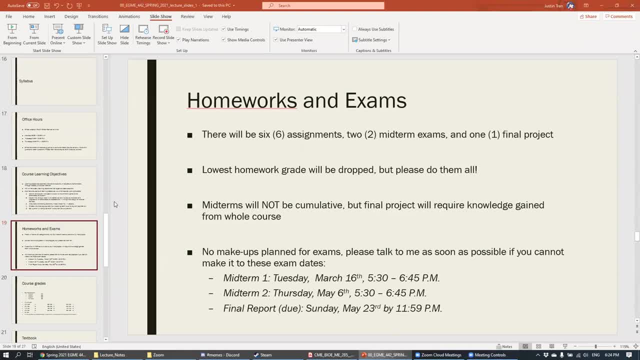 Okay, Are there any questions on on this? so far? Okay, So you. So you will need to buy the other book. That's what we'll talk about in a minute when we go to the textbook. Great, Yeah, we'll talk about that soon. So only six homeworks total. Yes, only six homeworks. no final, so no final exam. No, this is only going to be a final project. final project will be individual and that is non negotiable. So the final project you will do on your own. 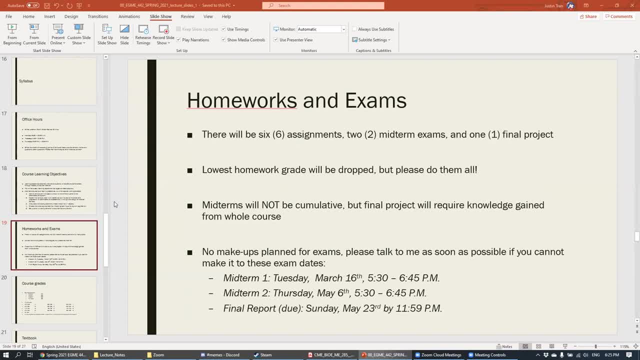 You know there will be no groups for the final project, So you will need to buy the other books. So you will need to buy the other books. Yeah, homework usually takes a while. Yeah, so I'm gonna be six assignments, but they will be six significant assignments. Yes, 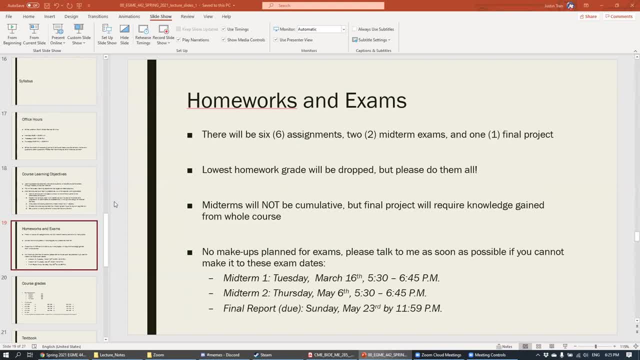 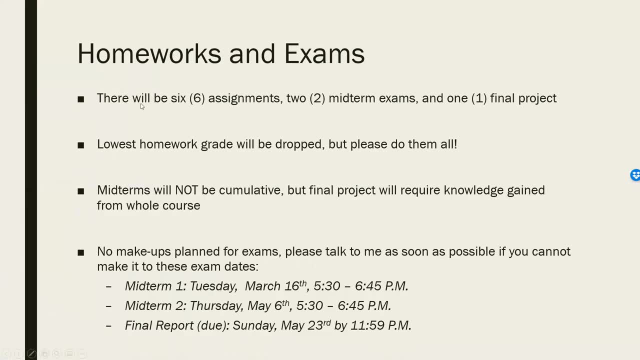 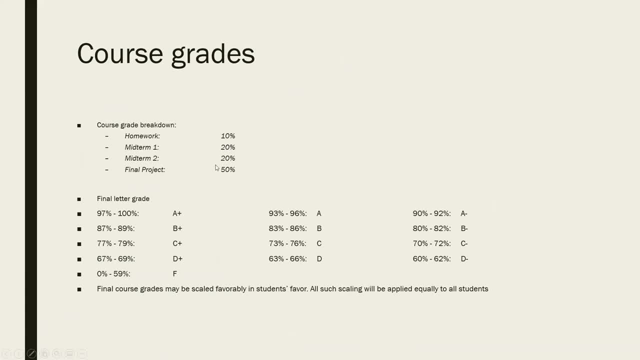 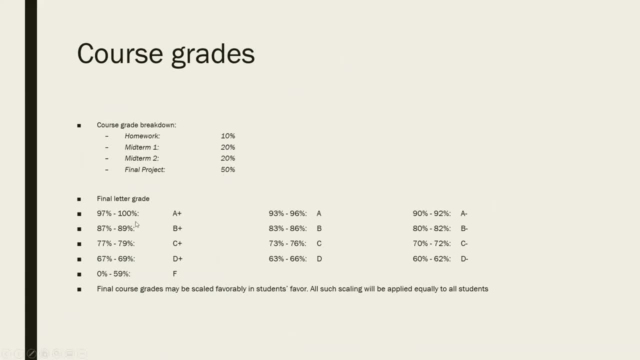 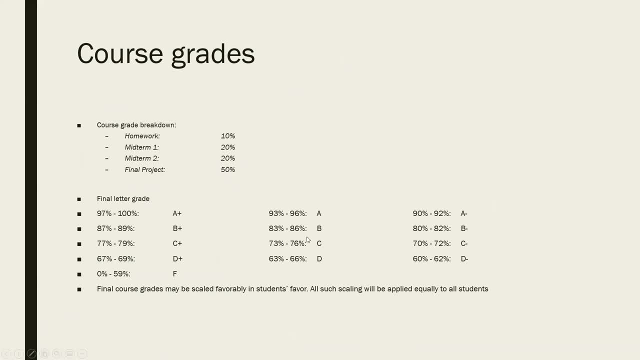 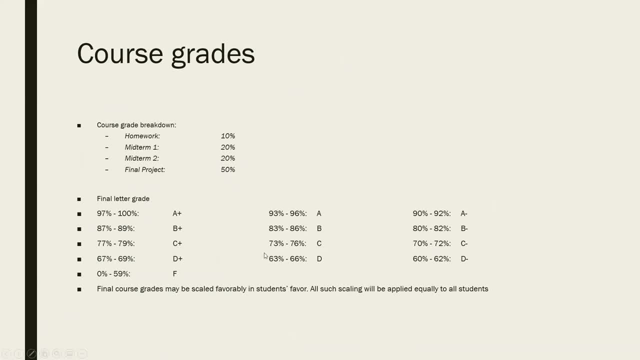 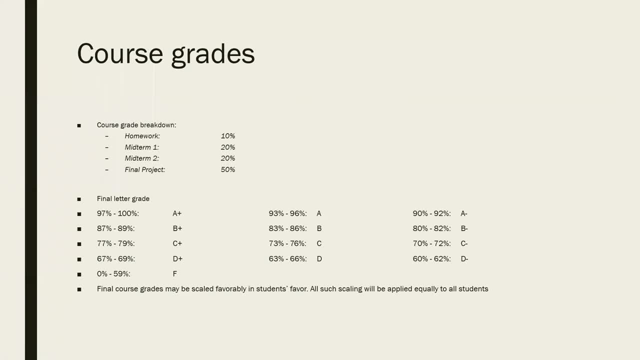 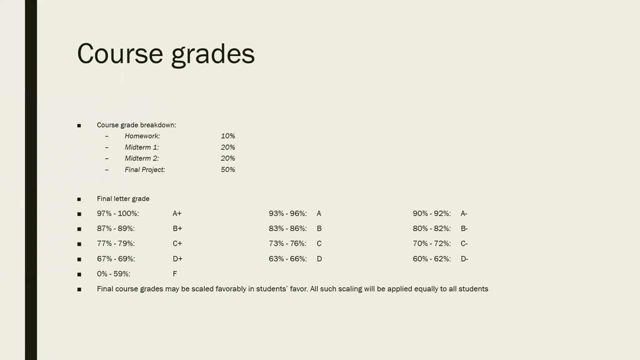 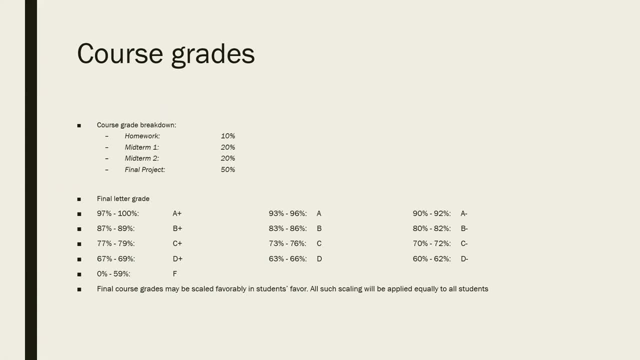 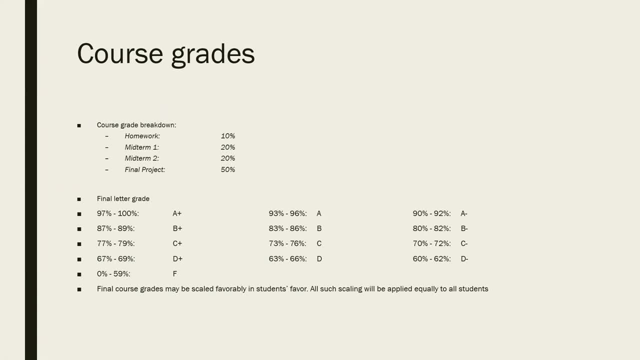 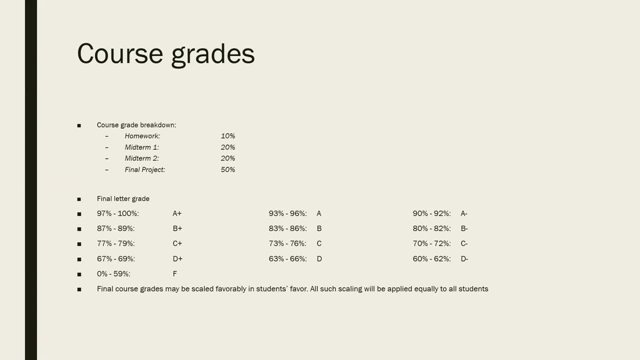 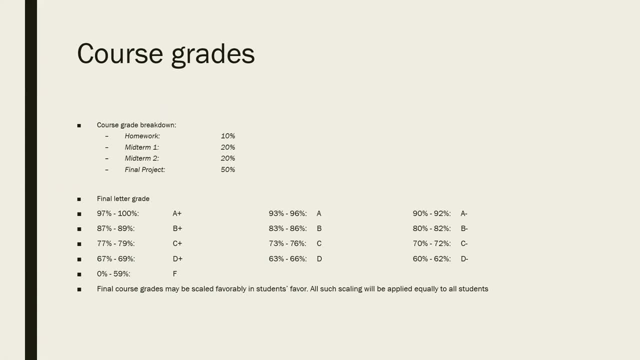 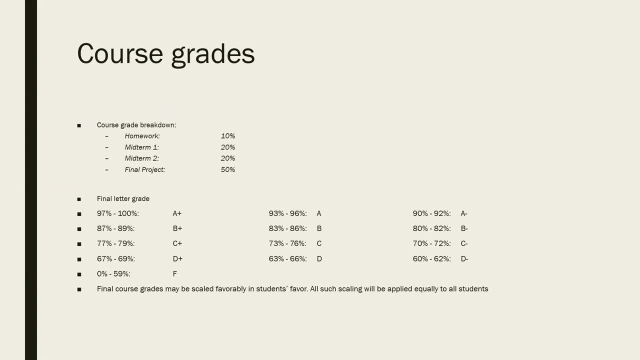 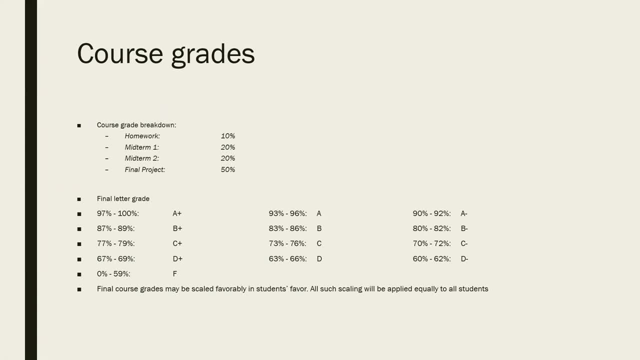 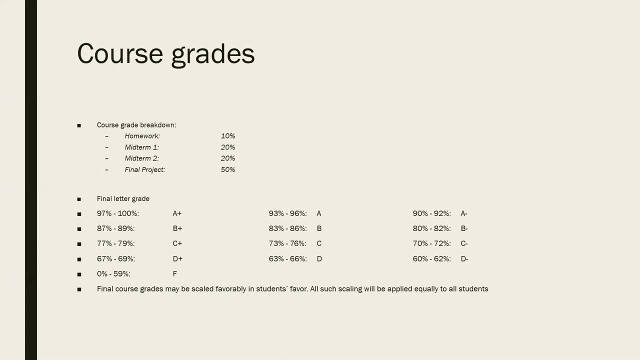 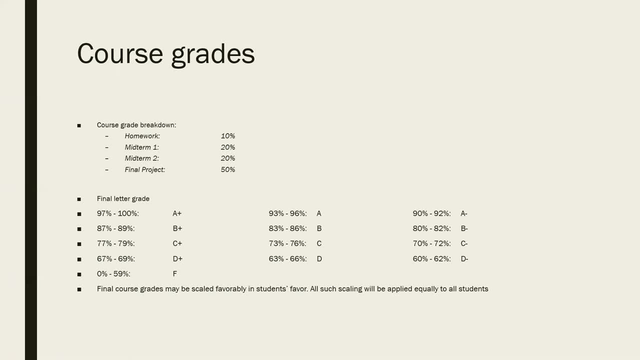 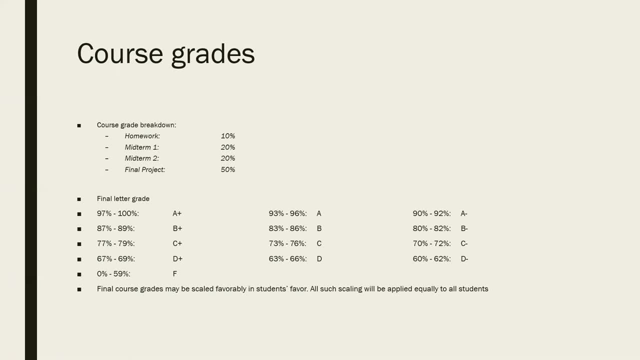 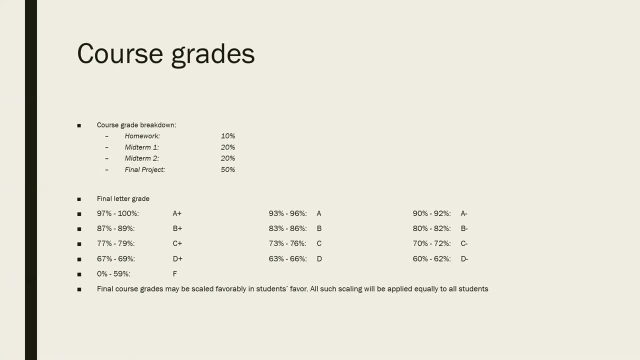 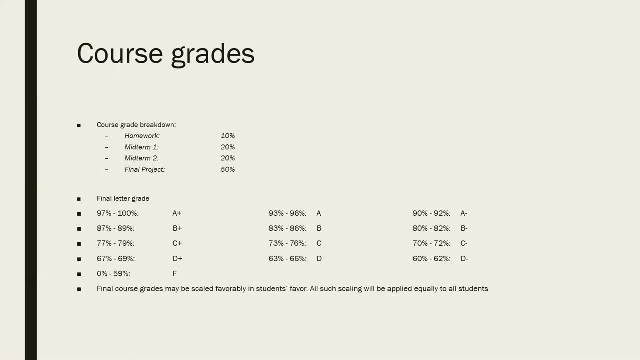 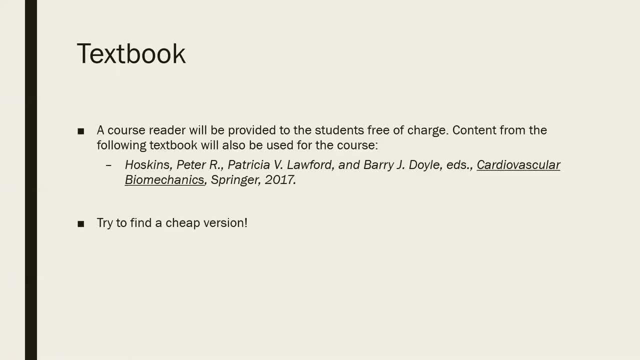 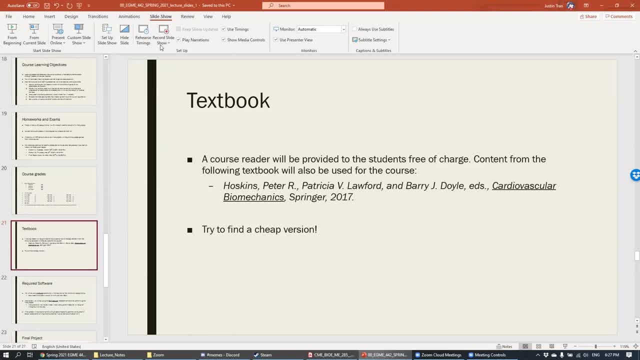 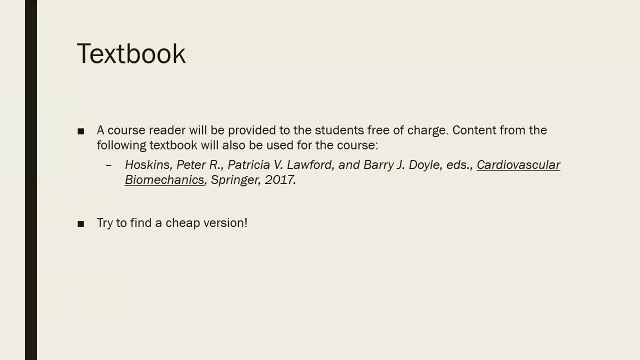 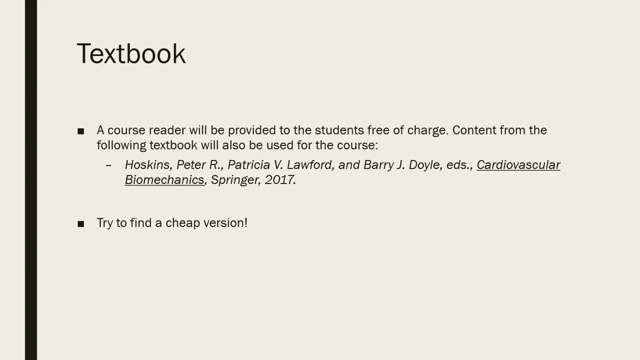 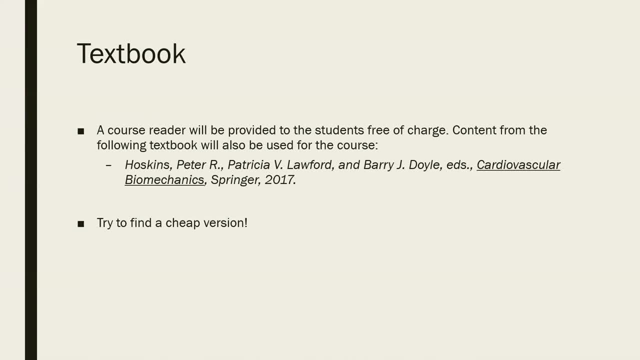 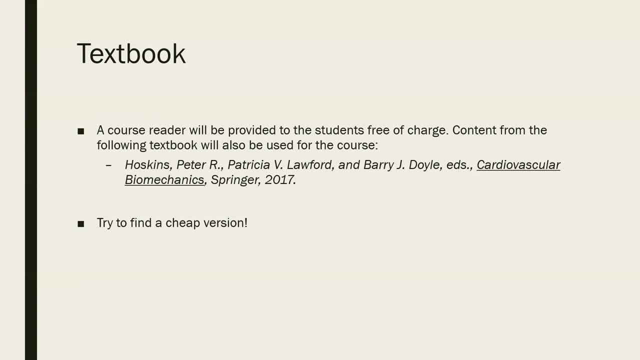 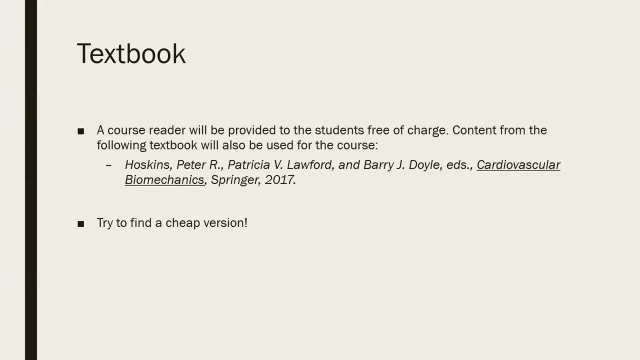 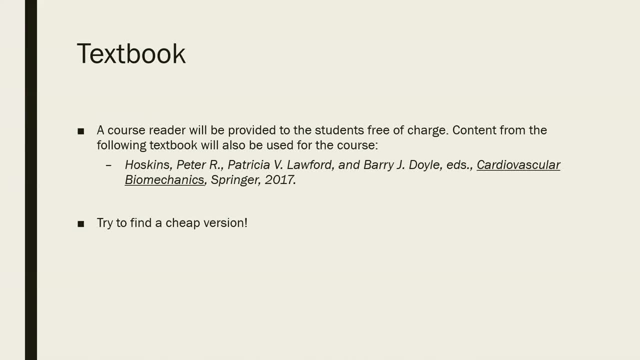 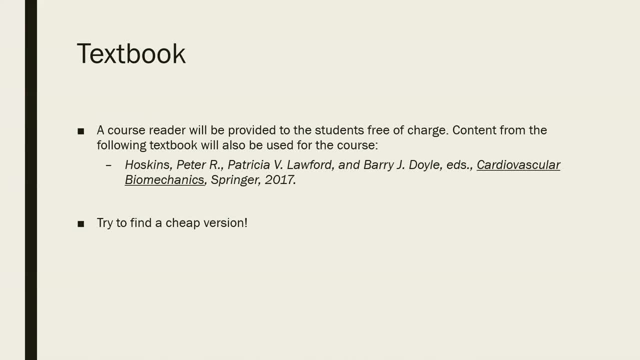 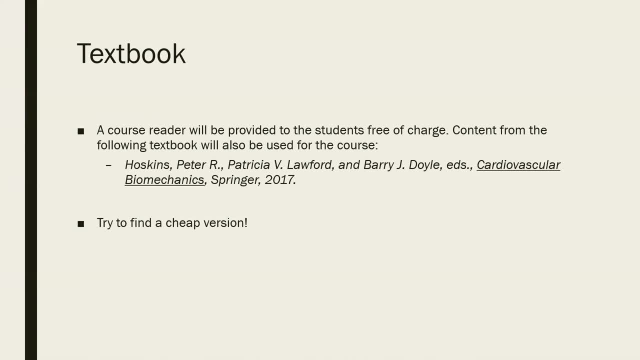 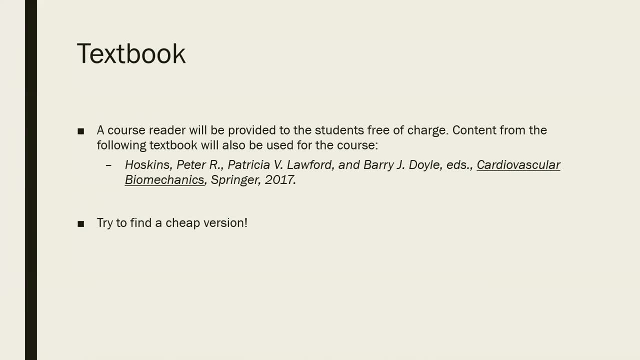 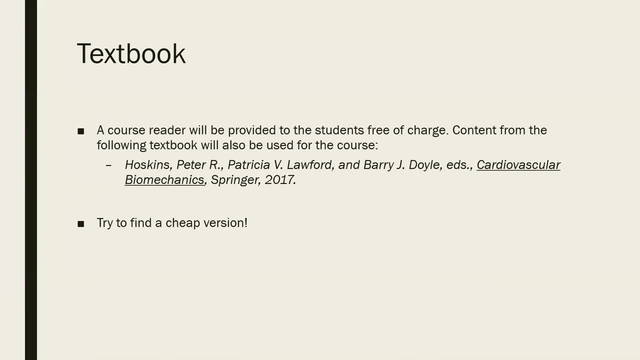 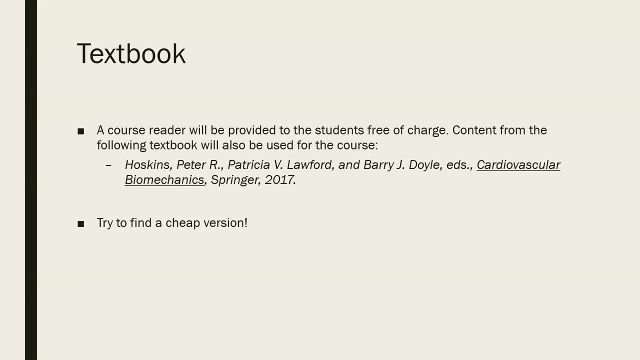 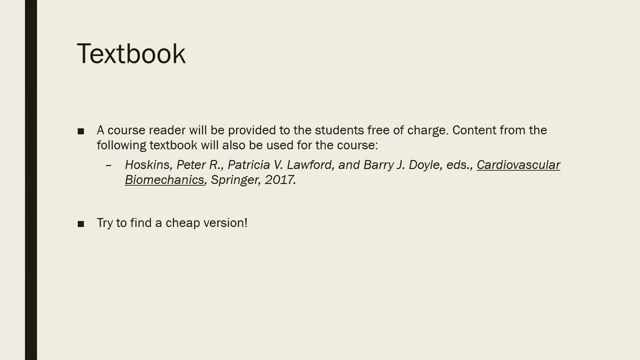 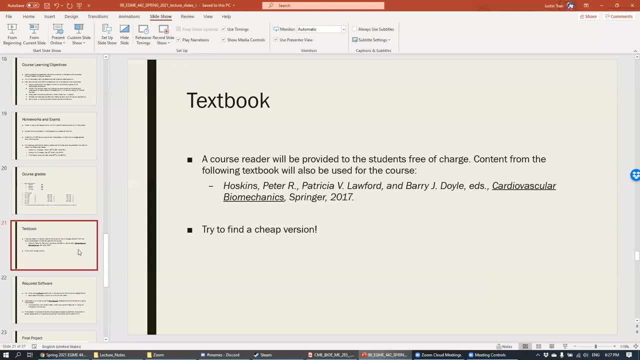 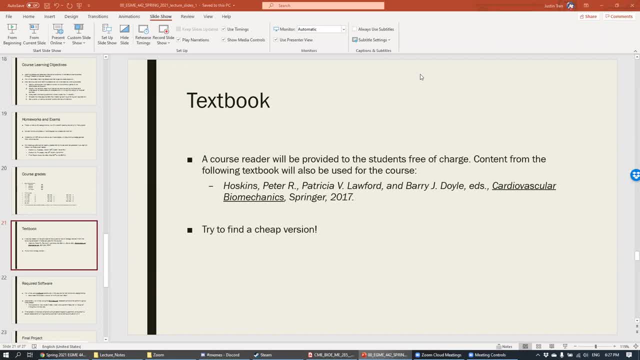 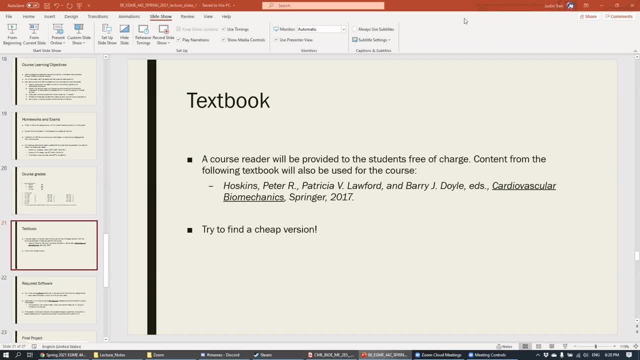 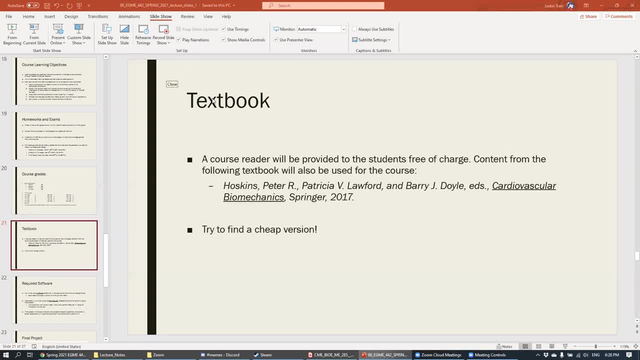 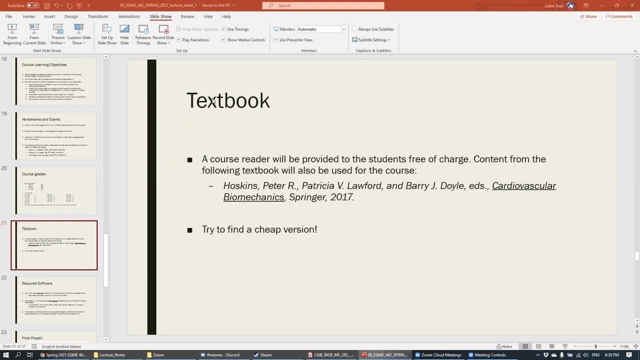 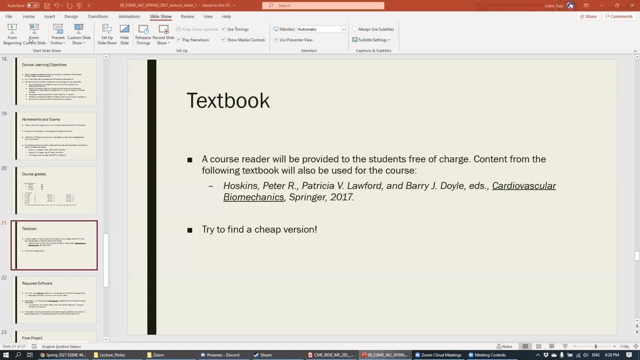 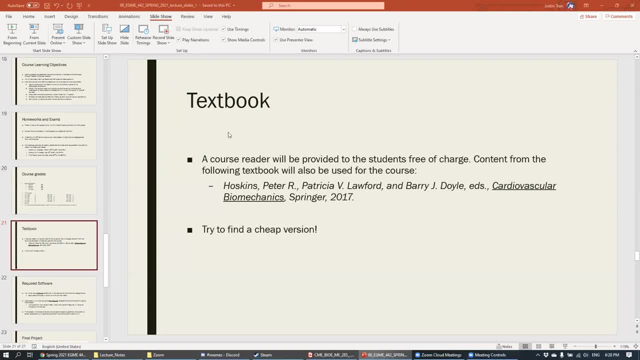 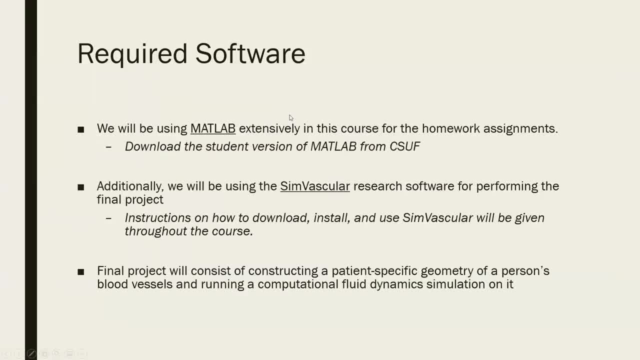 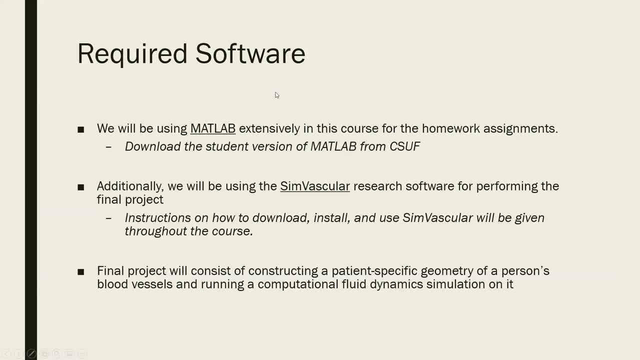 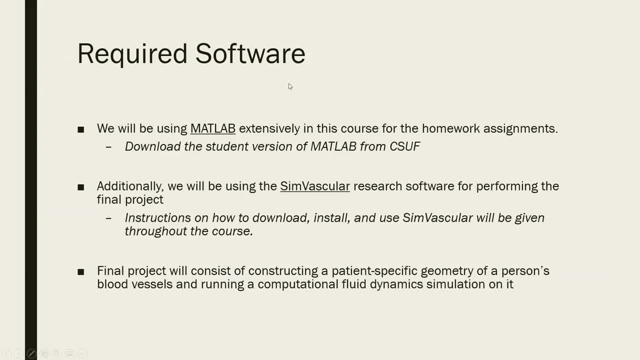 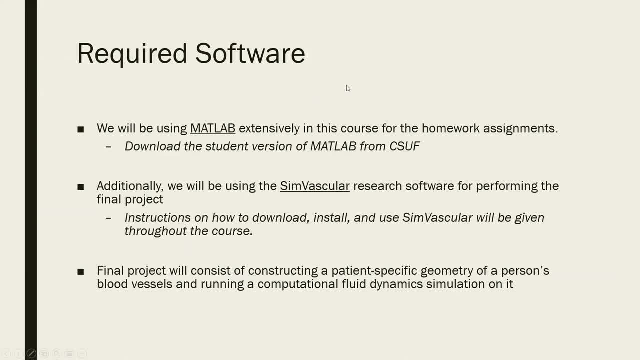 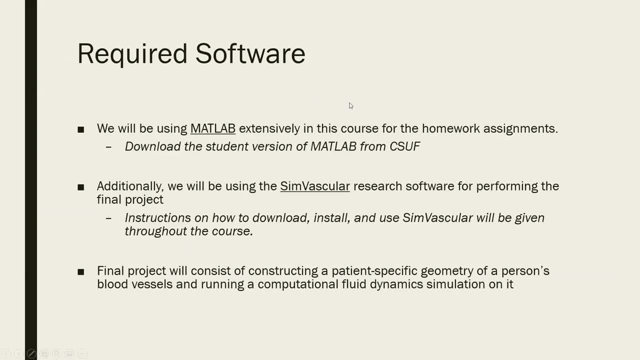 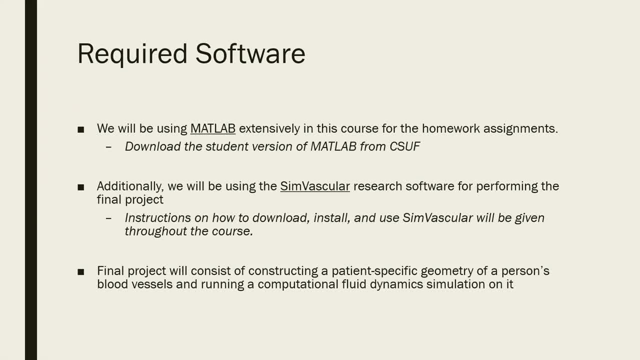 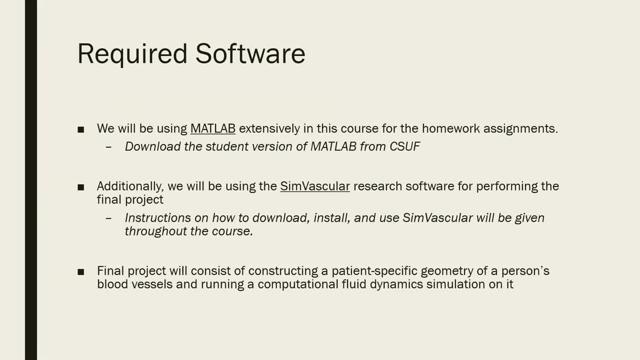 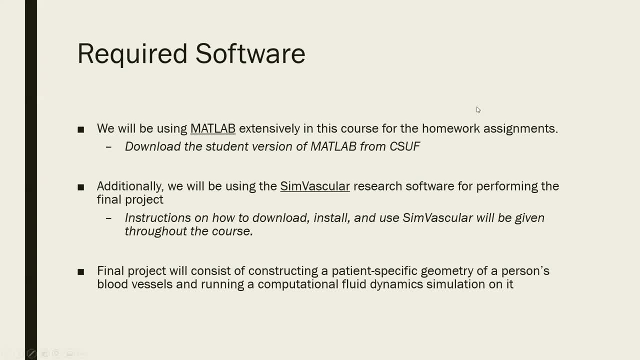 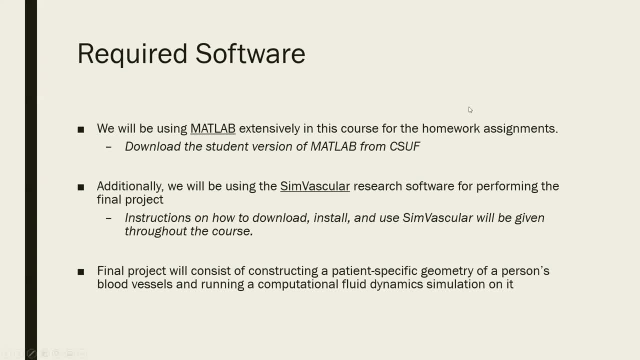 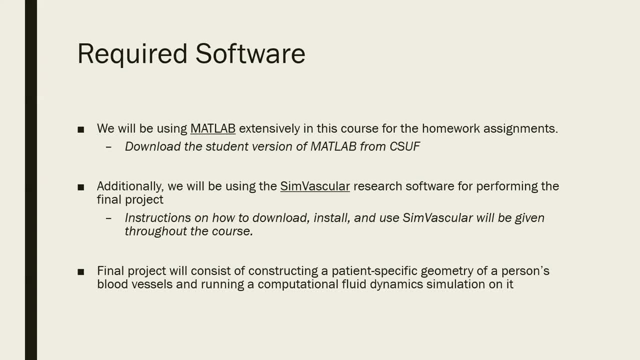 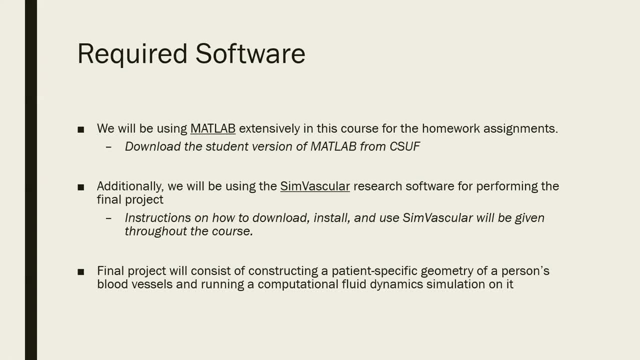 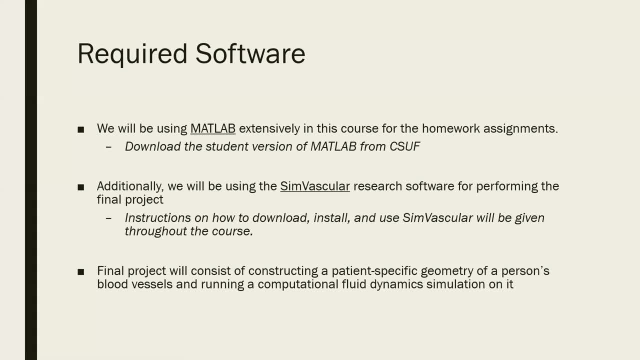 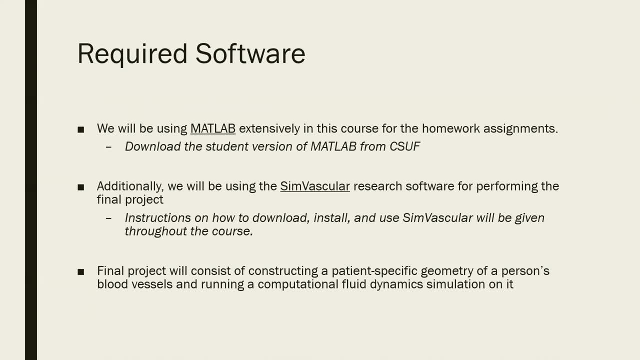 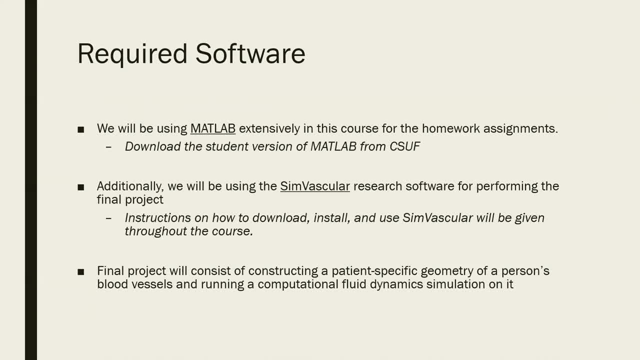 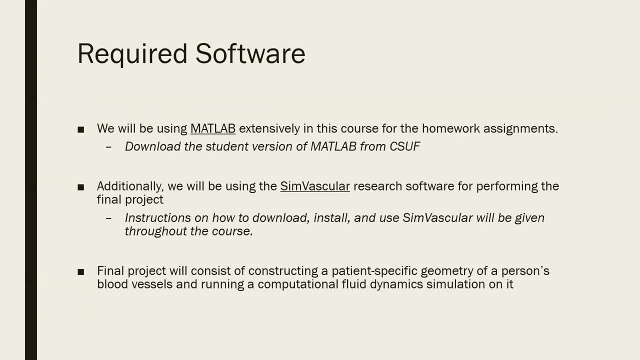 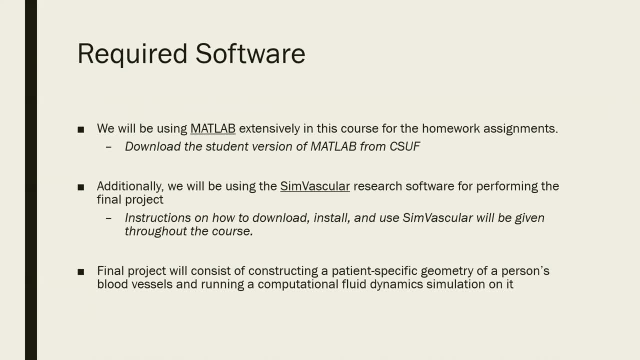 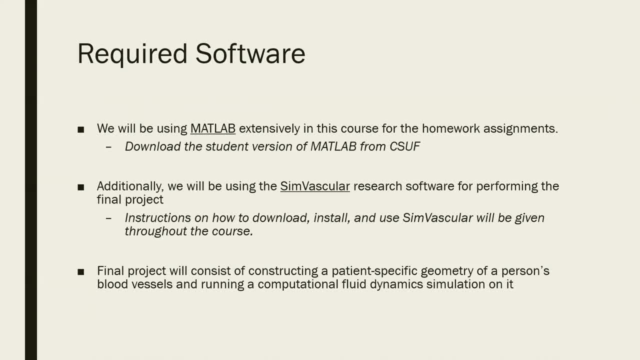 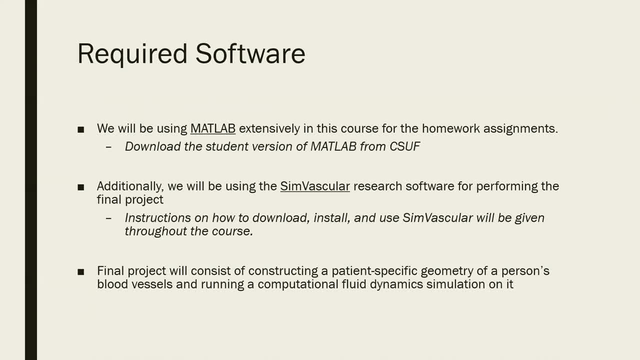 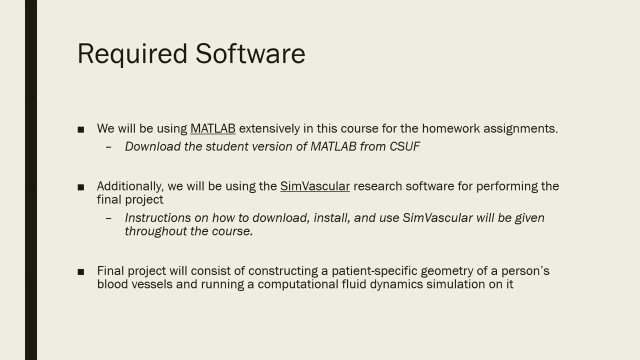 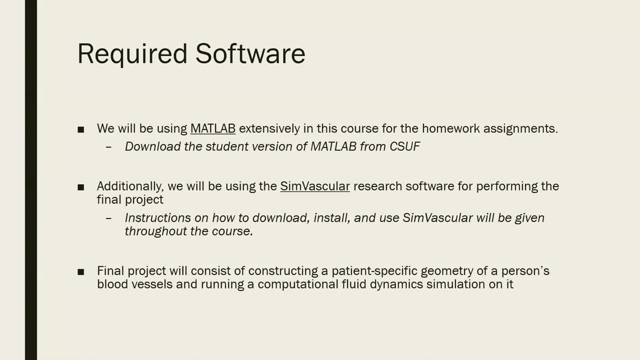 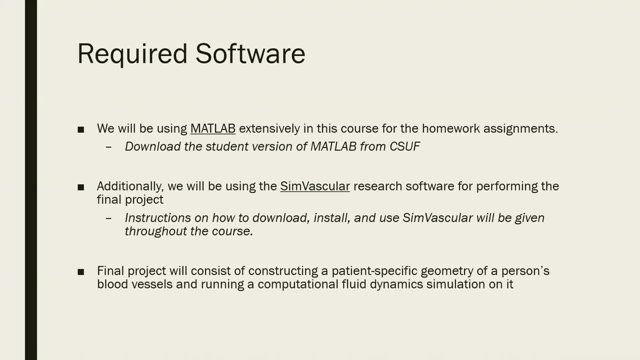 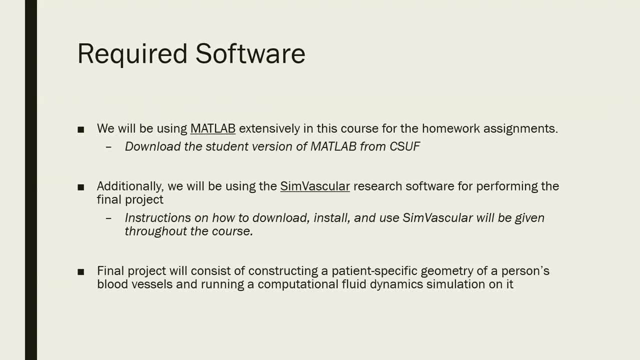 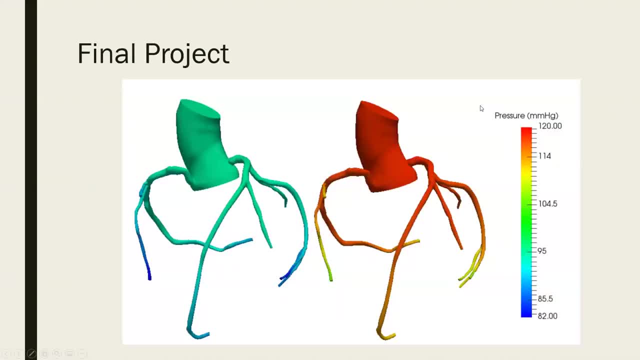 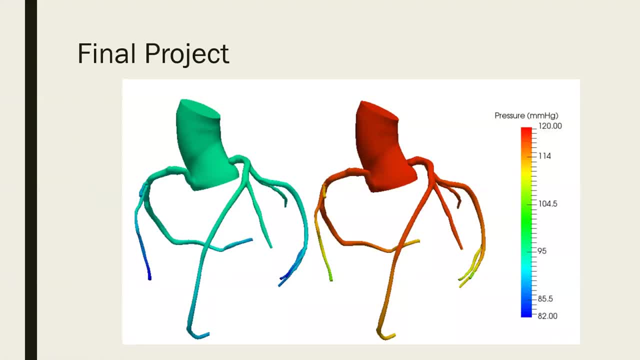 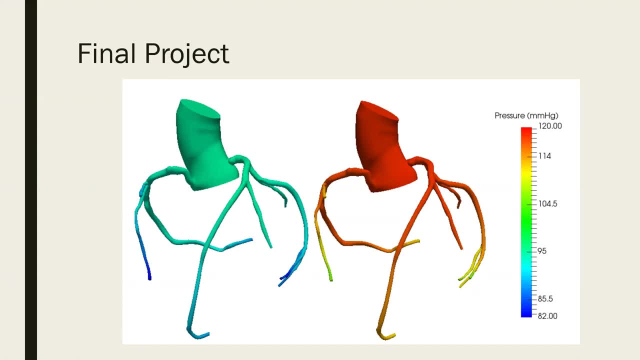 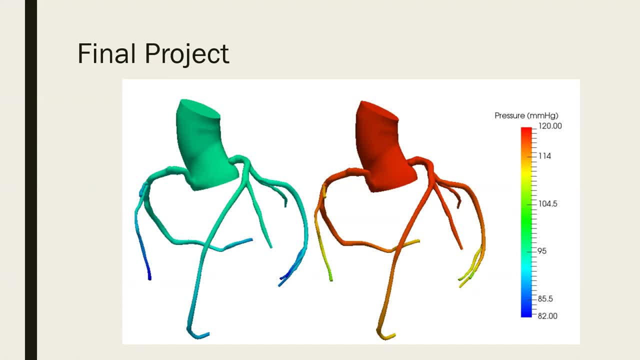 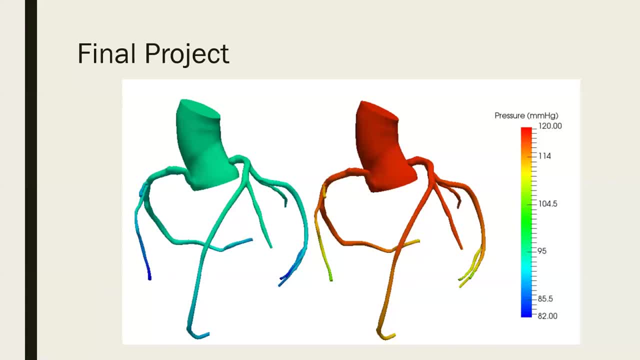 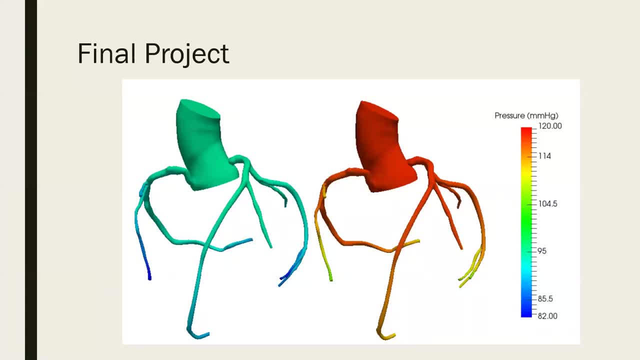 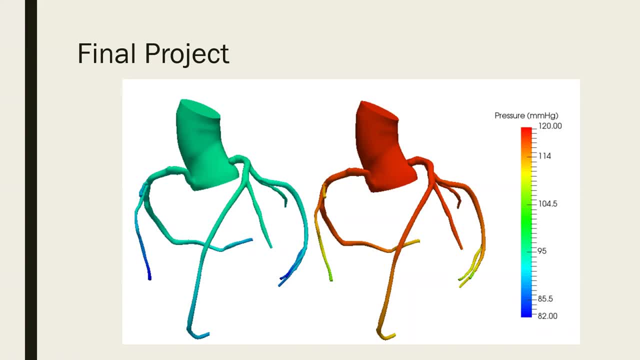 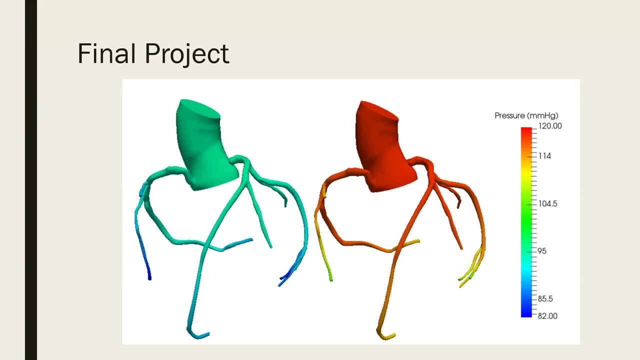 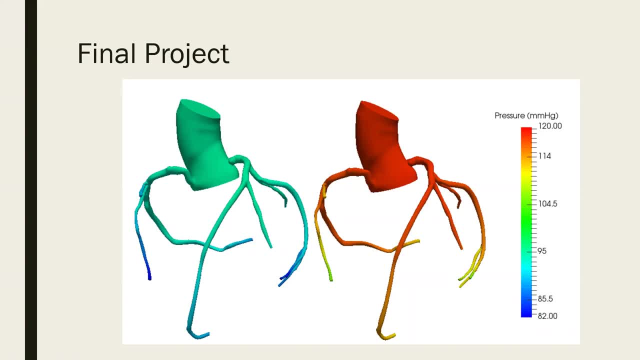 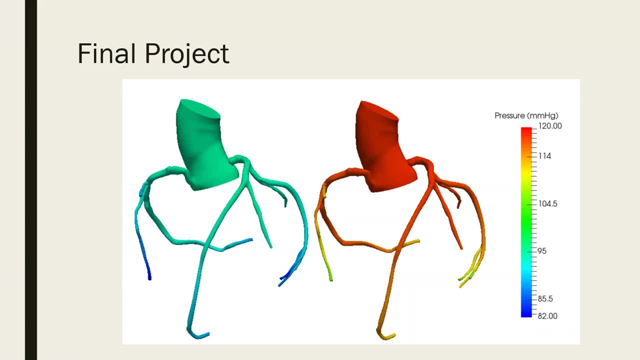 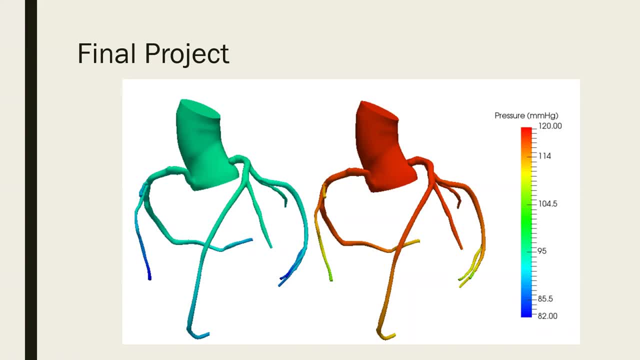 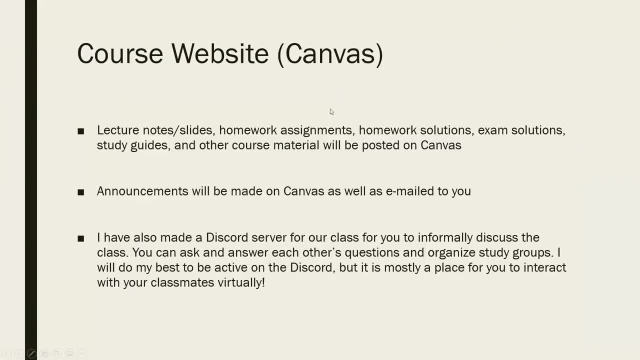 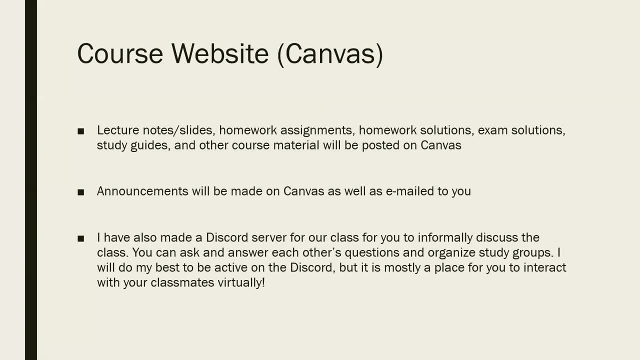 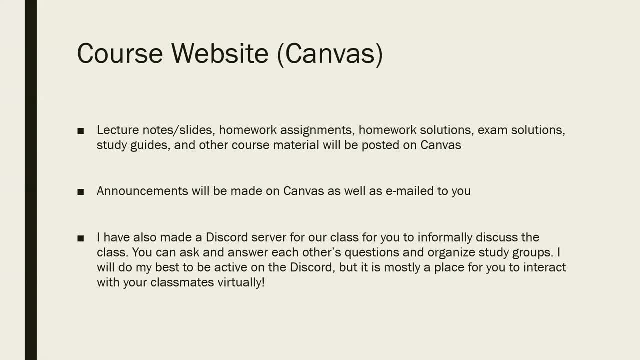 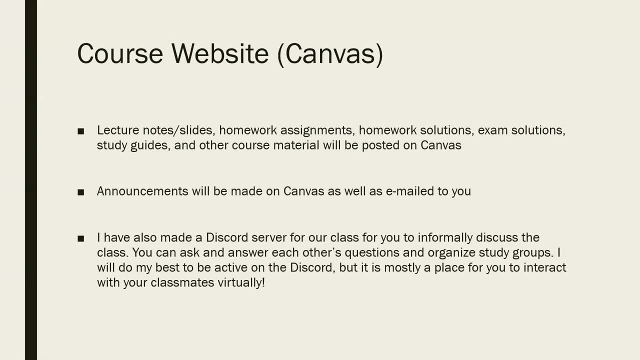 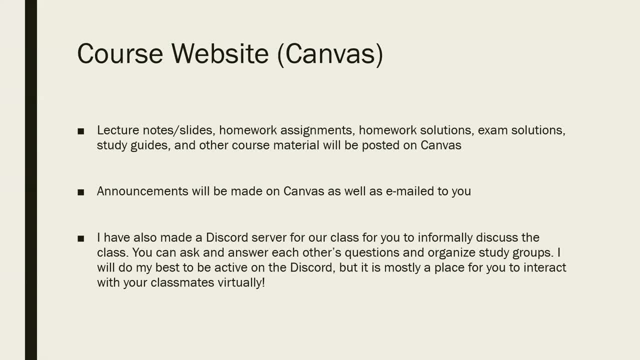 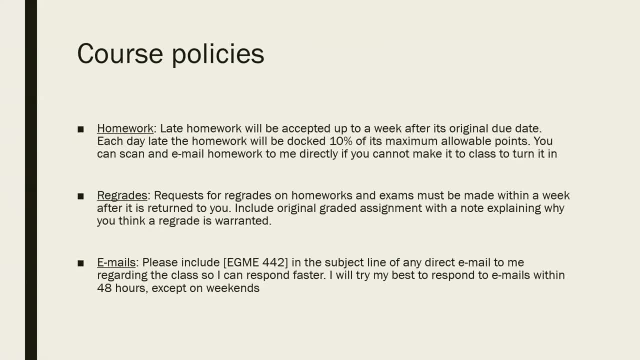 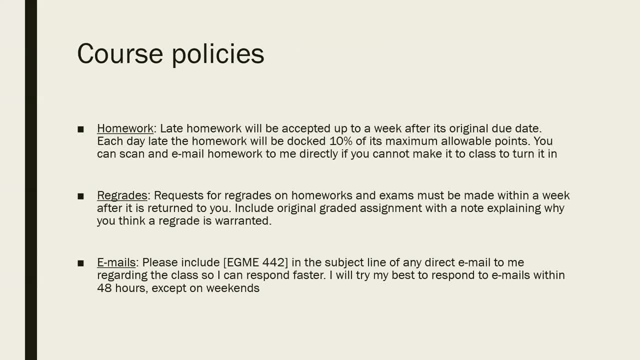 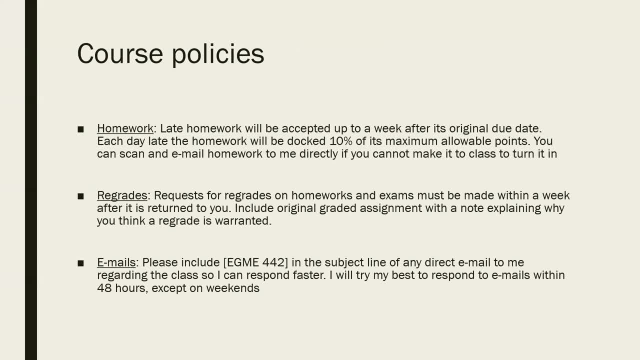 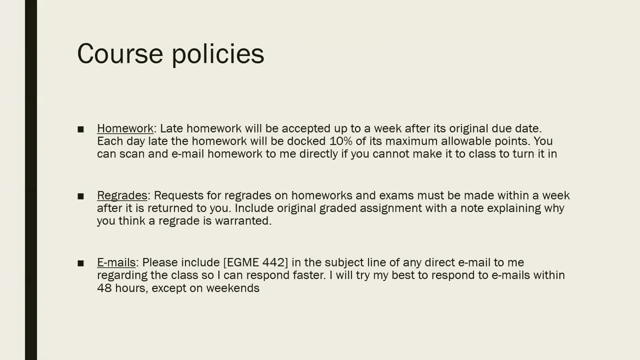 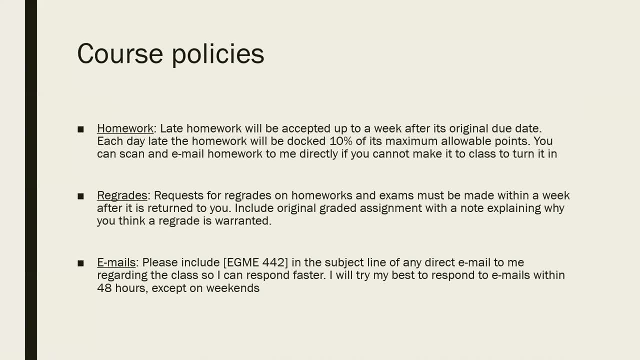 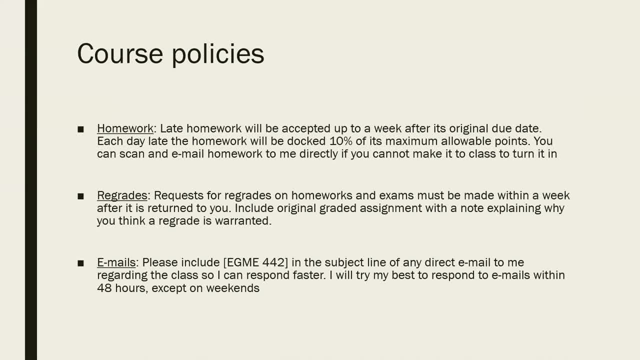 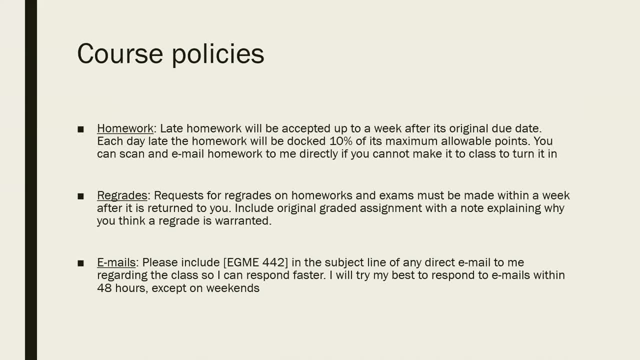 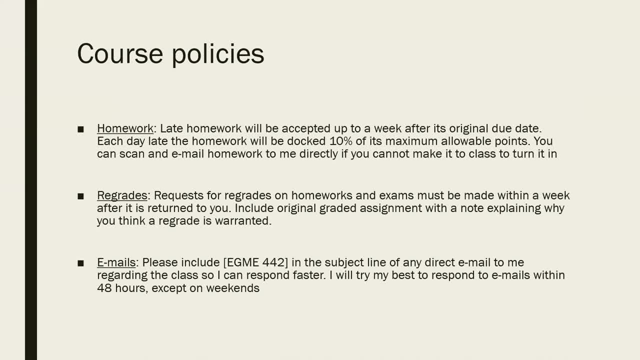 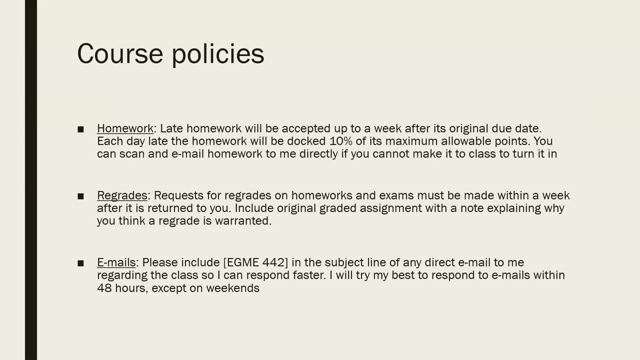 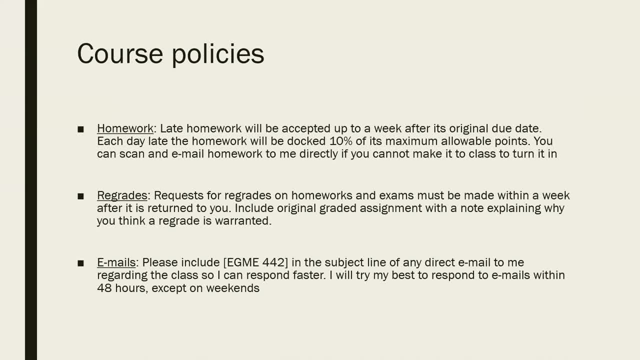 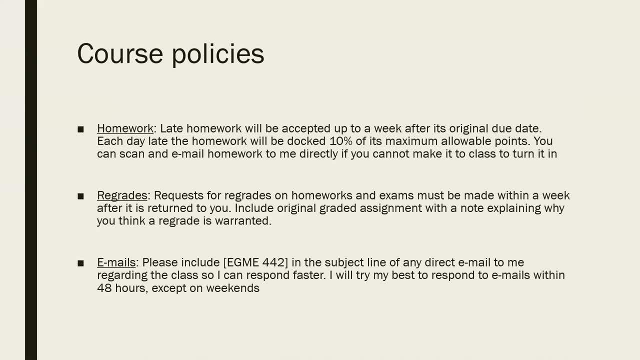 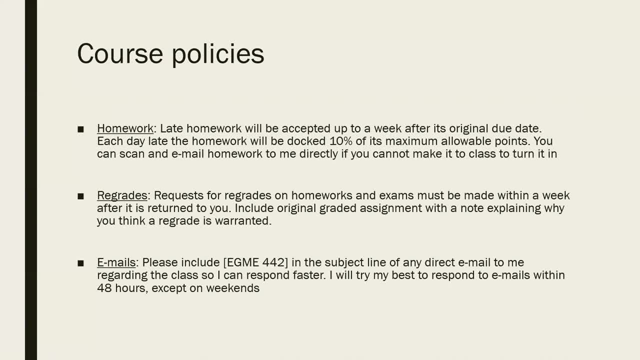 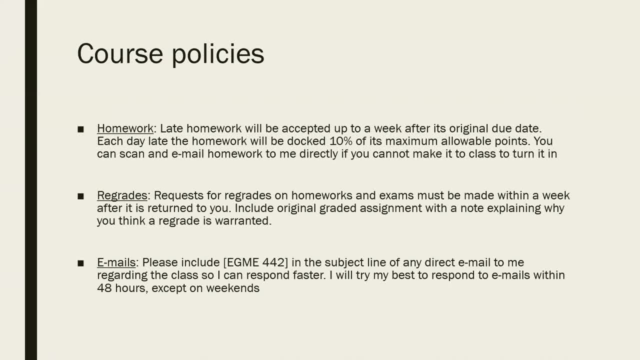 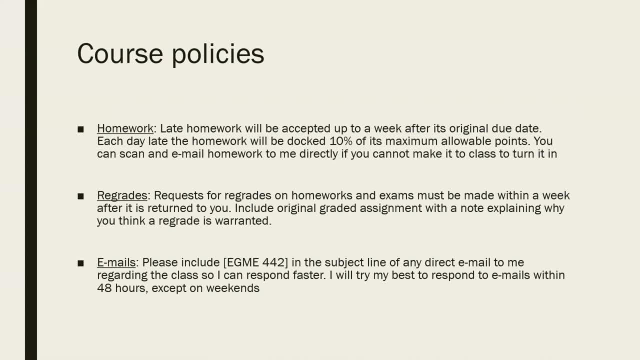 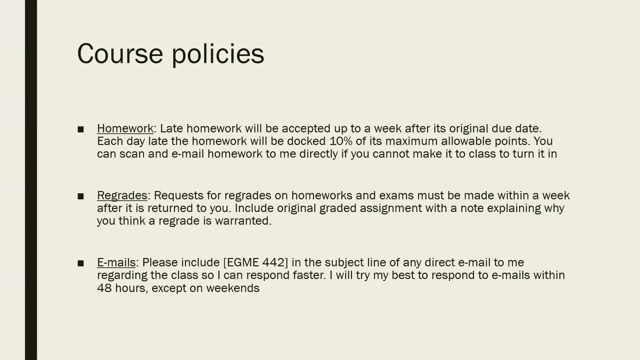 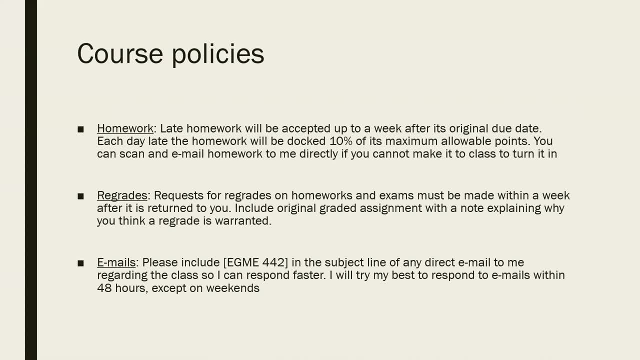 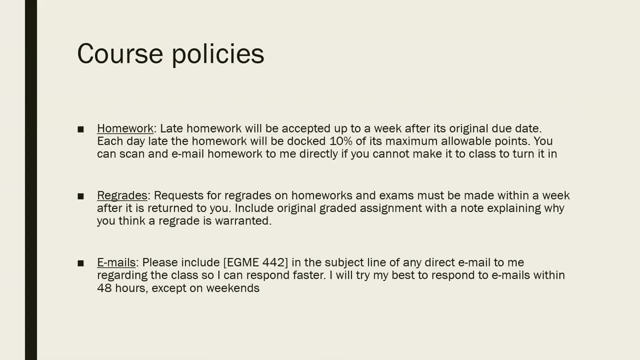 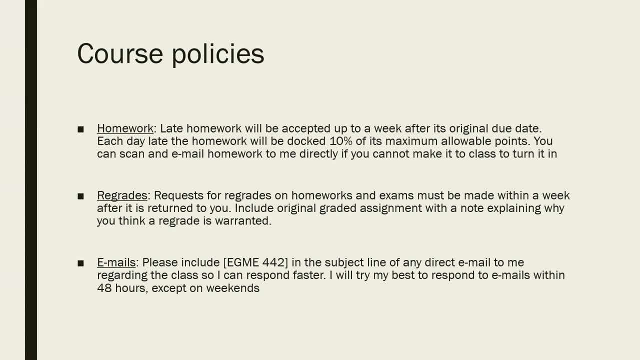 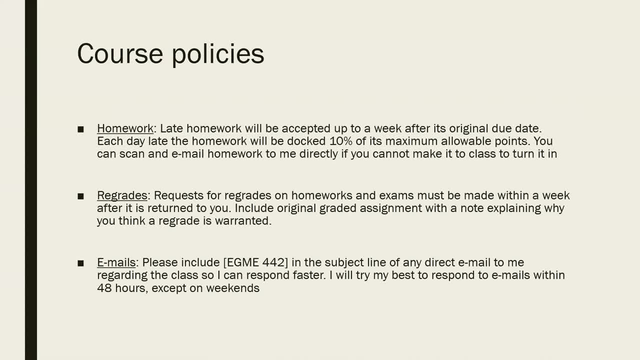 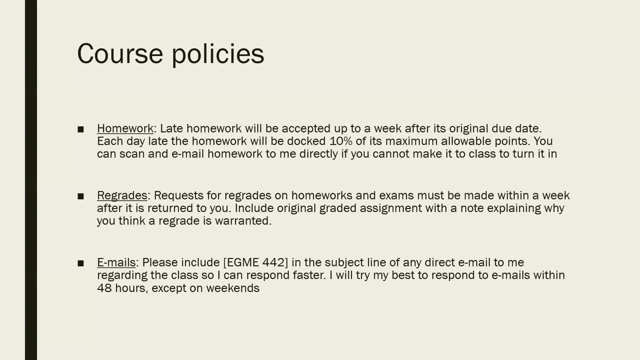 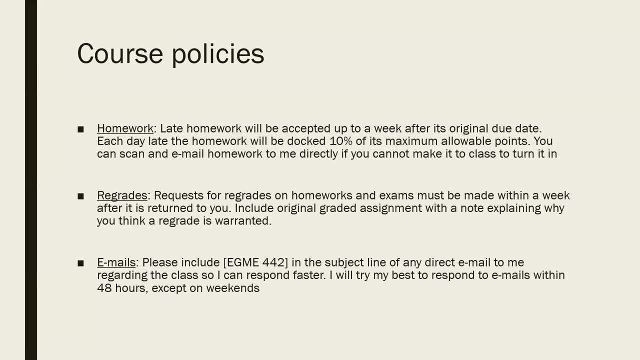 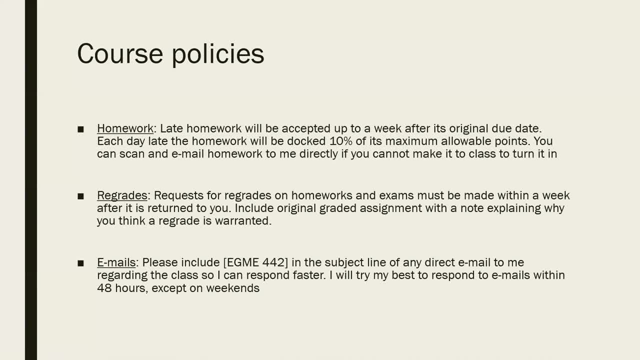 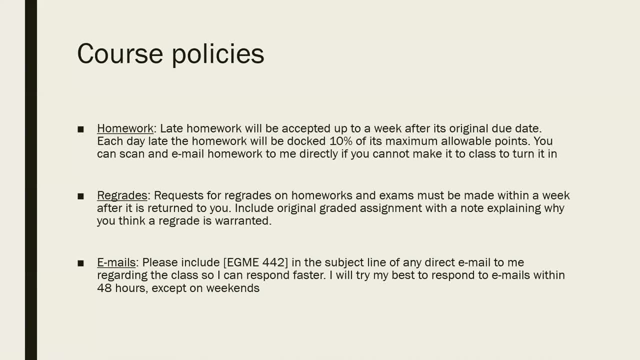 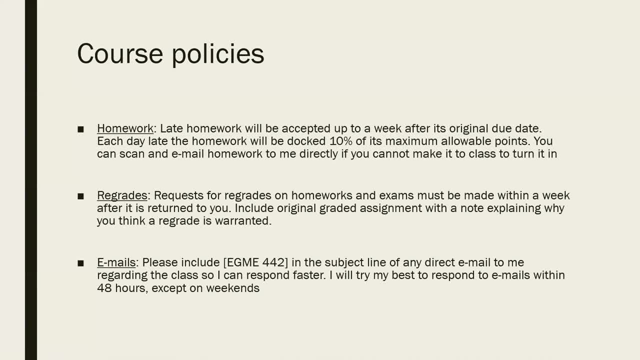 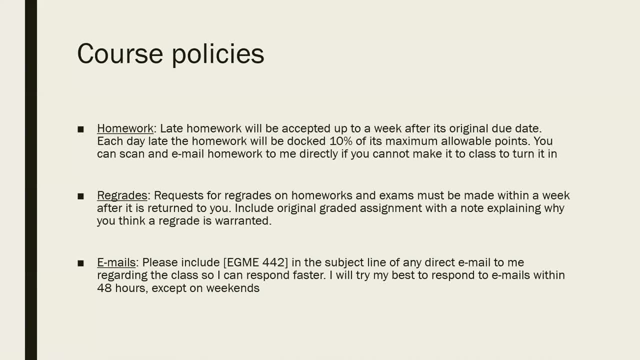 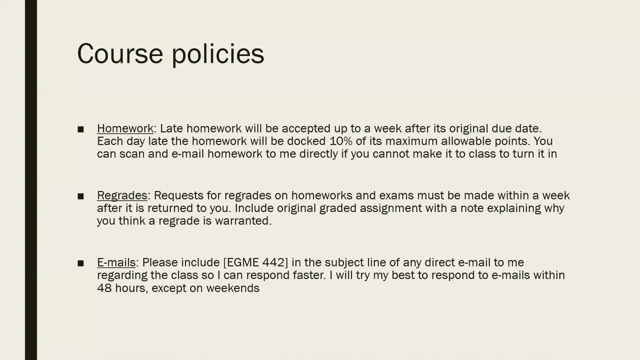 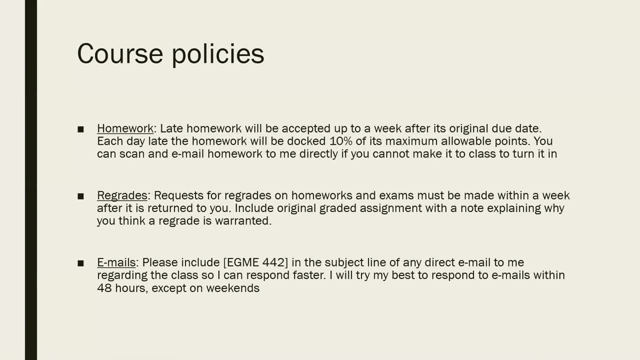 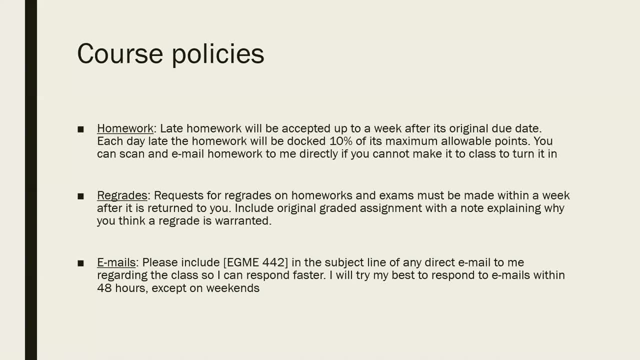 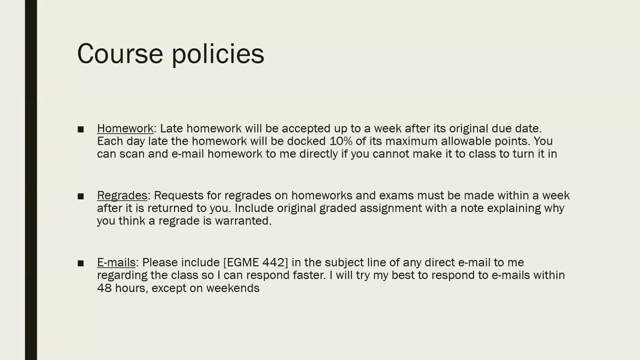 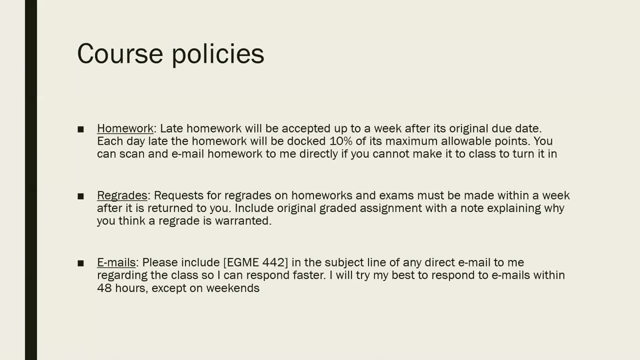 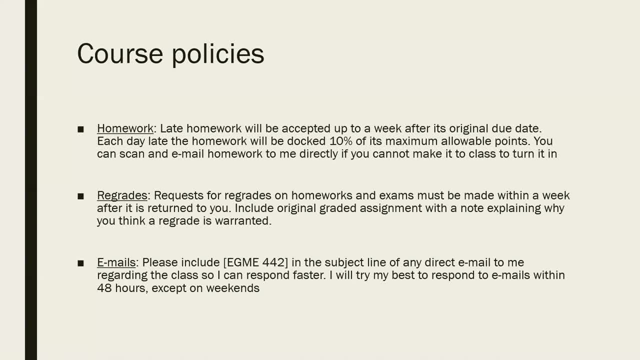 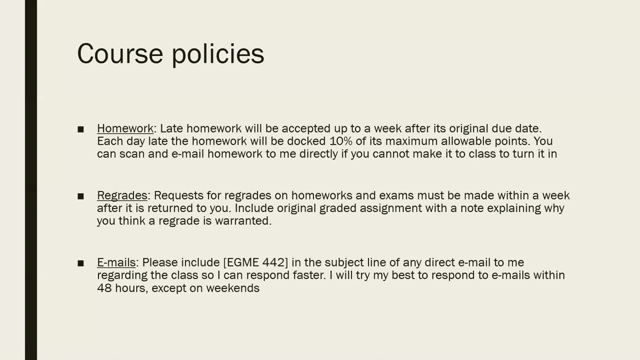 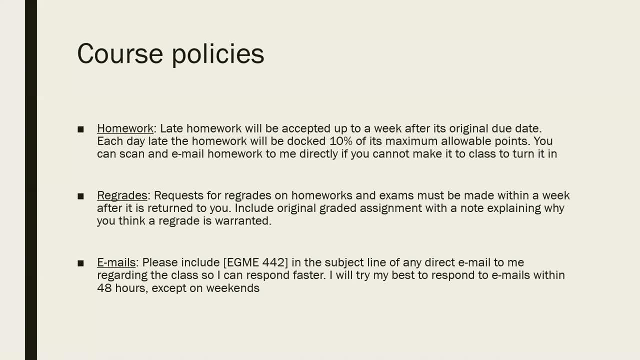 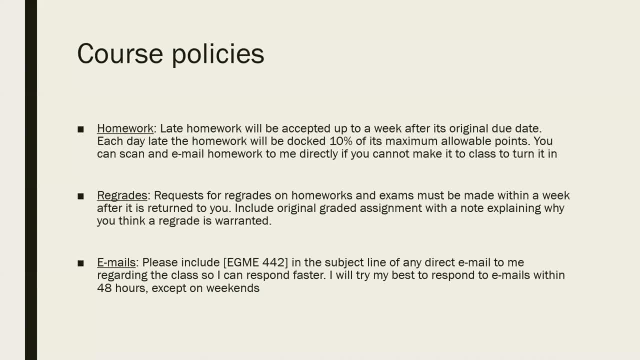 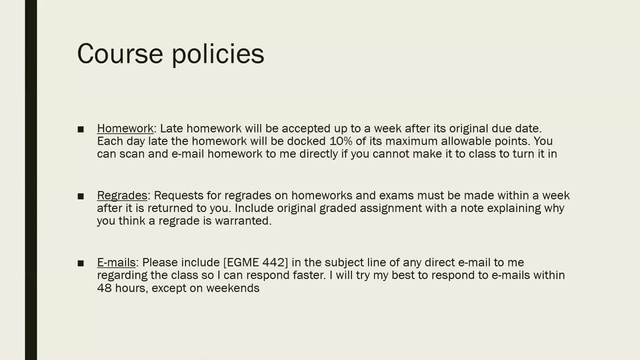 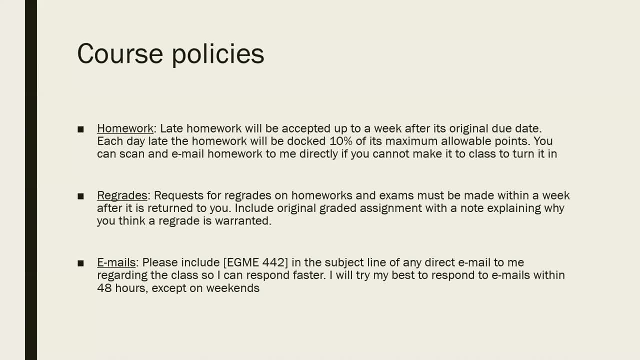 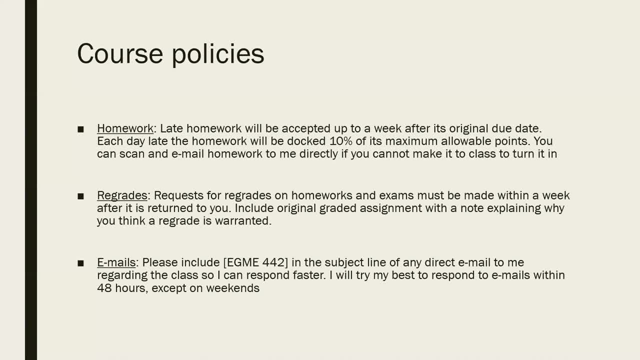 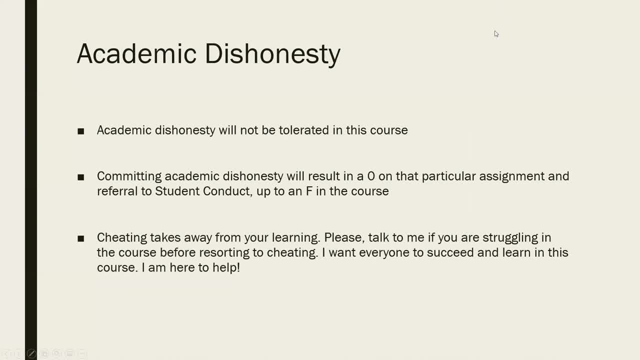 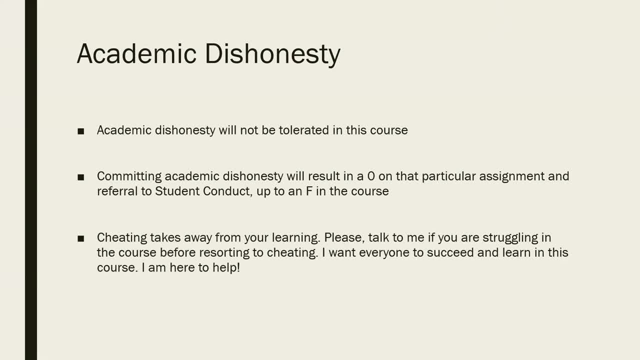 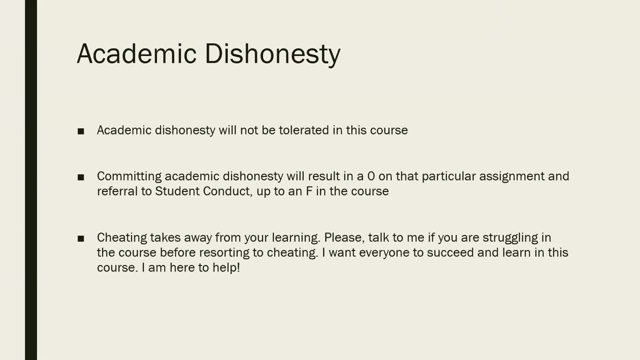 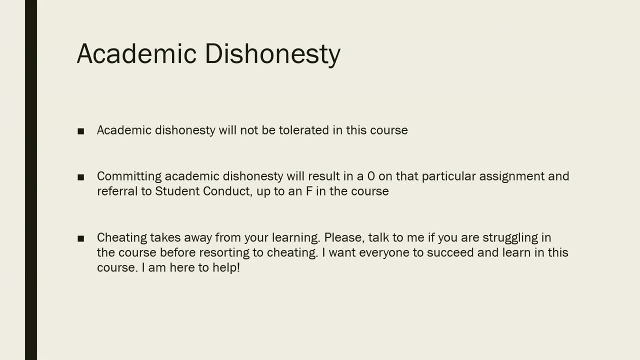 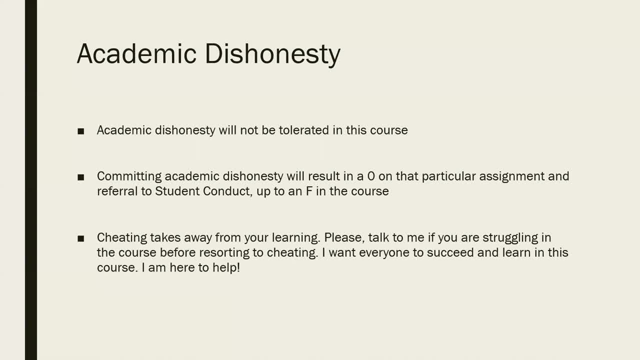 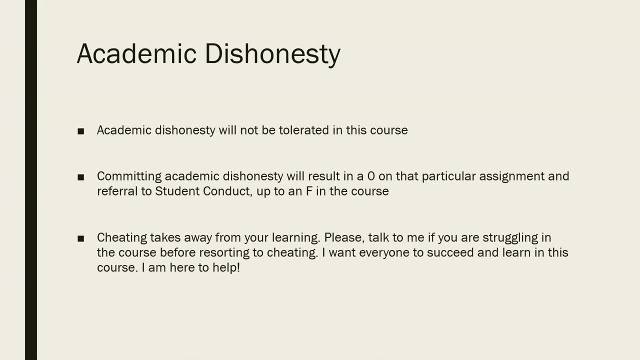 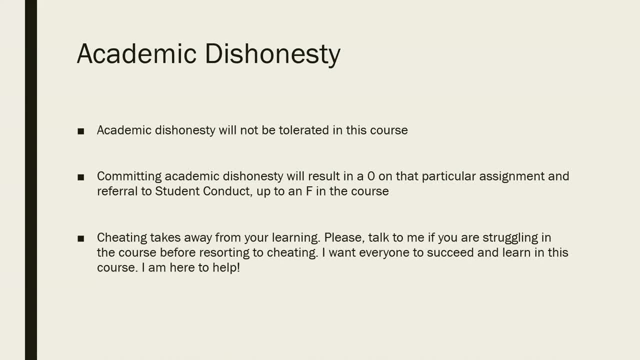 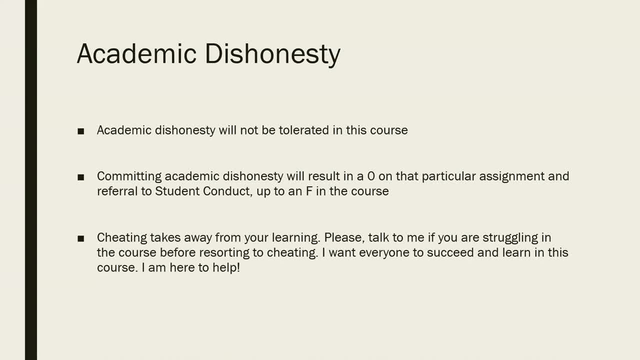 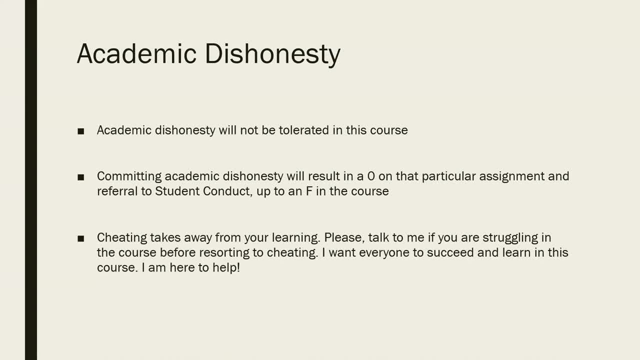 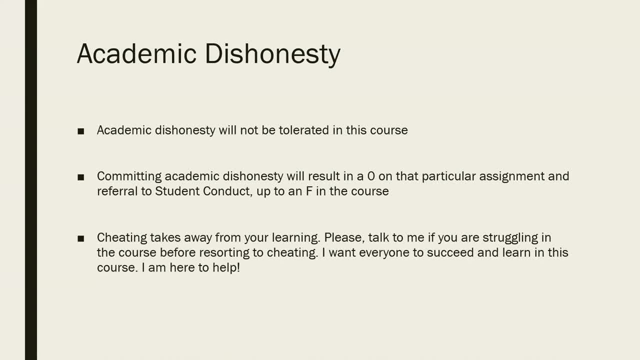 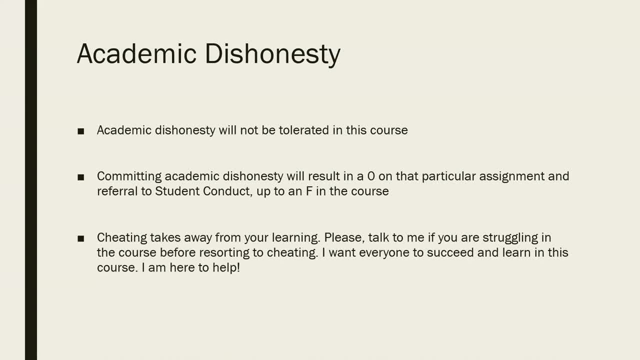 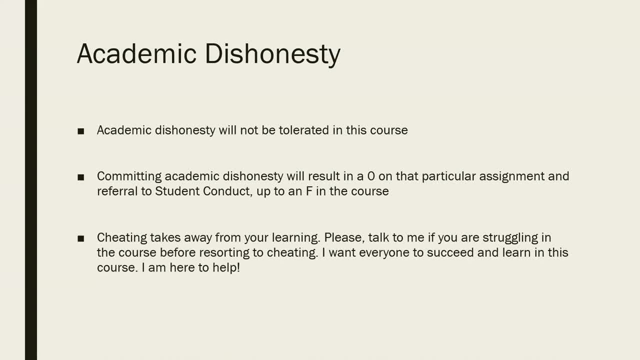 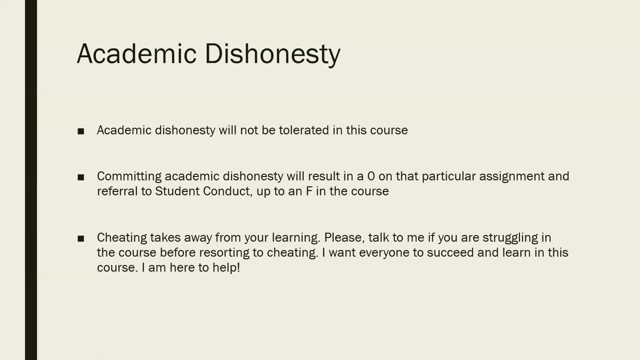 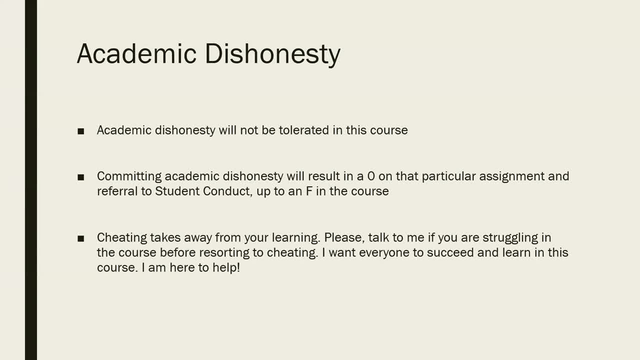 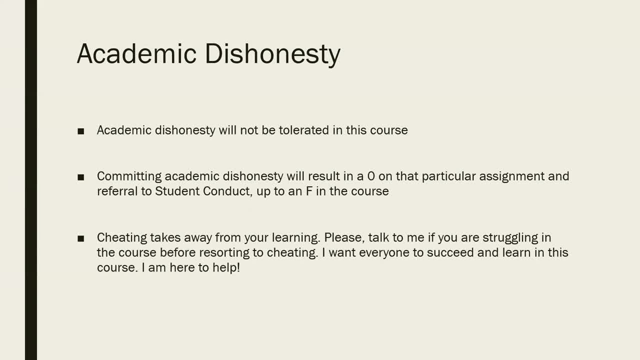 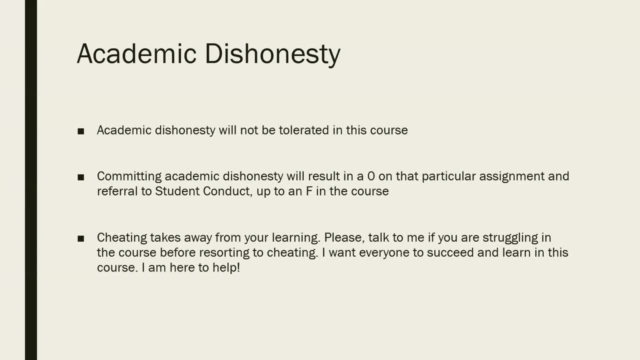 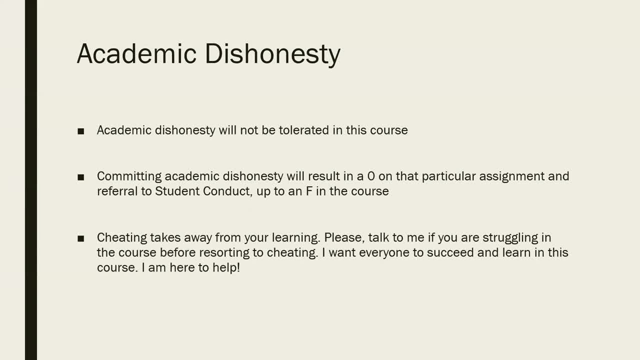 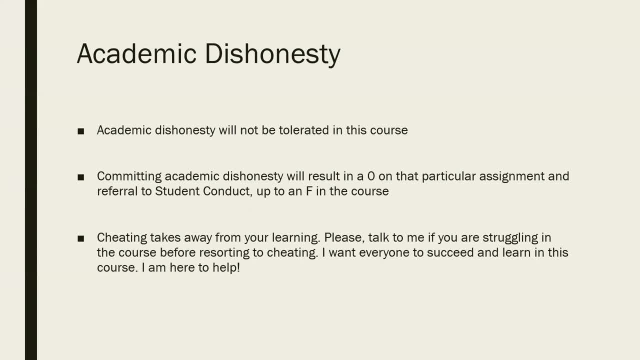 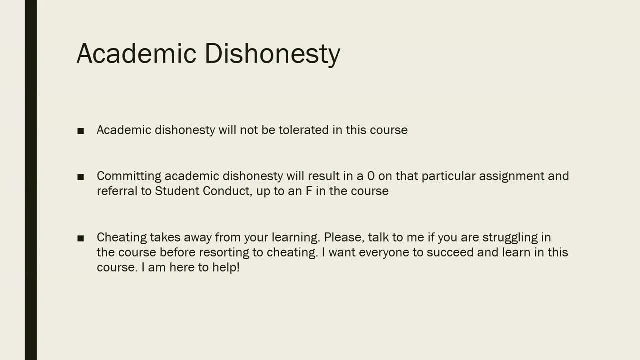 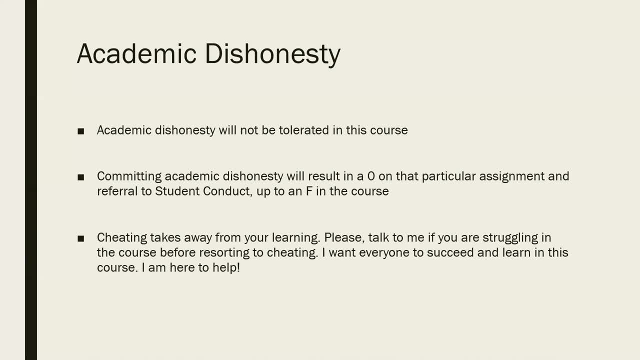 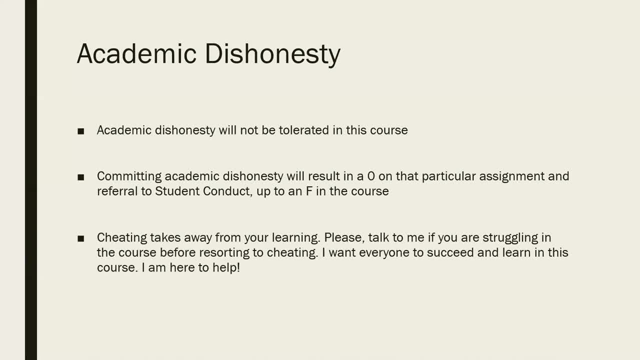 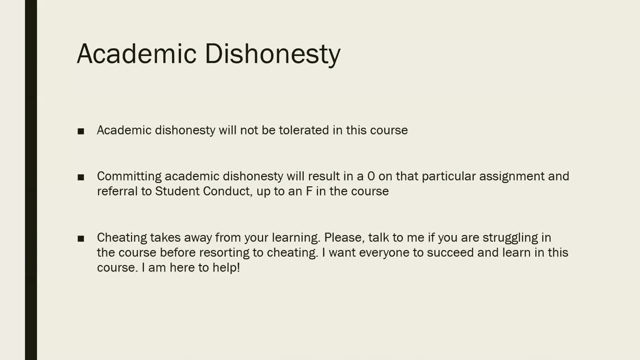 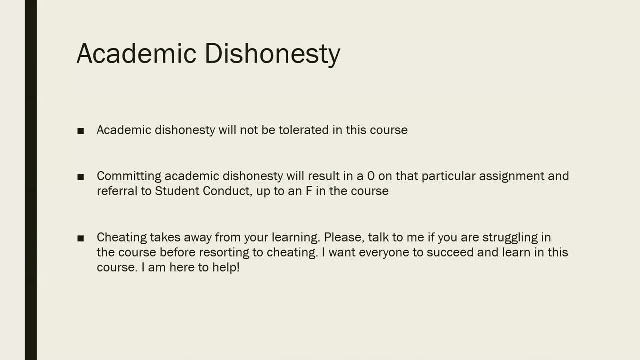 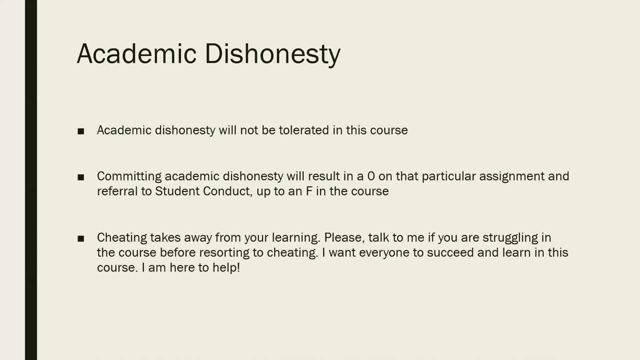 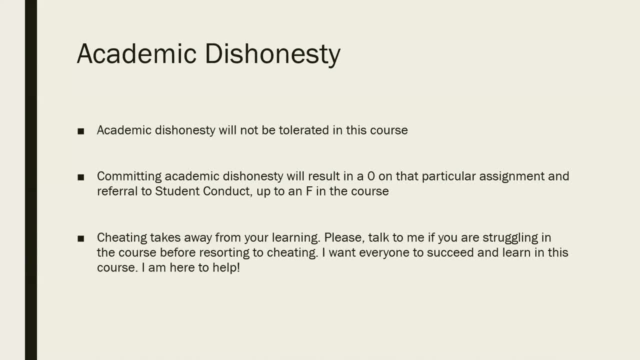 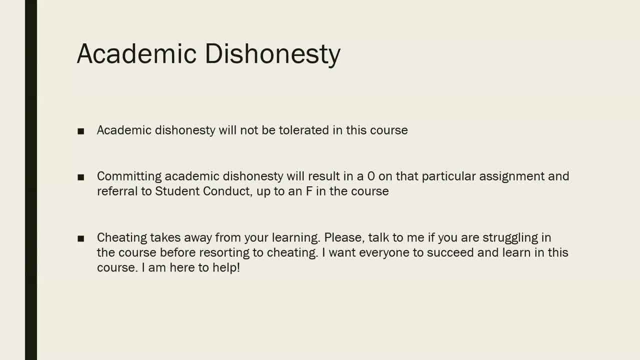 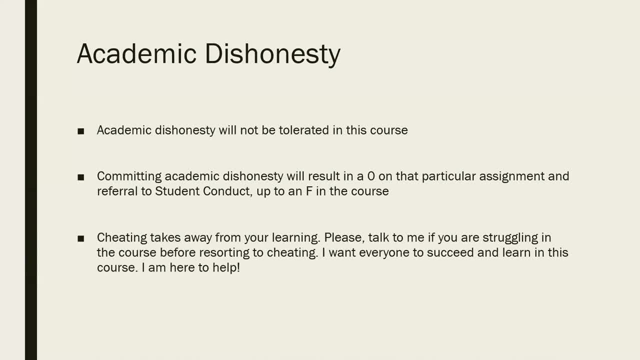 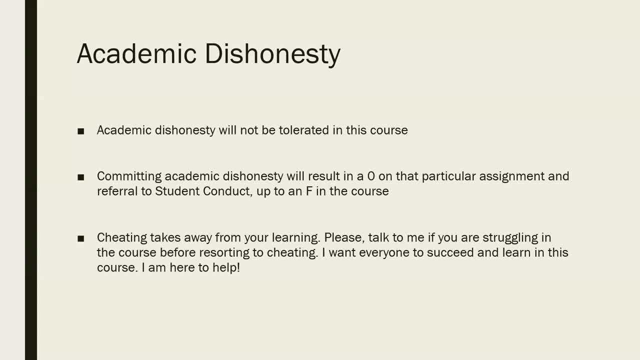 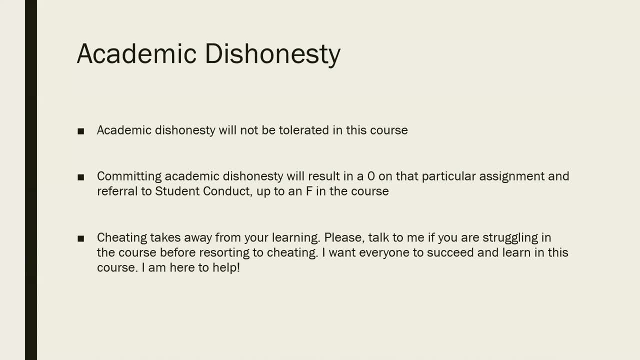 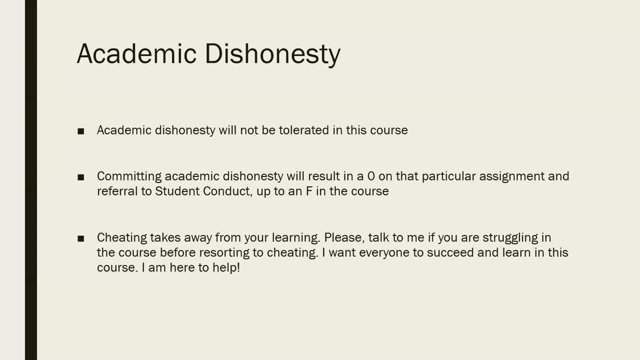 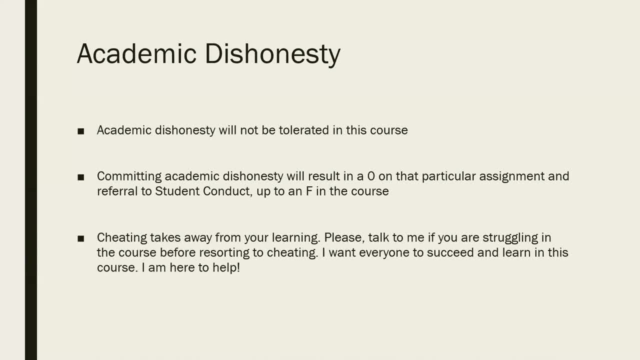 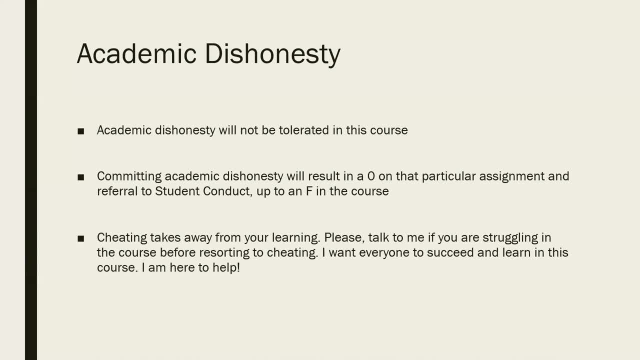 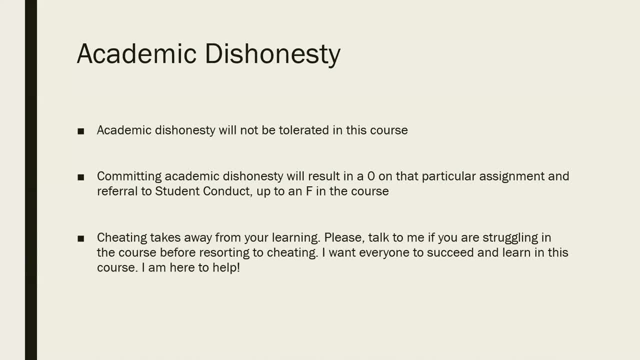 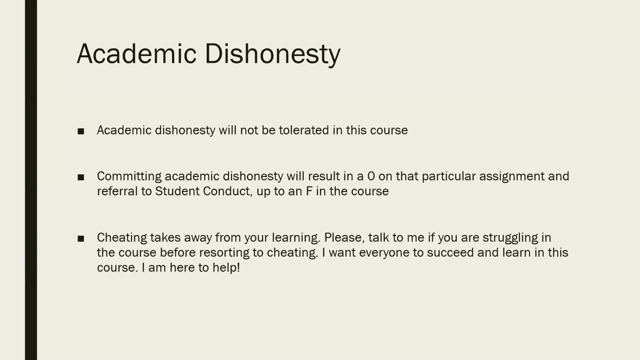 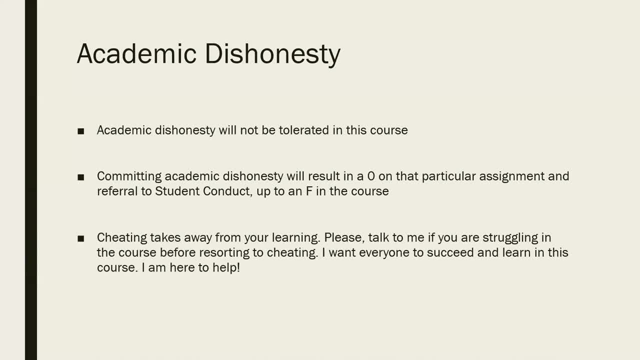 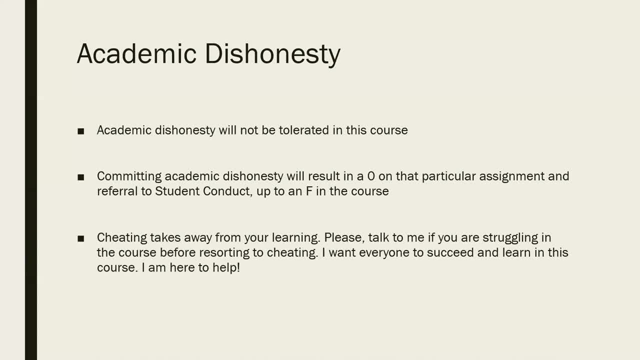 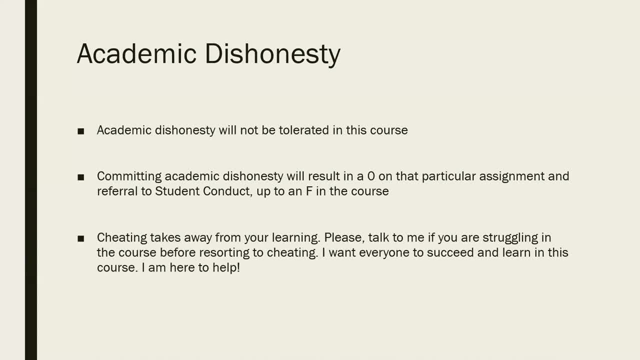 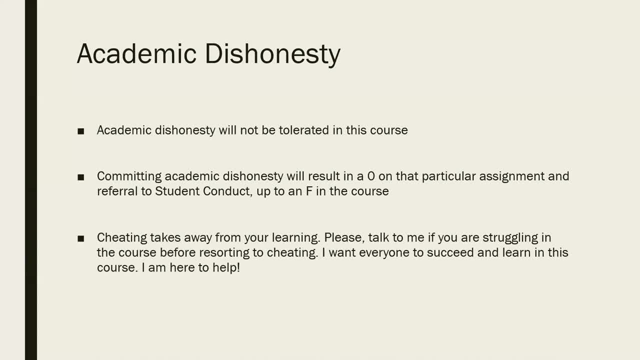 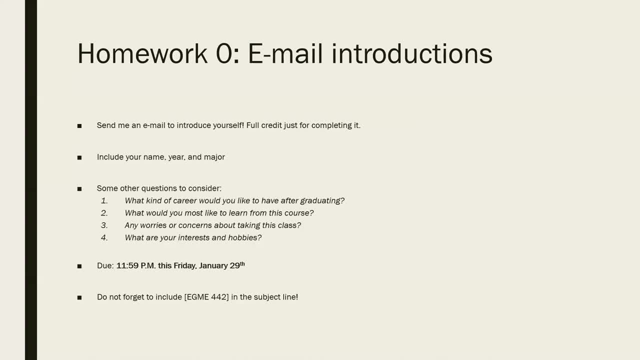 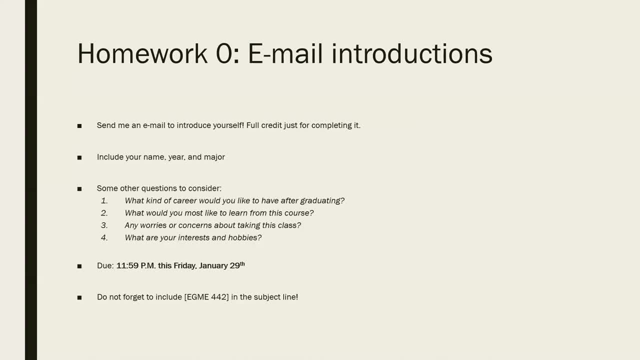 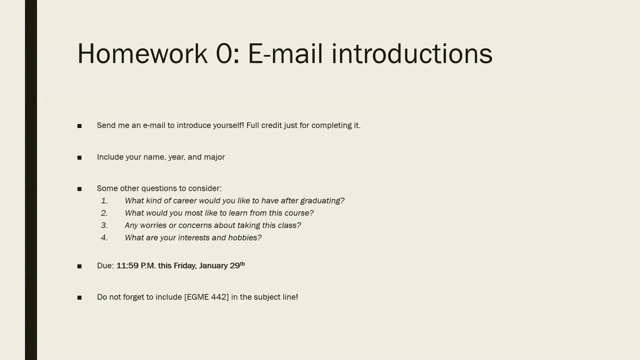 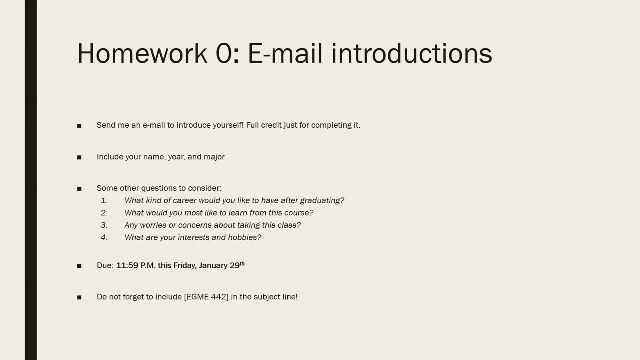 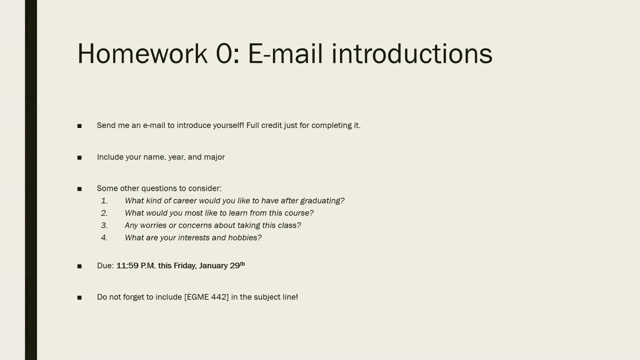 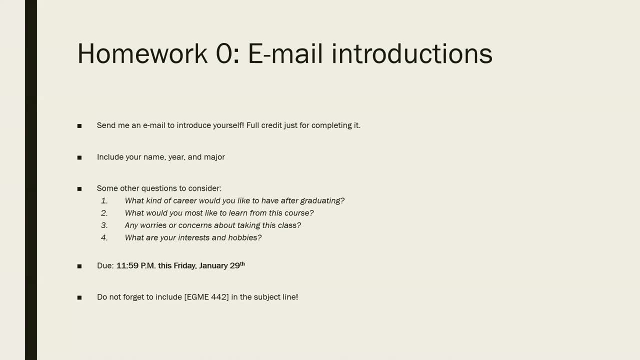 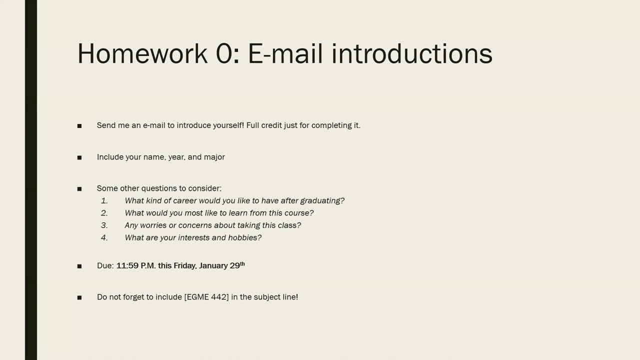 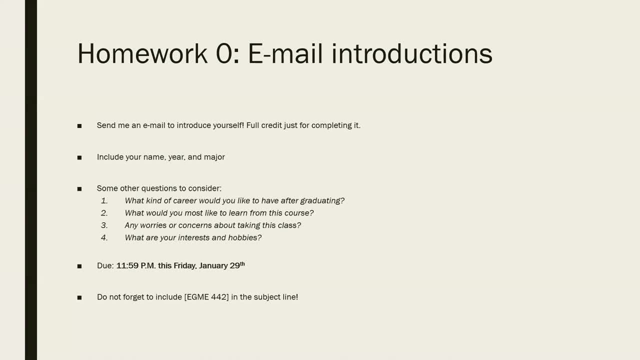 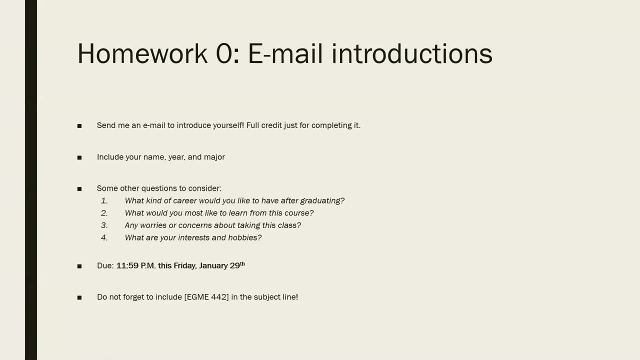 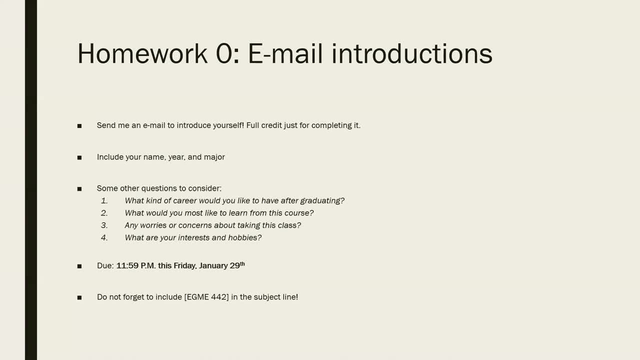 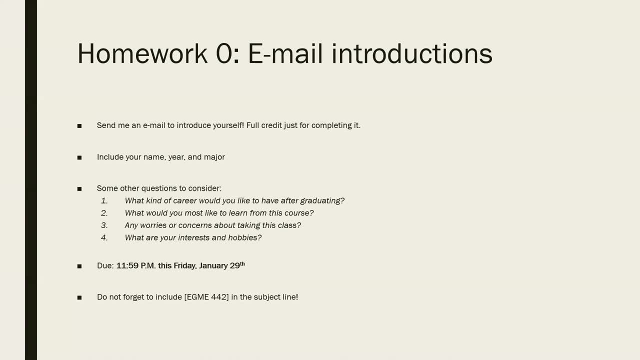 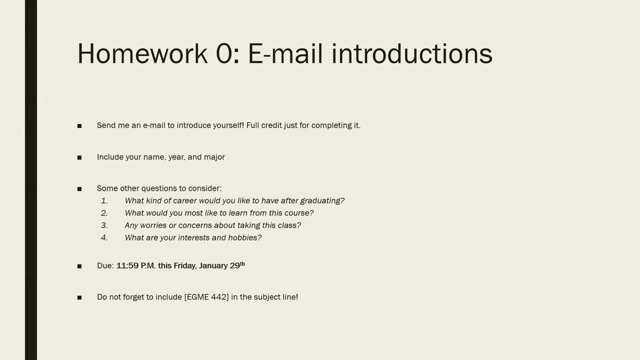 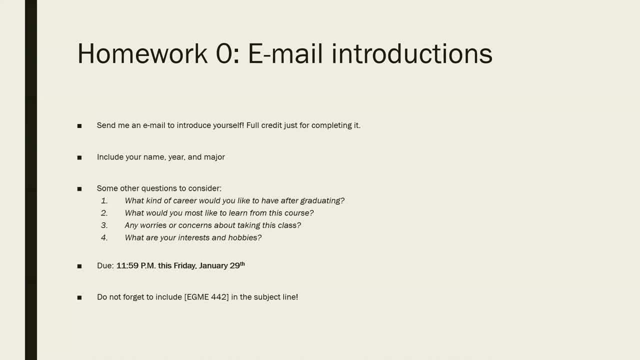 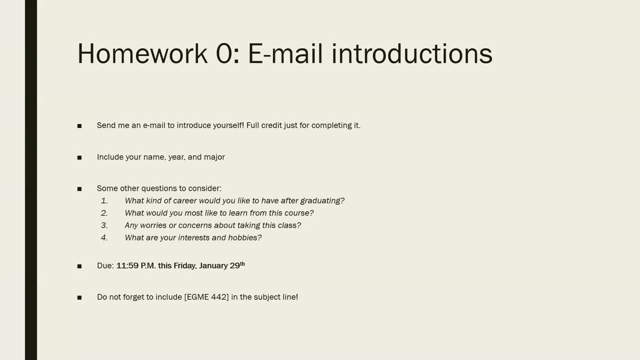 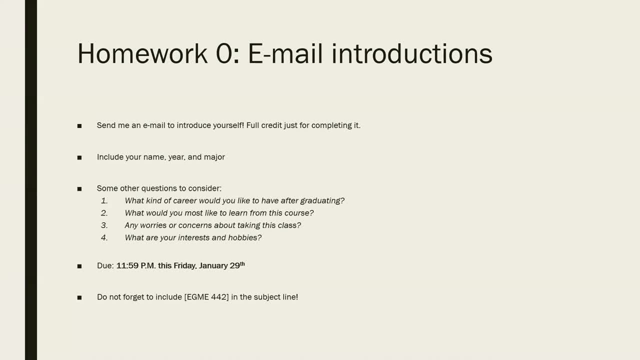 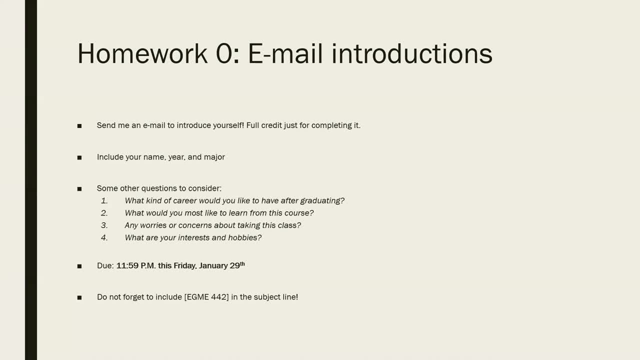 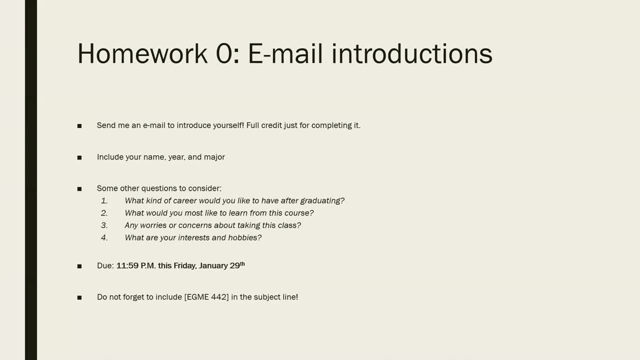 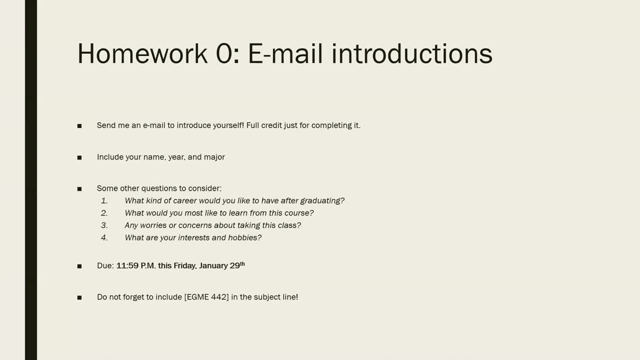 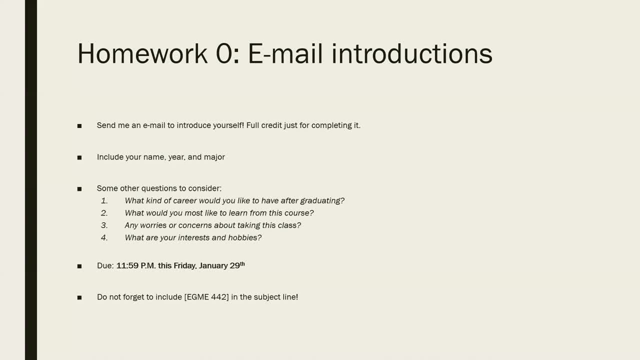 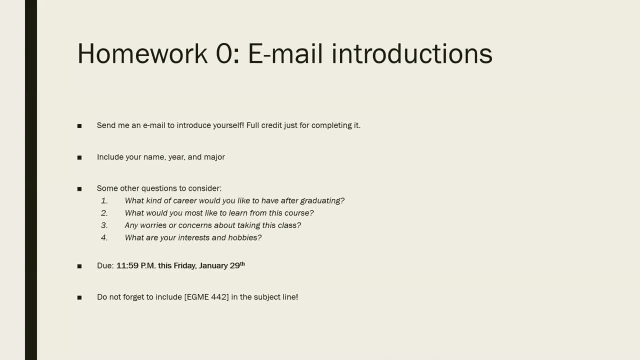 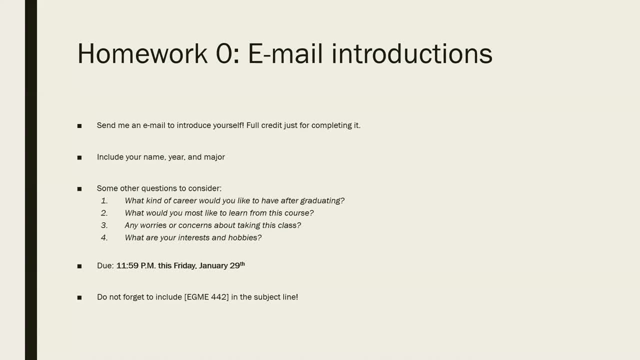 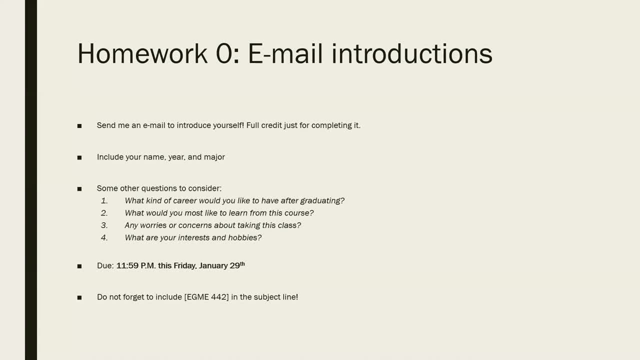 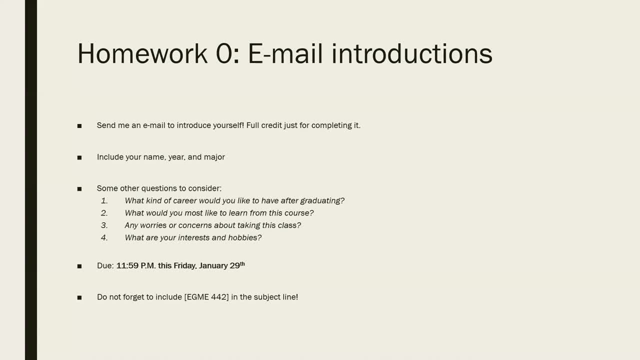 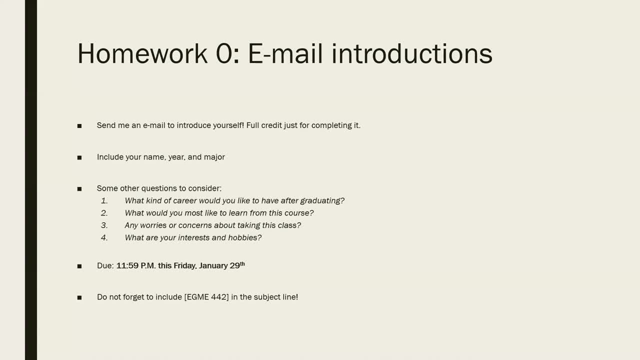 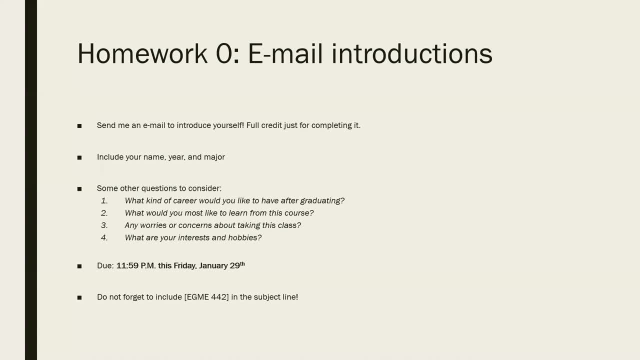 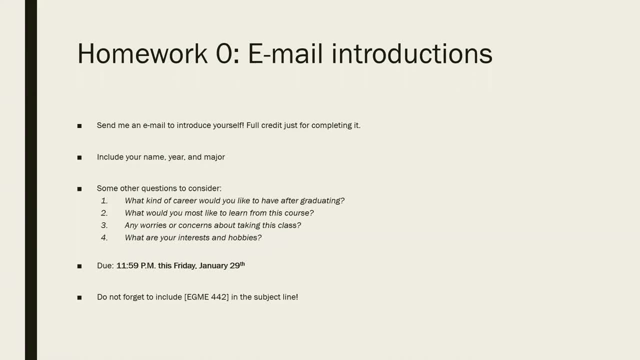 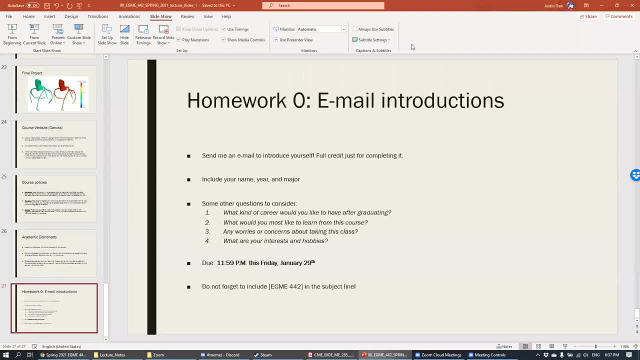 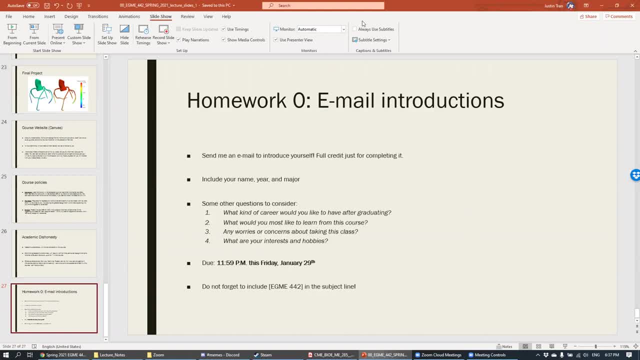 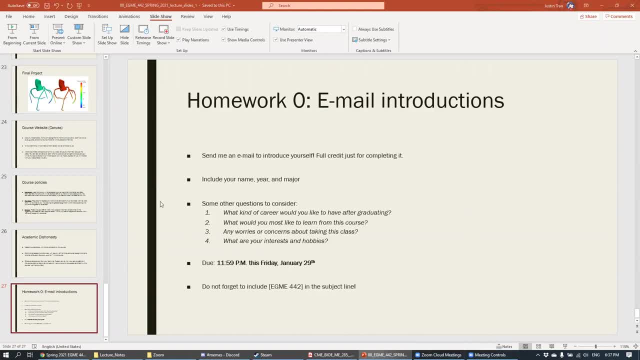 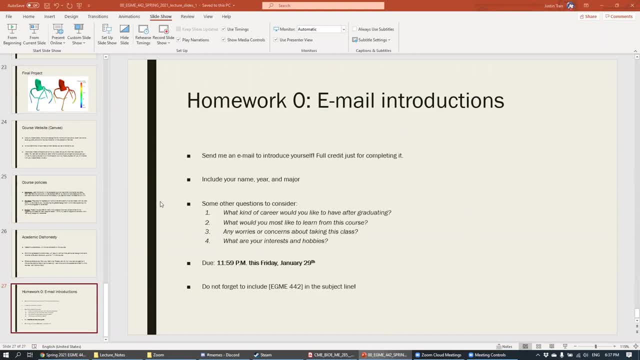 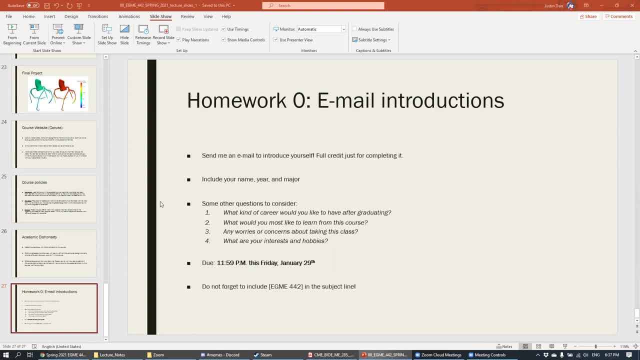 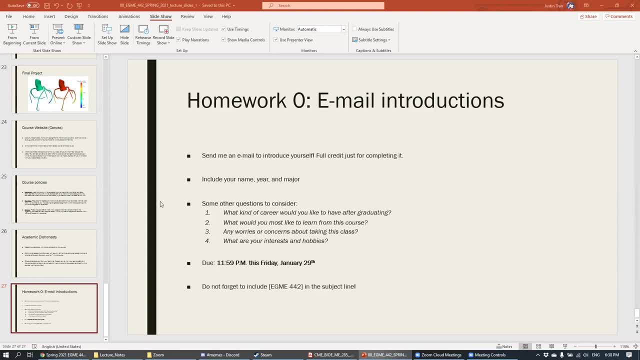 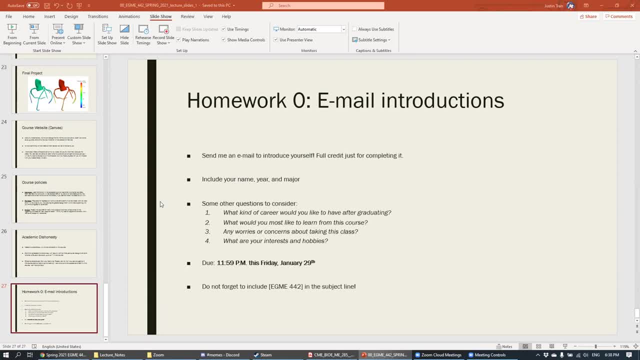 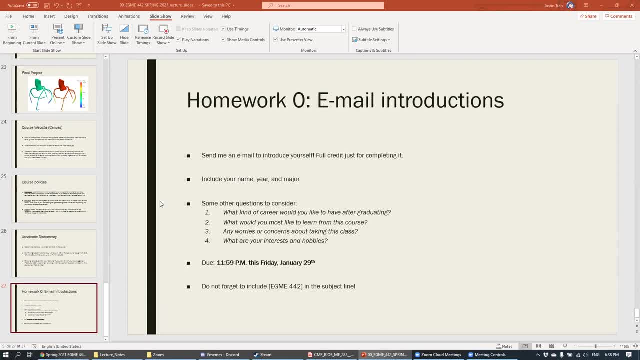 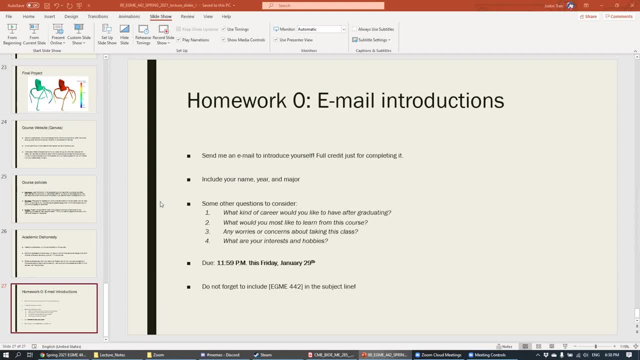 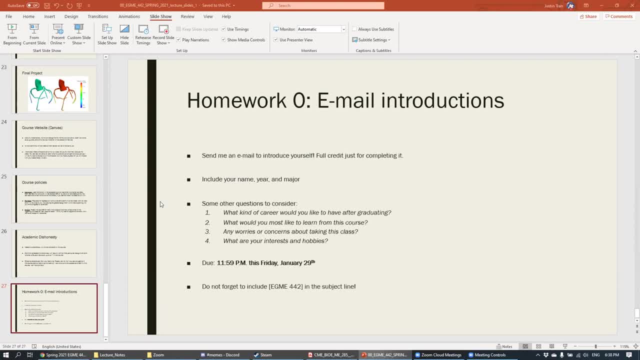 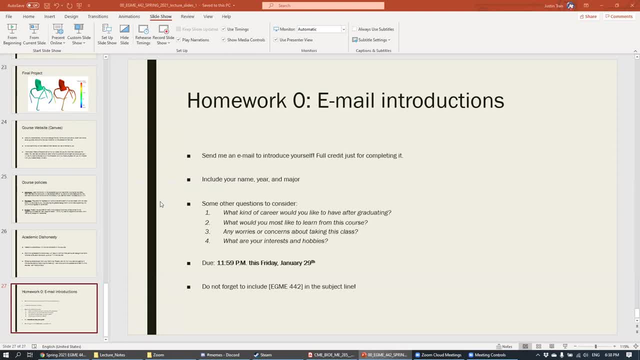 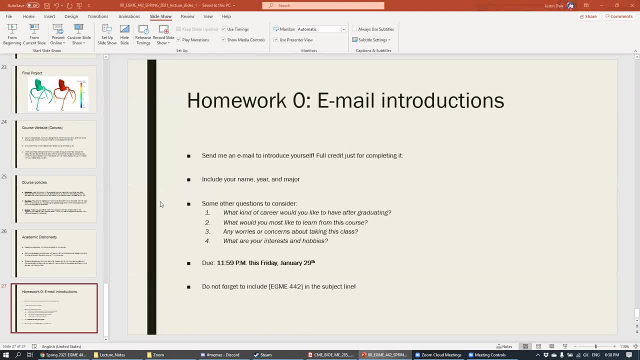 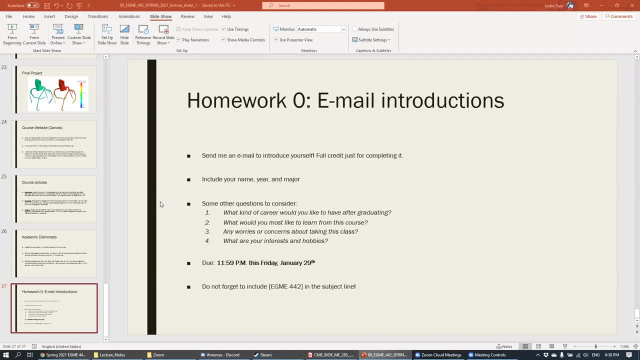 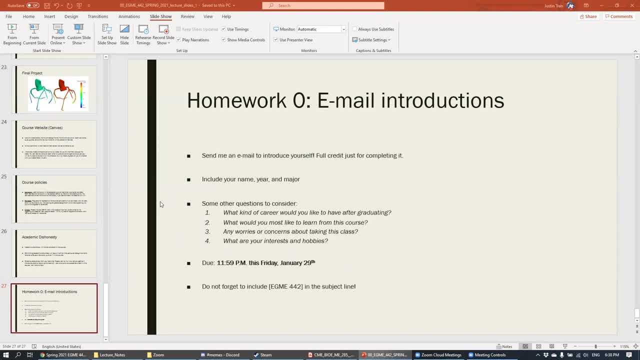 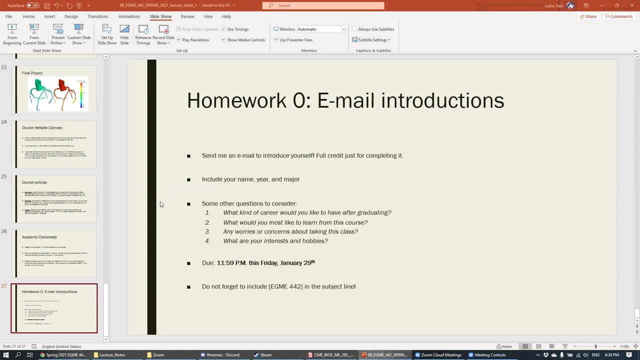 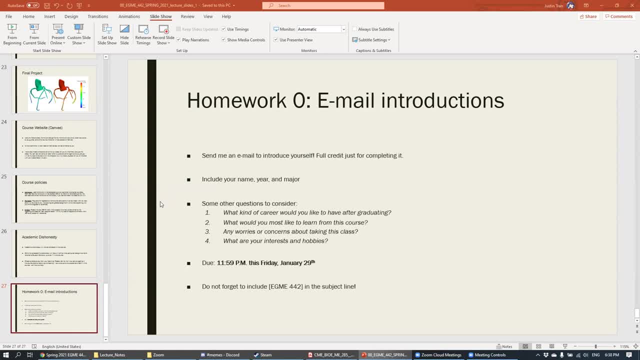 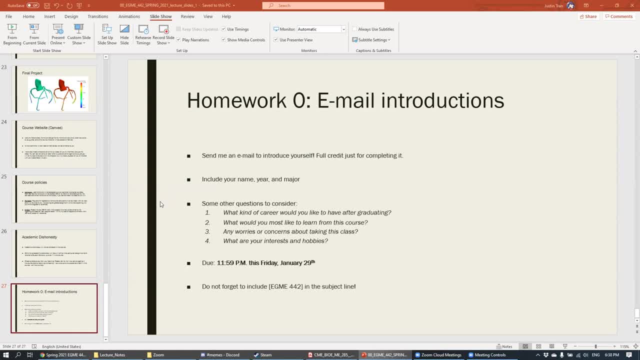 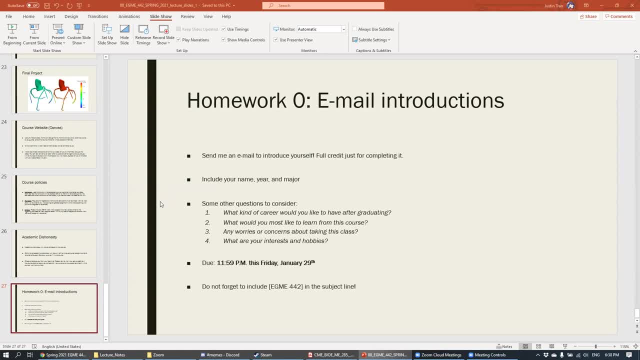 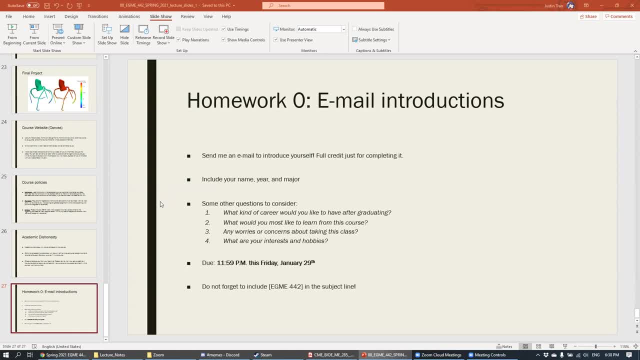 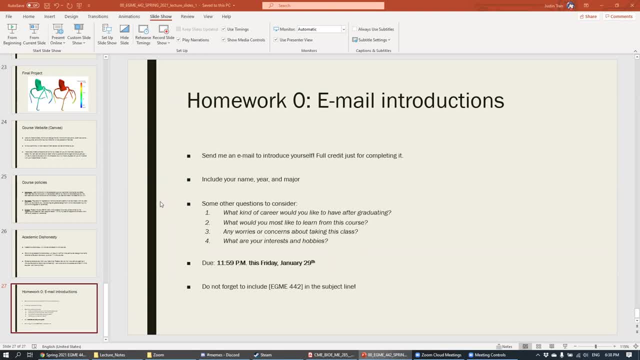 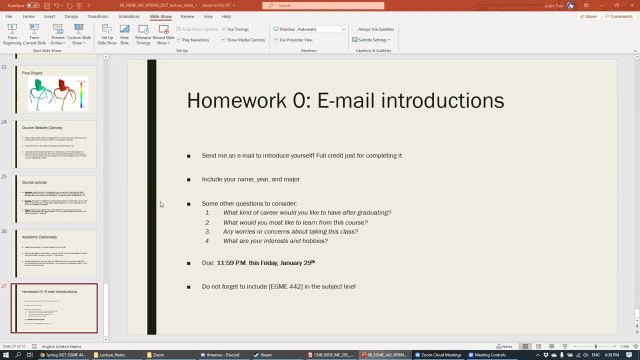 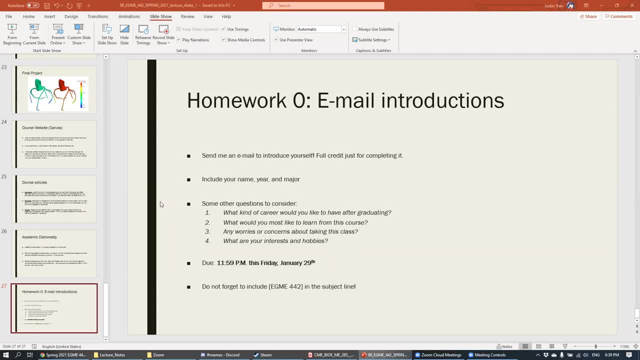 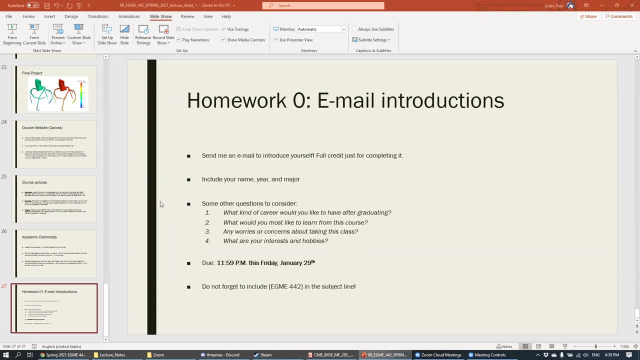 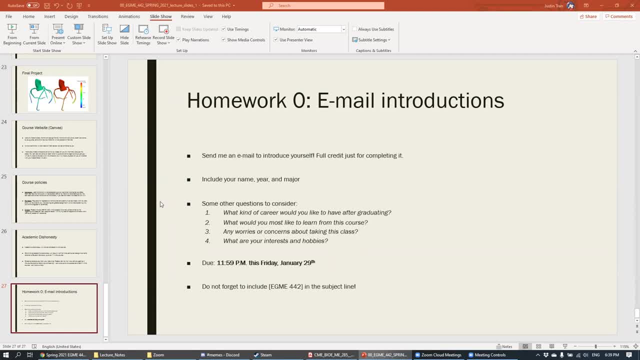 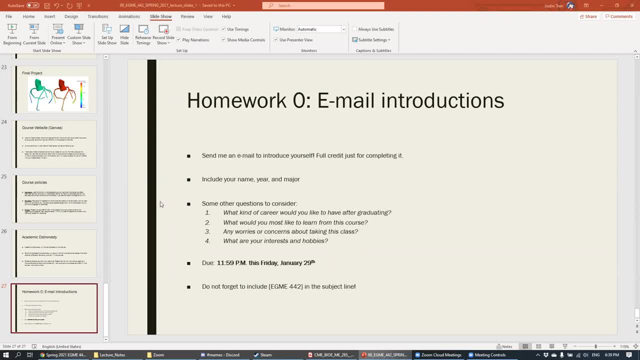 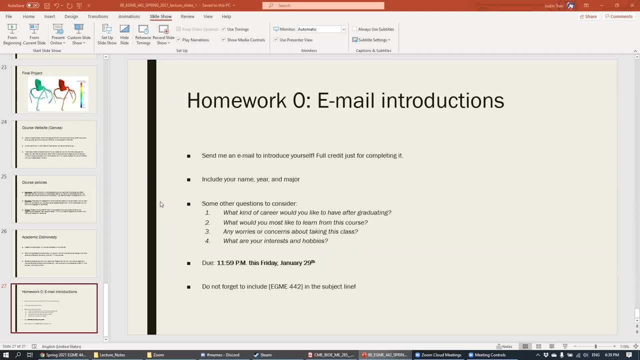 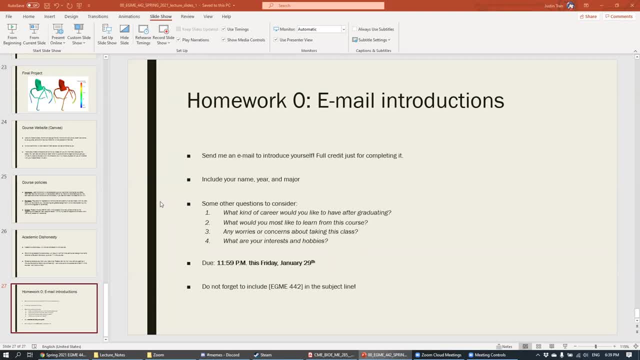 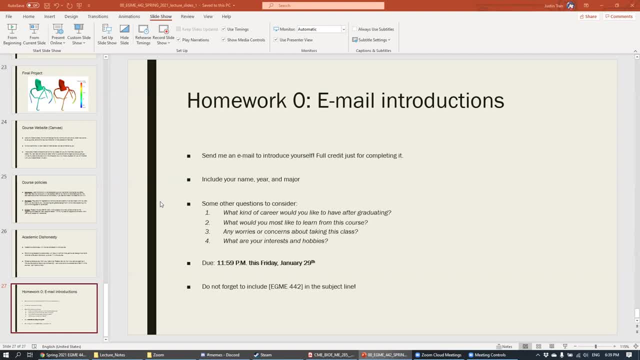 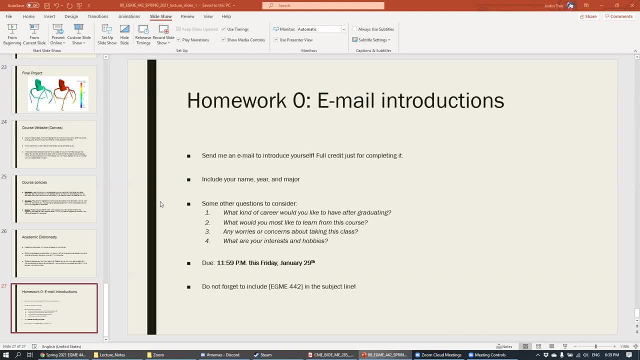 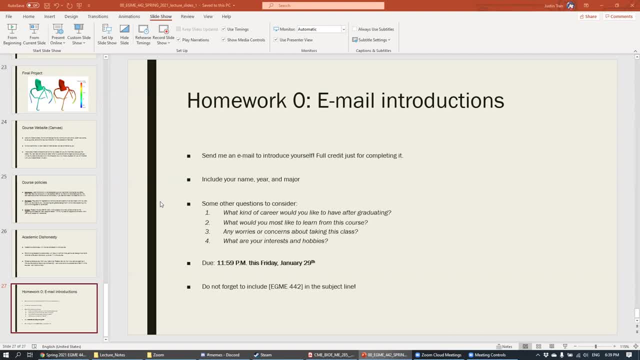 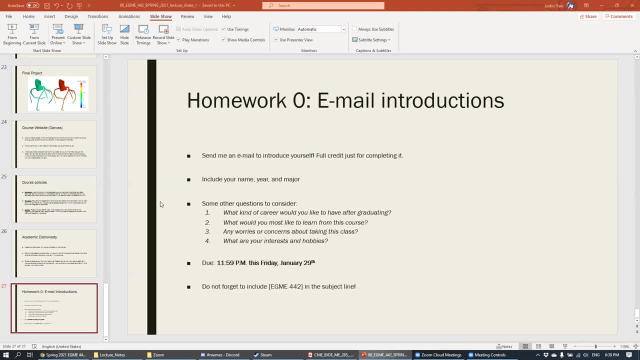 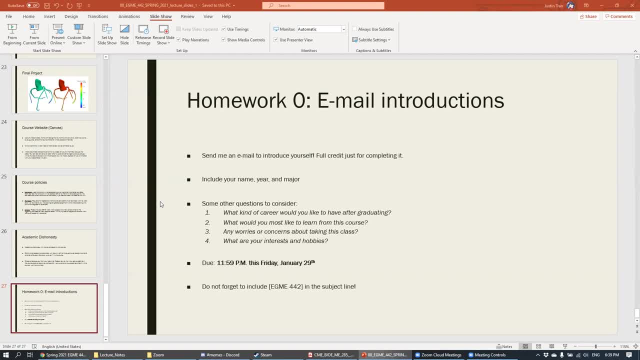 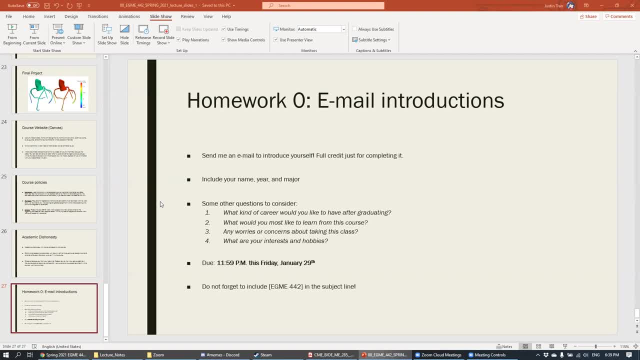 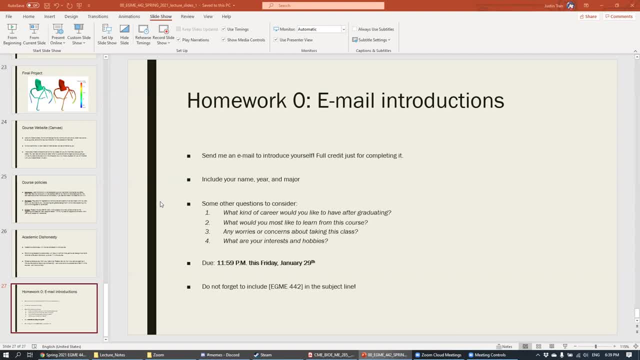 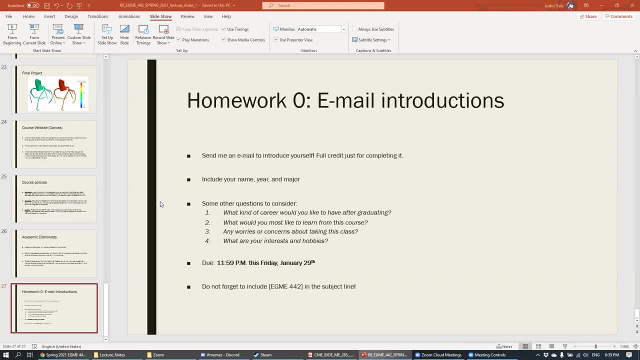 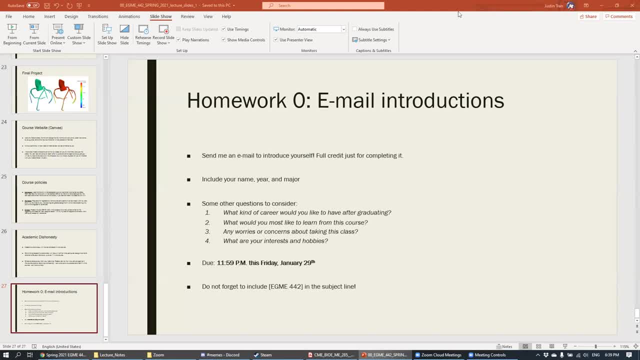 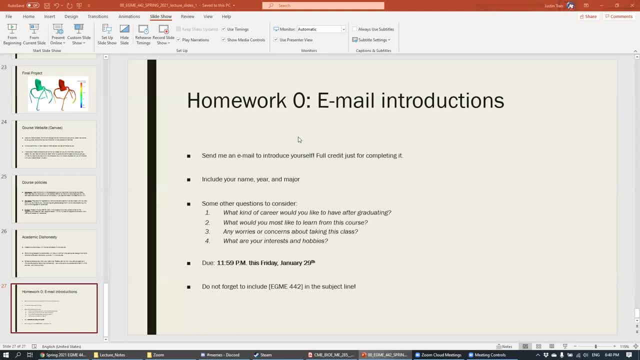 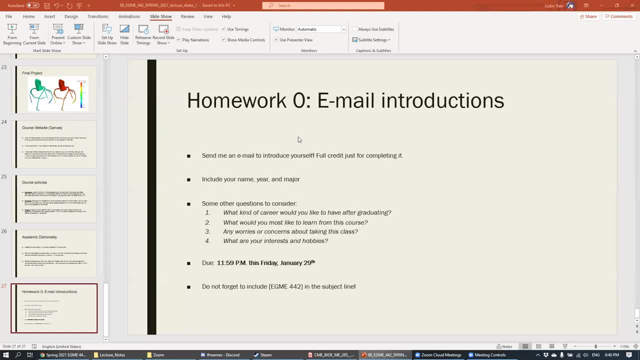 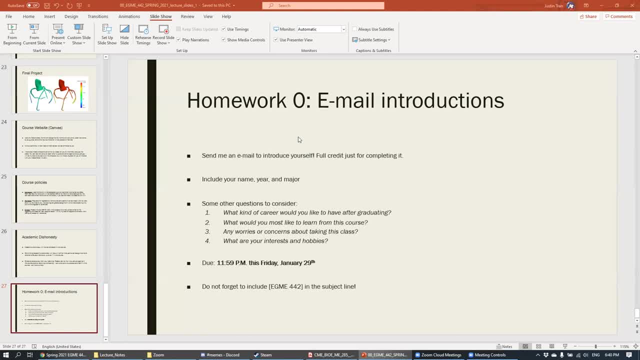 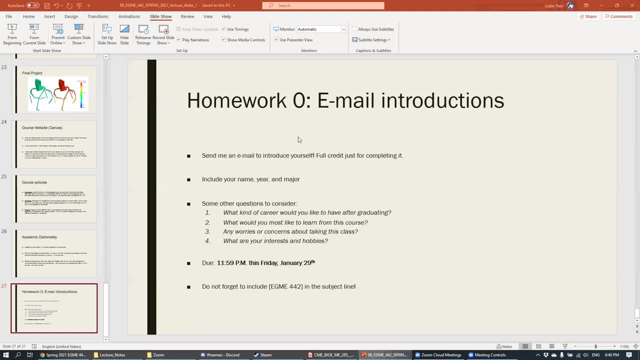 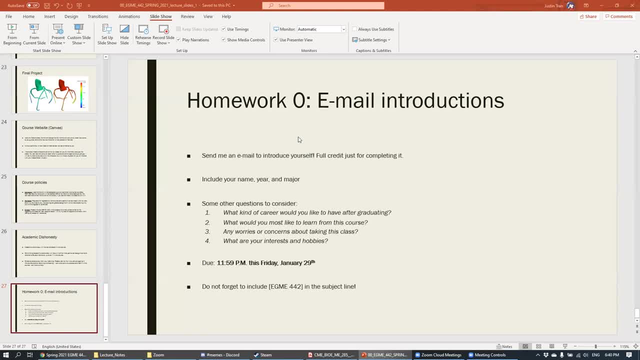 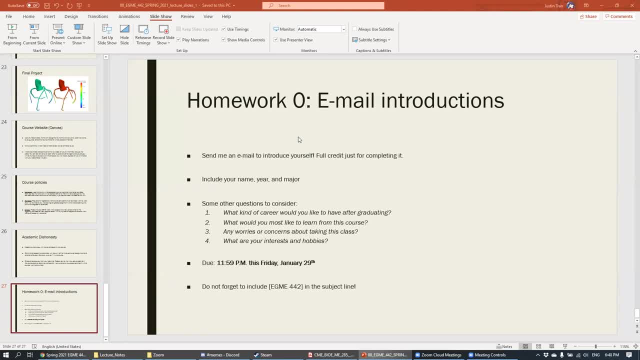 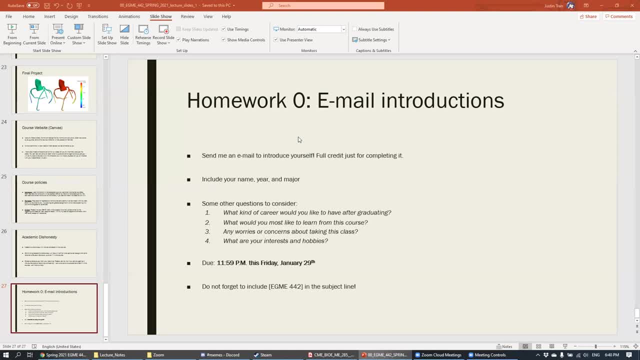 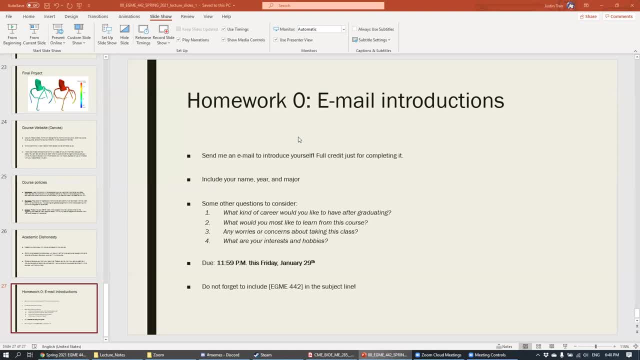 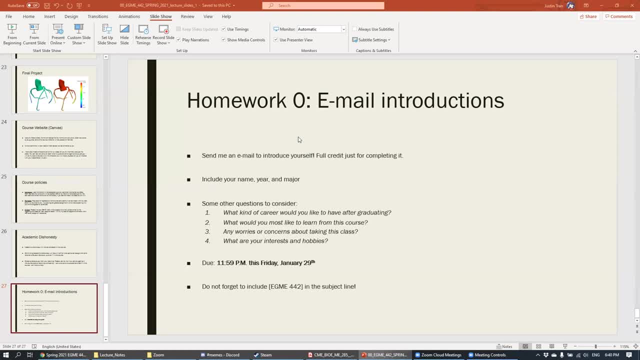 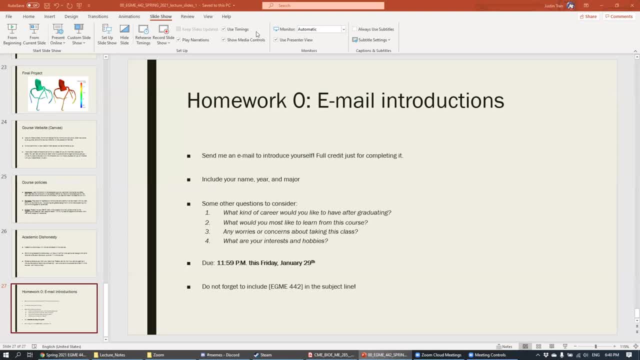 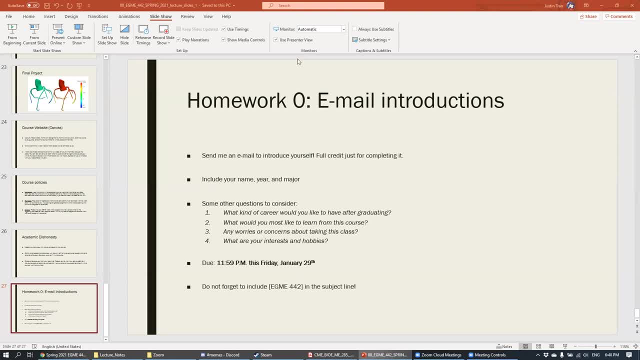 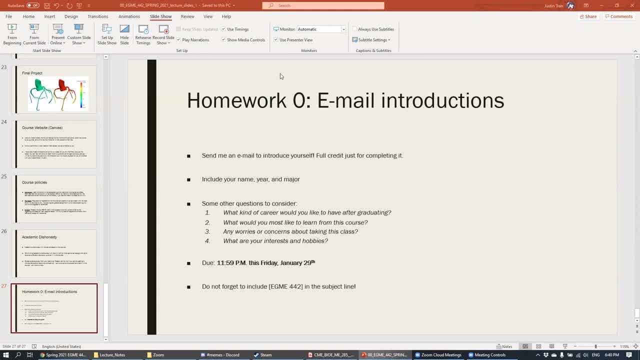 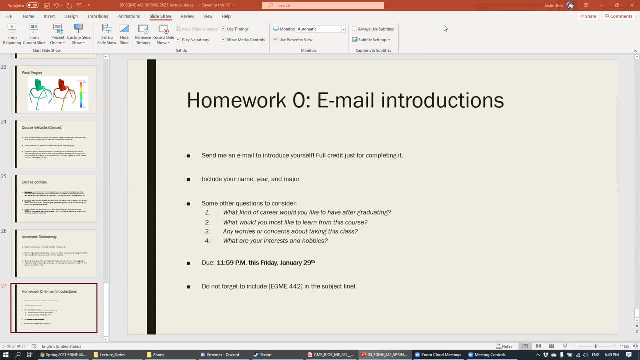 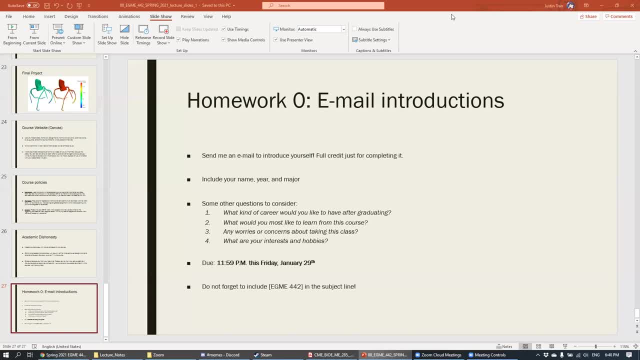 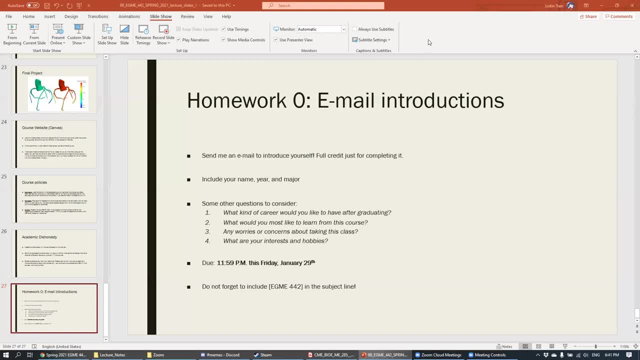 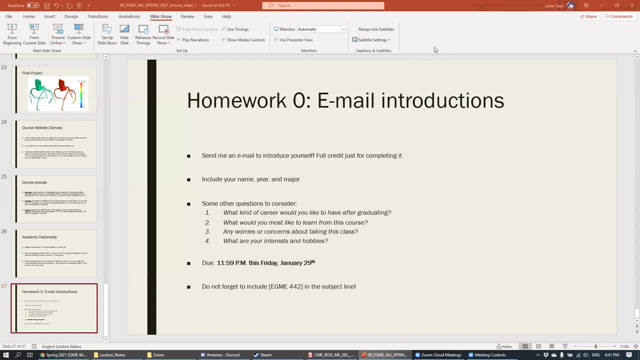 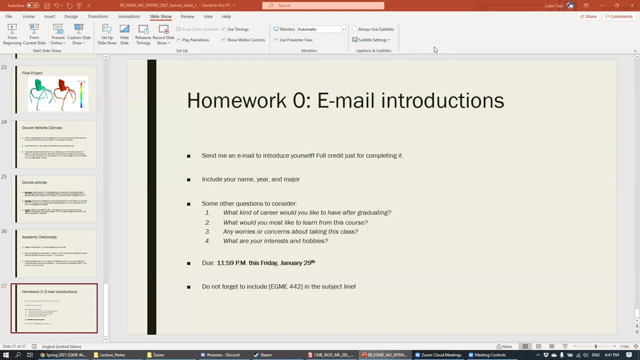 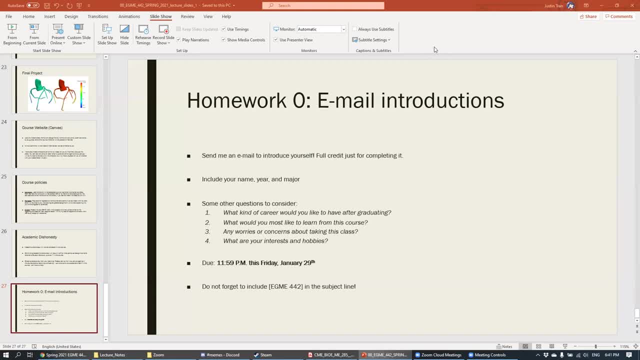 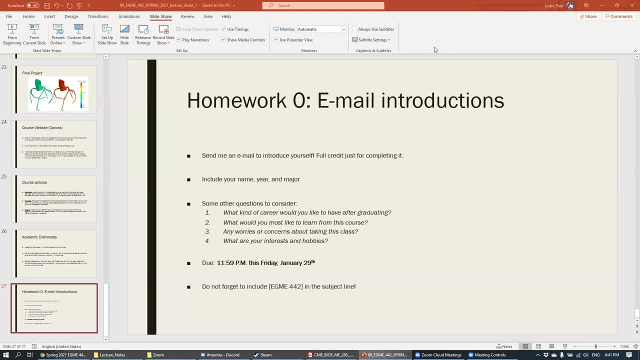 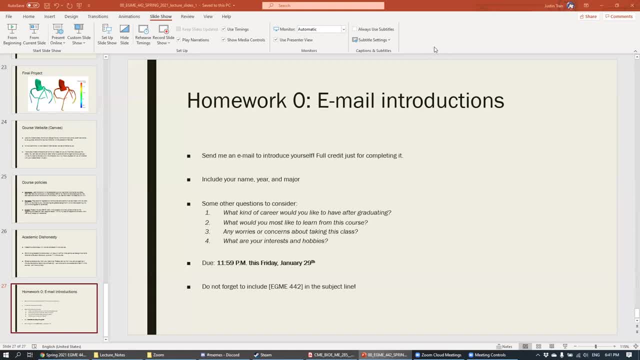 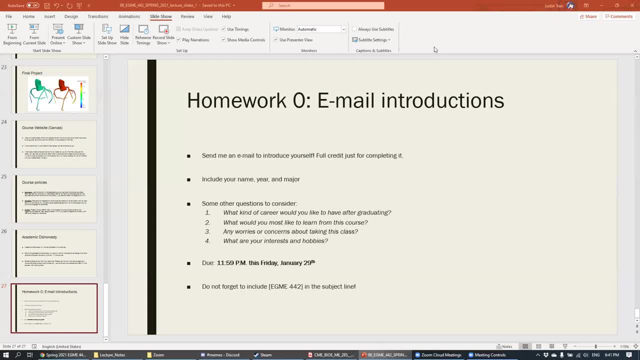 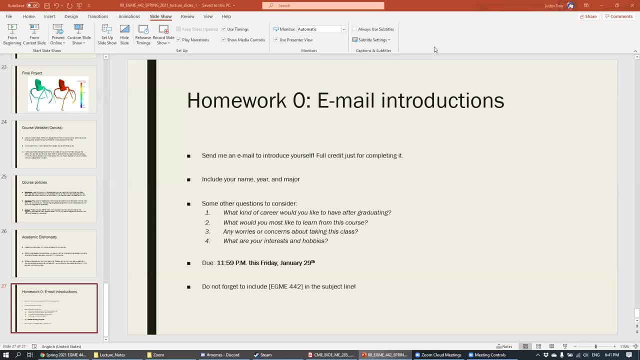 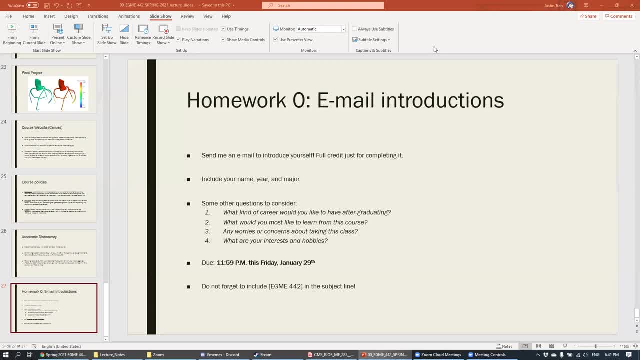 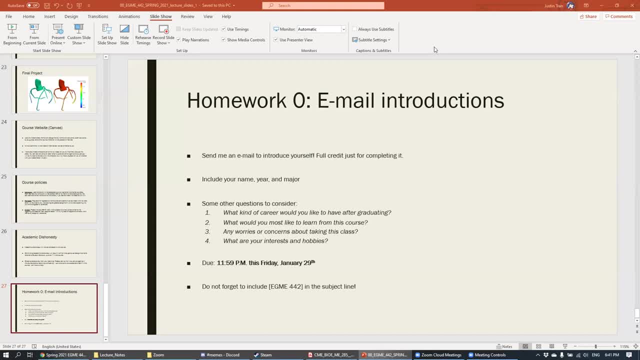 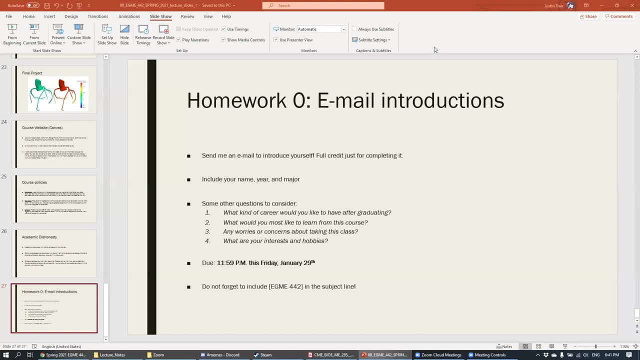 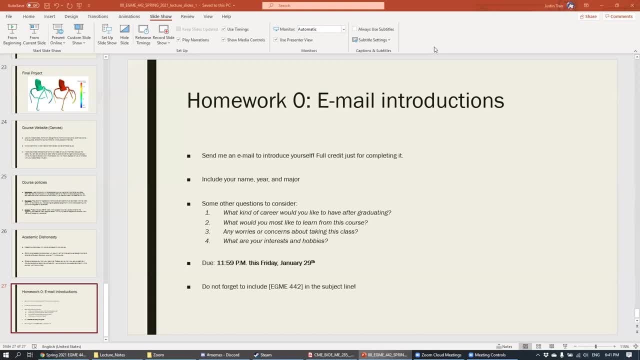 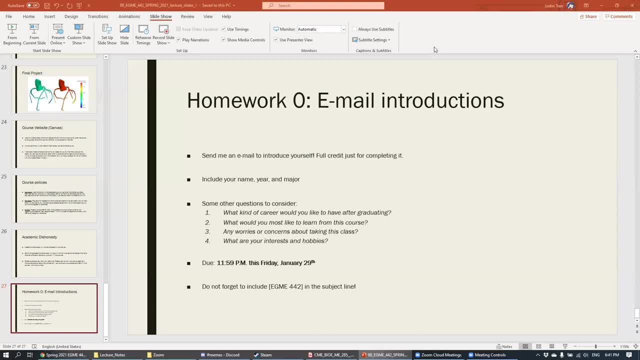 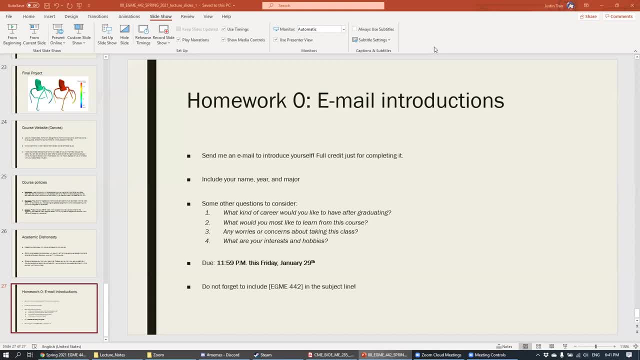 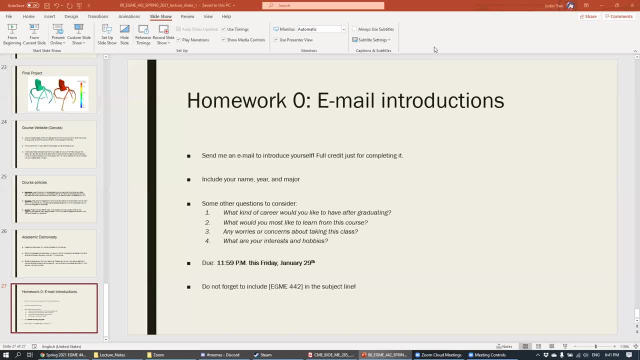 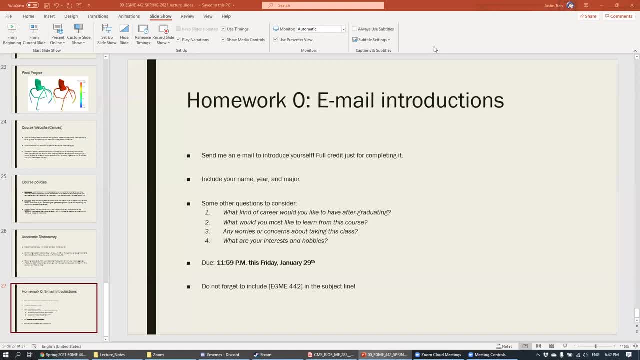 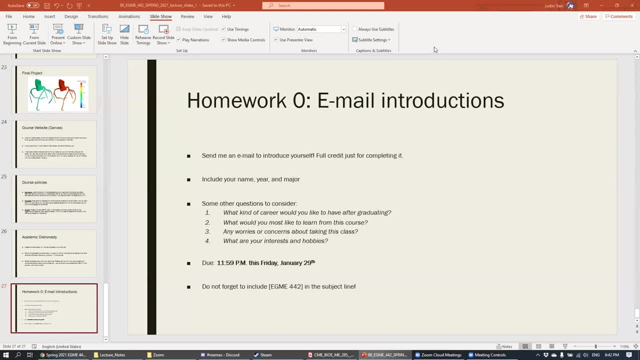 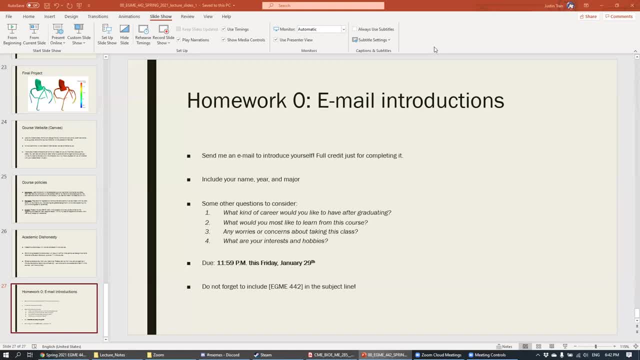 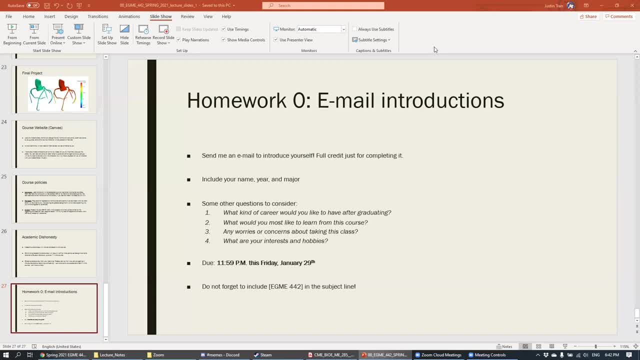 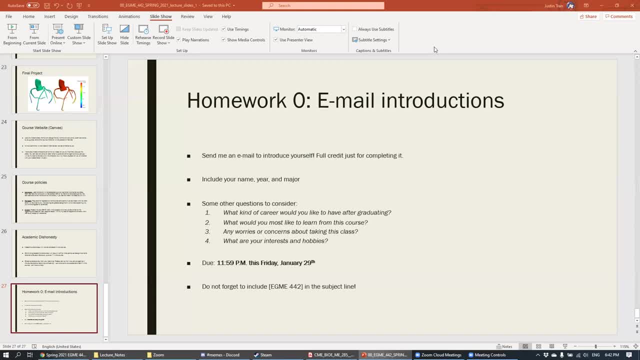 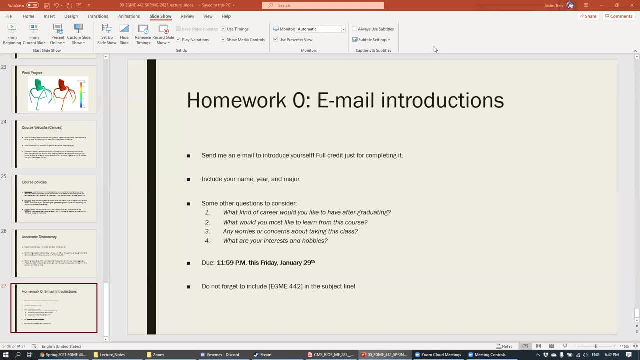 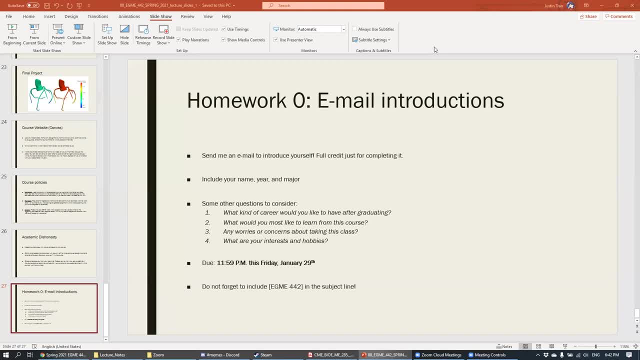 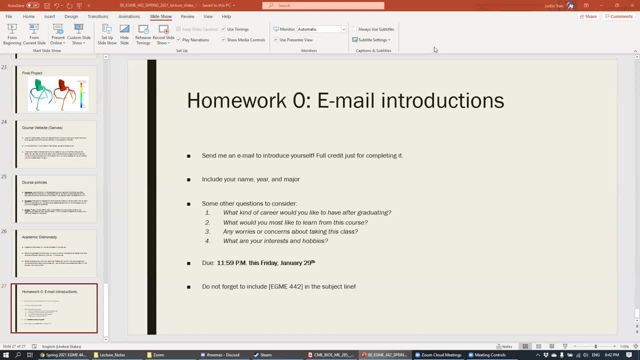 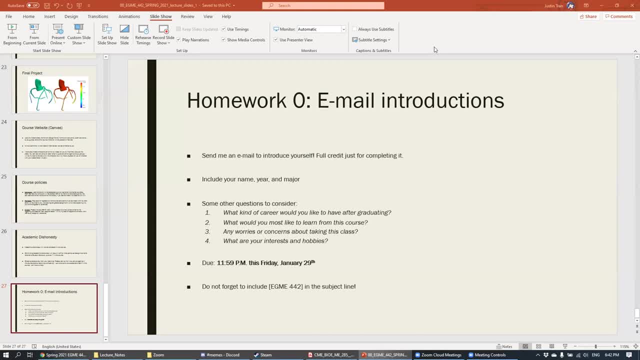 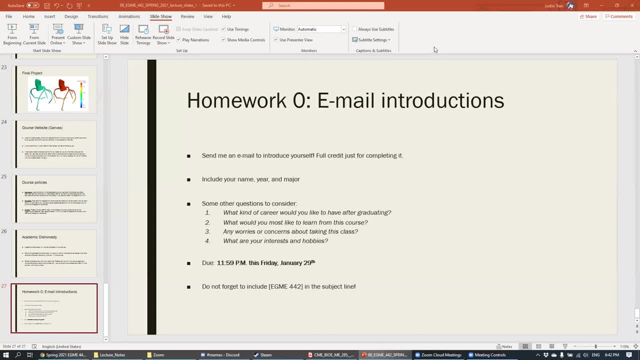 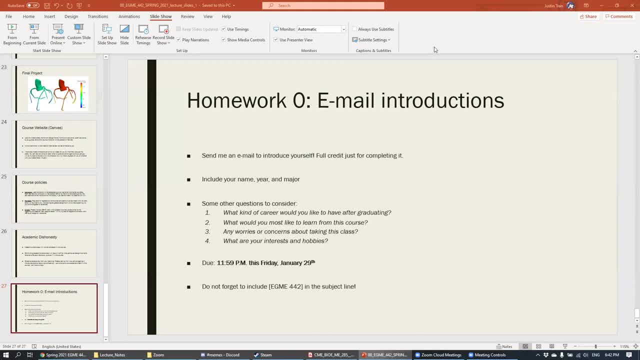 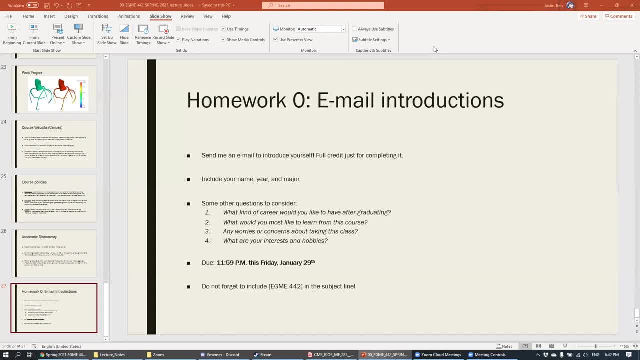 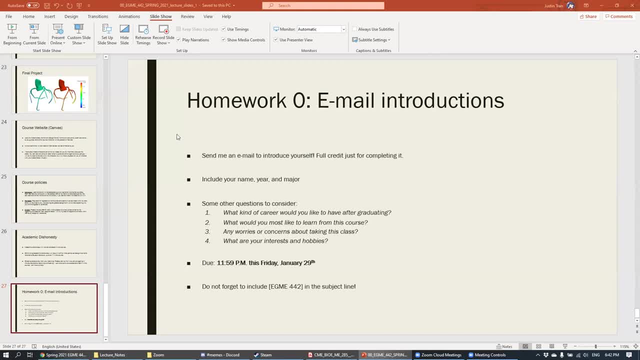 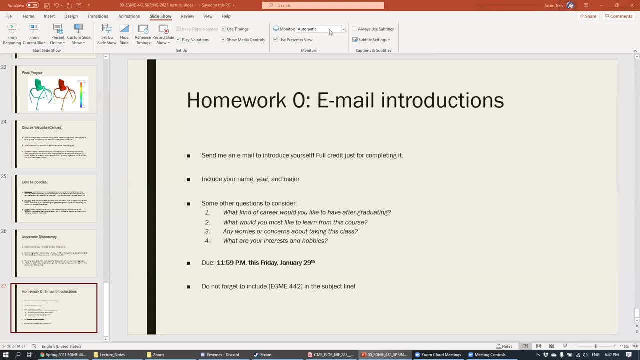 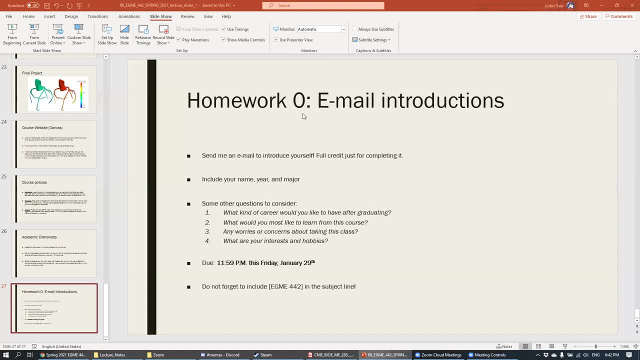 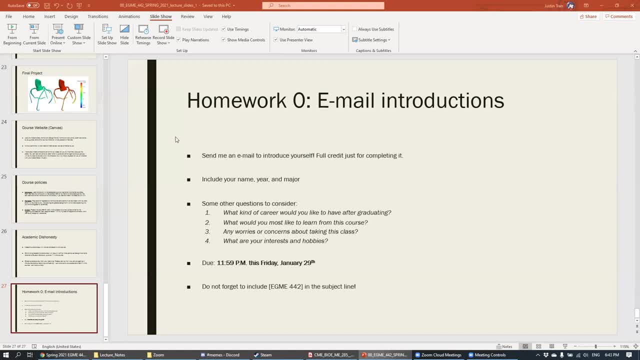 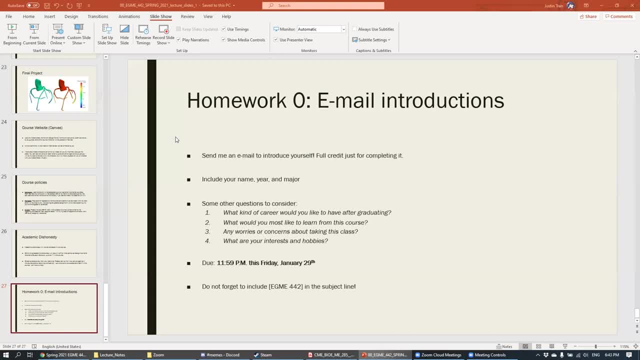 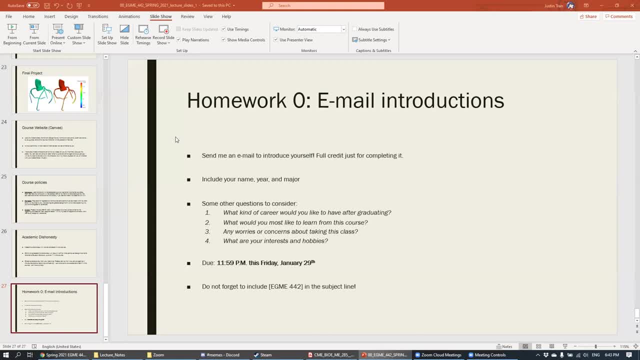 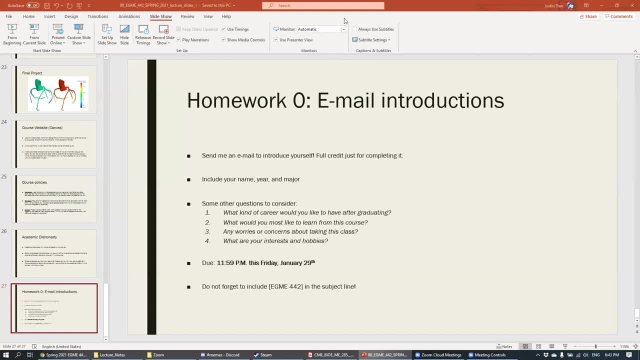